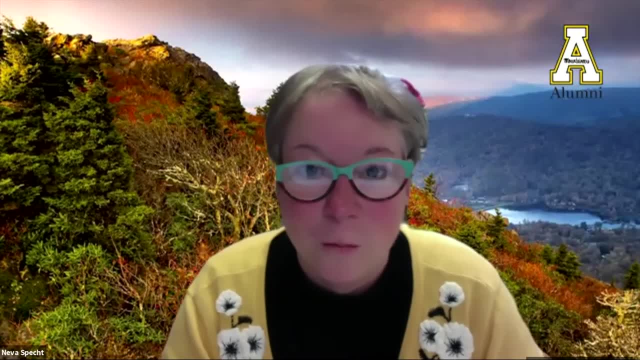 Carla to kind of pitch the video and then we'll share screen that and then we'll come back after that And I'm sure we can have a great discussion about everything's going on. So thanks, Carla, for doing this and I'll turn it over to you. Yeah, no problem. Thanks for the invitation. 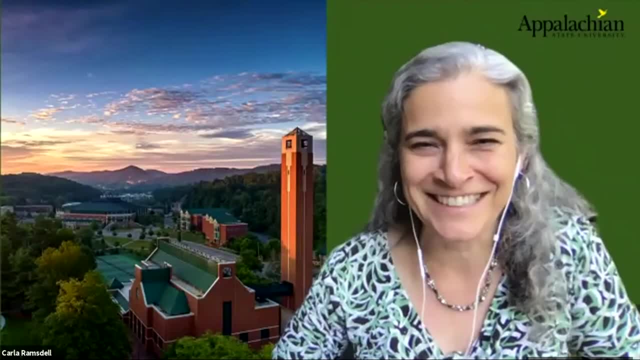 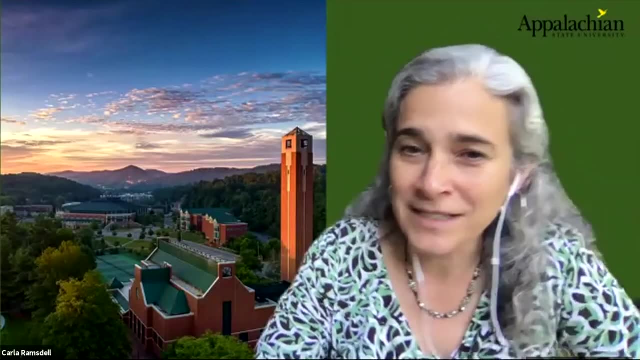 Thanks for being here. Good to have a fellow physicist on board, That's fun. So, because of the timing of this, I just went ahead and did the solar cooking demo separately and recorded it, And so I think we're just going to go there and 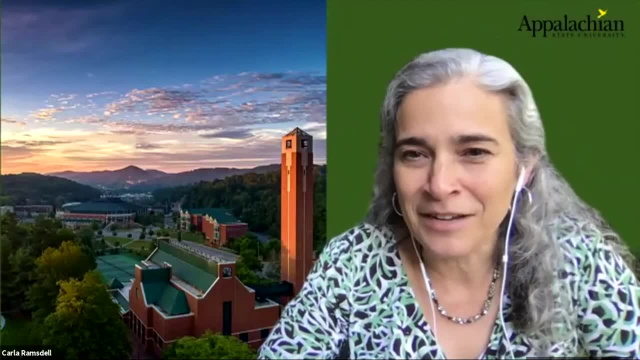 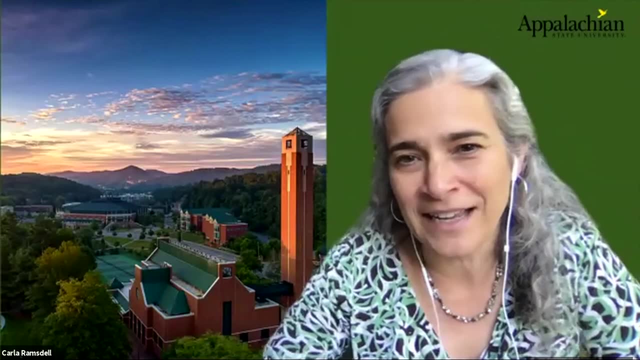 watch that. It was a really pretty day. We had a little bit of cloud cover come in. for the most part We had some pretty optimal cooking conditions. So I think we'll just watch that and then do Q&A afterwards. So if you have any questions, as we're going through it, if you just want to, 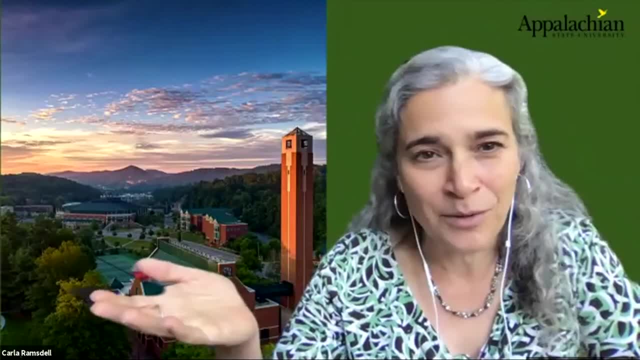 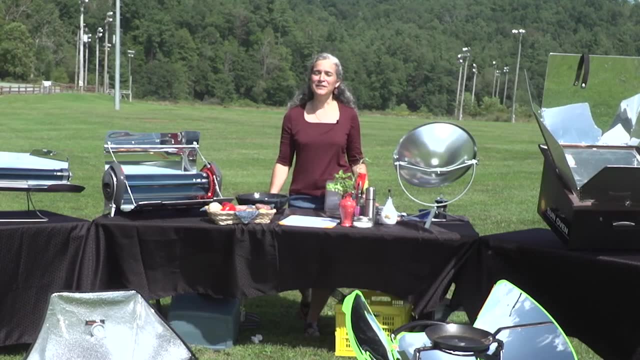 jot them down. that'd be great. Just so you know this is being recorded. Hi, my name is Carla Ramsdell and I teach in the Department of Physics and Astronomy here at Appalachian State University. I am here in the middle of Boone. 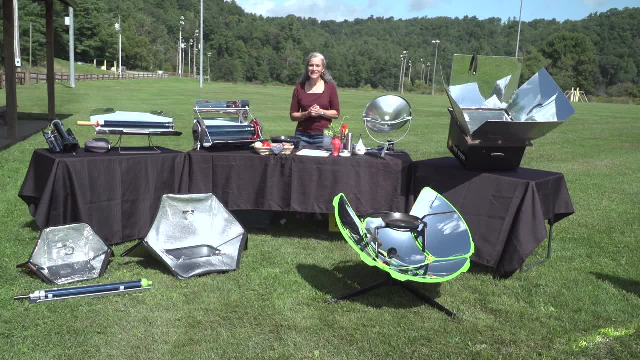 in this beautiful September day in the Appalachian Mountains And I'm going to do a little demonstration about solar cooking. First a little bit of background about myself. I came into higher education as a second career. I am a registered professional mechanical engineer and I worked in. 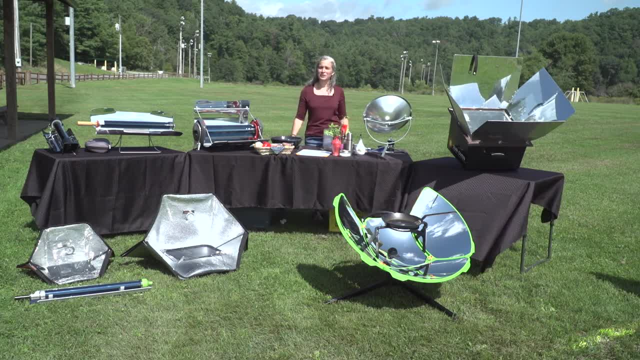 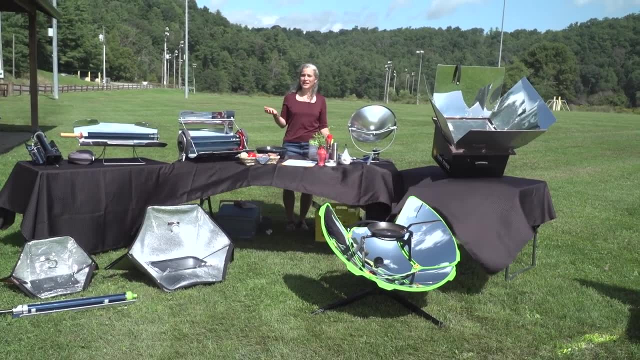 the electricity power generation sector for a long period of time and then came into higher education, So it seemed natural that I would just start teaching. So I'm going to show you a little bit of what I learned about energy and about energy, which is what I did. So I teach courses on energy. 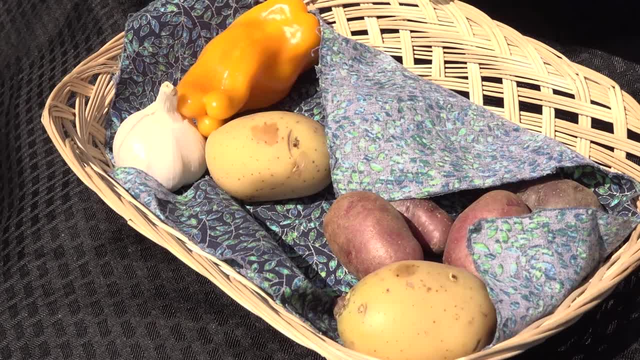 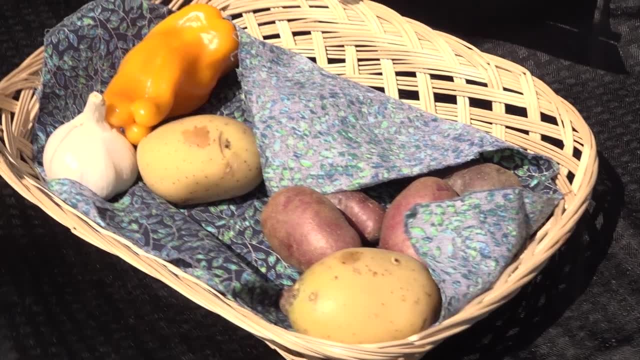 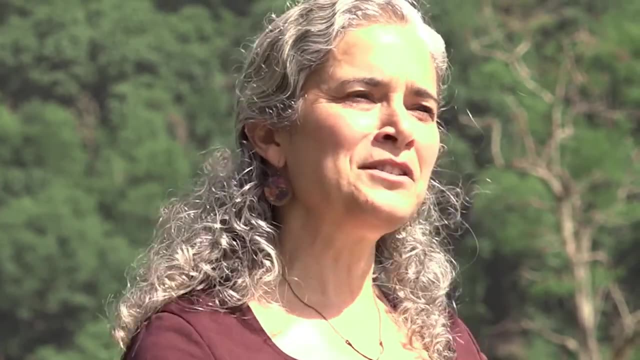 and sustainability. But I noticed that I'm Italian And so food is a huge part of who I am and my upbringing, And I recognized that when I interjected comments about food into my classroom, for example, talking about specific heat, and I see this sea of students somewhat engaged in that I mentioned. 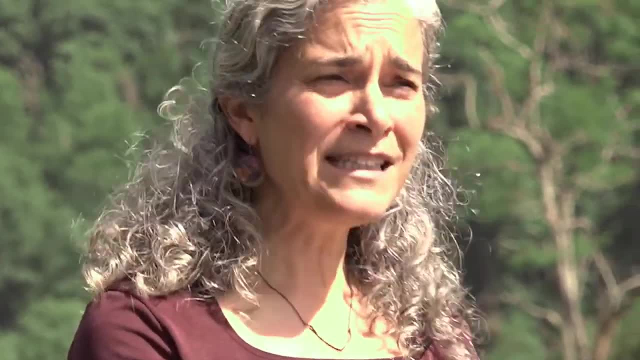 well, that's why we use a stone and that's why a pizza cooked on a stone comes out so much crispier all of a sudden. I would recognize that. I know we had some people. I wanted torock conceptualanias. you know we couldn't keep it fresh in class. you know we hadn't used that much energy, So I was able to legs and donald 줄 dangerous with mainstays, м seinem. 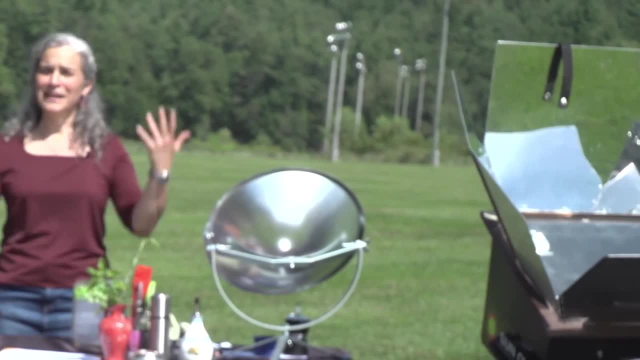 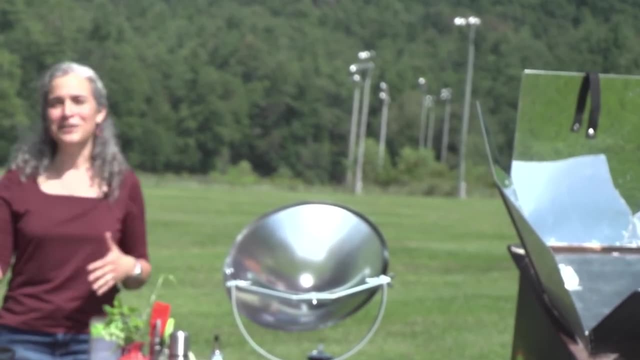 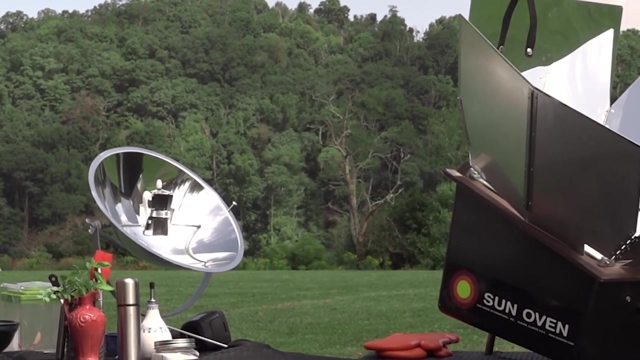 that all of my students immediately are looking at me and engaged and asking their neighbors: wait, what did she just say? I think that was important, and so I recognize that introducing food into physics and into this discussion about sustainability was a fantastic way to engage people. as I started doing more. 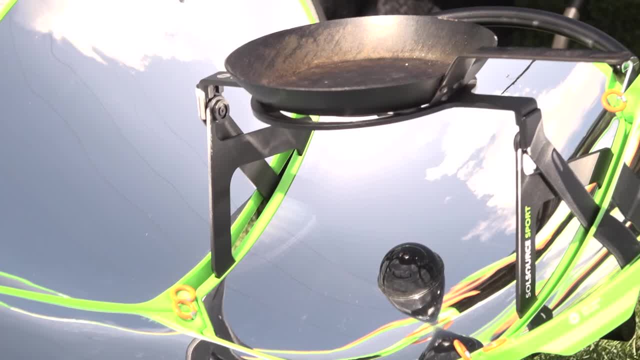 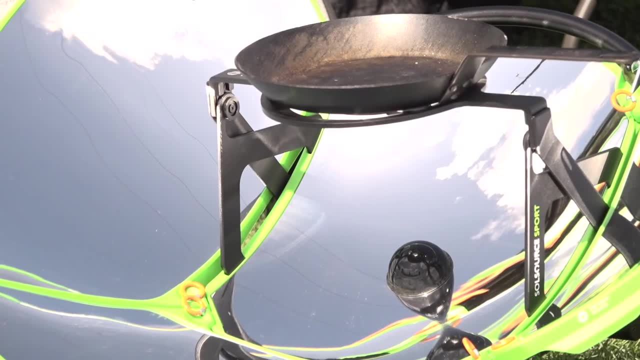 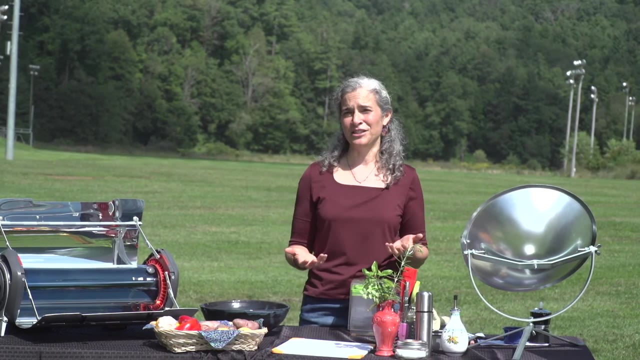 research about physics and food. I recognize that this is an energy source that I believe is underrepresented in our energy efficient discussions. food is energy and how we, how we manipulate it is really important and is one of the big drivers in climate change currently. so now my work is all about the physics. 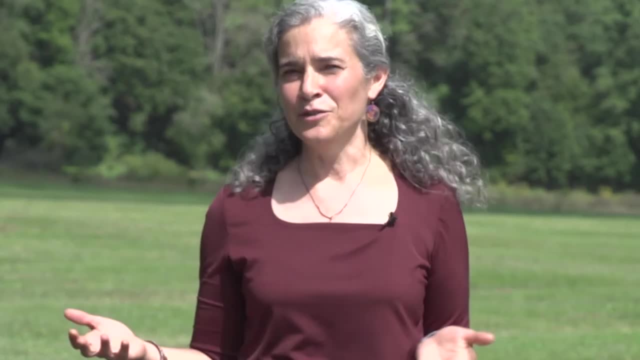 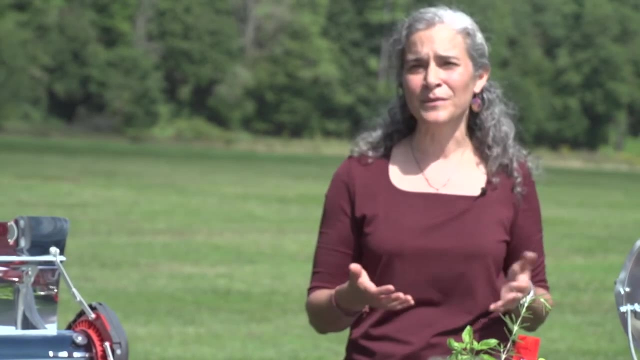 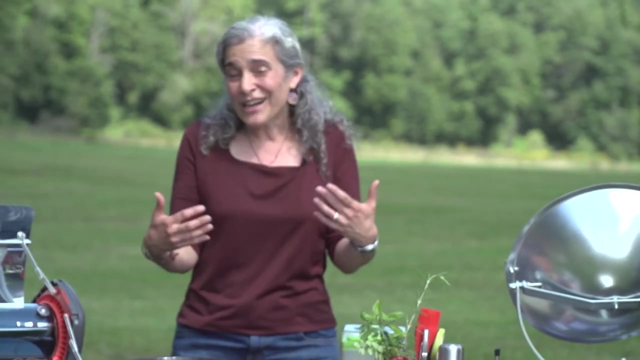 of food and the thermodynamics, studying the energy of the food system- and I take a really broad, broad look at it- from what foods we choose to grow, and then how we process them, how we package them, which is a big deal, and then how we transport them and refrigerate or freeze them. and then the fun part happens when 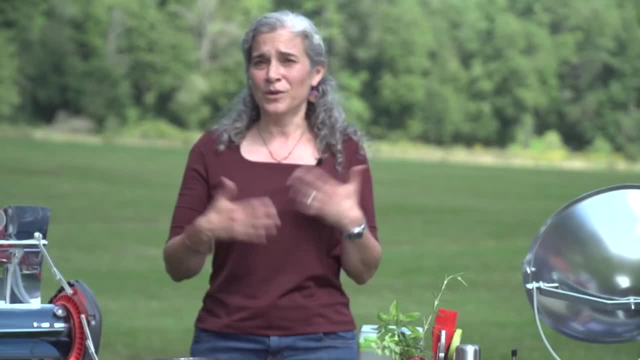 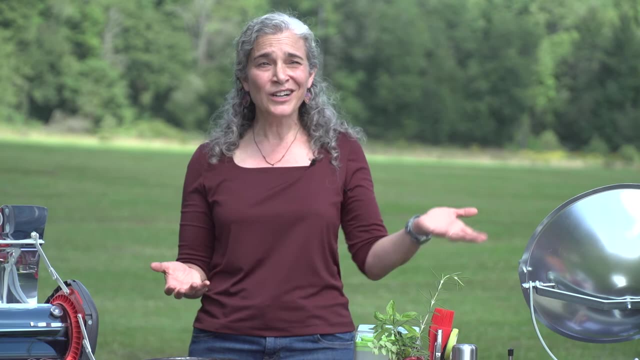 it gets into our home. so how we, how we cook it, what skillets we use. for example, my latest research project studied eight different skillet materials, from a $200 solid copper pan to a humble $15 cast-iron skillet, and we used infrared thermography to try to. 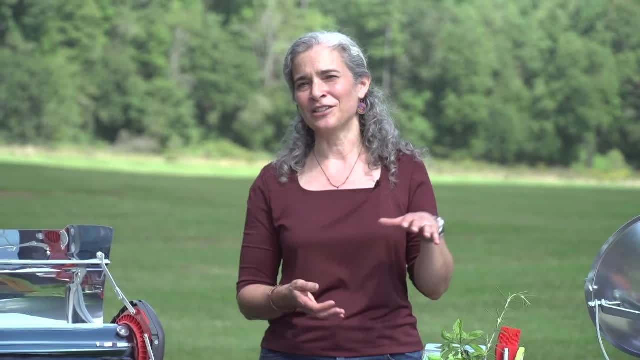 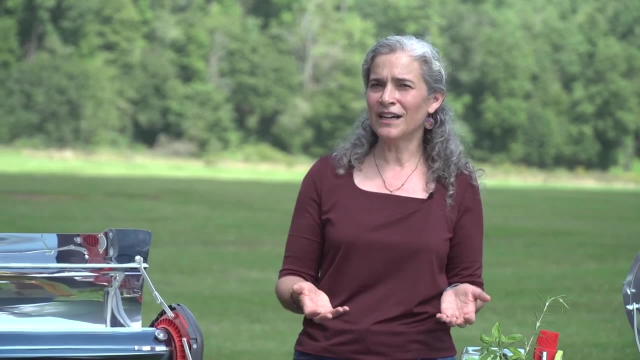 dictate what is the most sustainable skillet, both based on thermal properties and some non thermal properties. so so yeah, we cook in our home, we look at different types of ovens and talk about refrigeration, and then the final step of my work is looking at the disposal side of things and how we're 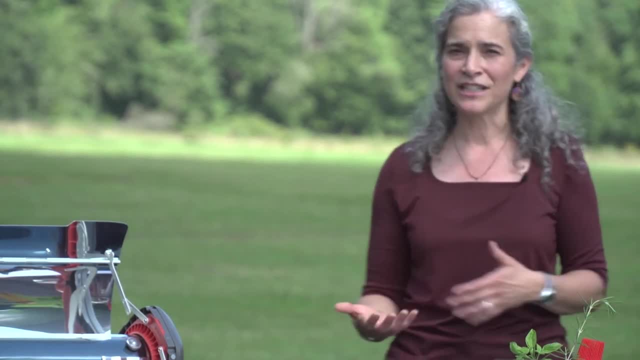 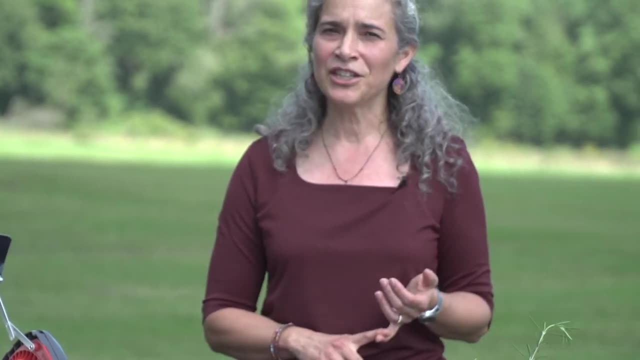 responsibly getting rid of things and recycling the packaging and what have you so? so that's the broad search. I teach courses. I teach a first-year seminar class on the physics of energy efficient cooking. I teach the general physics series, which I introduce some food into. I teach this course on energy. 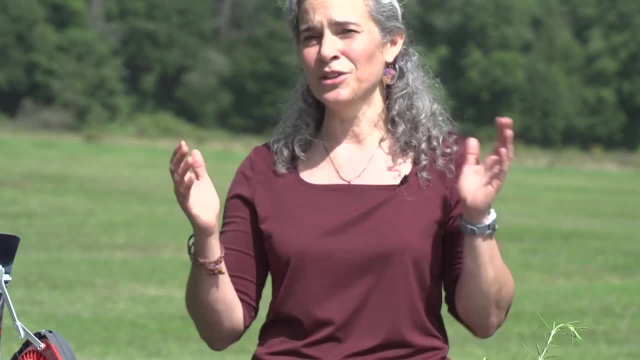 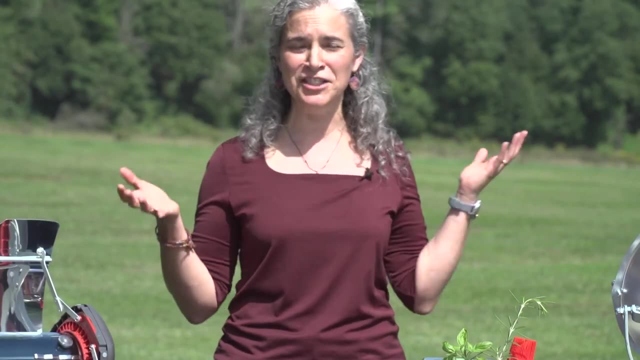 and sustainability, and then also I teach a course dedicated to the physics of food and cooking. so, as we said, we're gonna- we're gonna talk specifically about how to cook with the Sun Right. so when we're in our, in our kitchens, we can talk about efficient ovens, but still they have 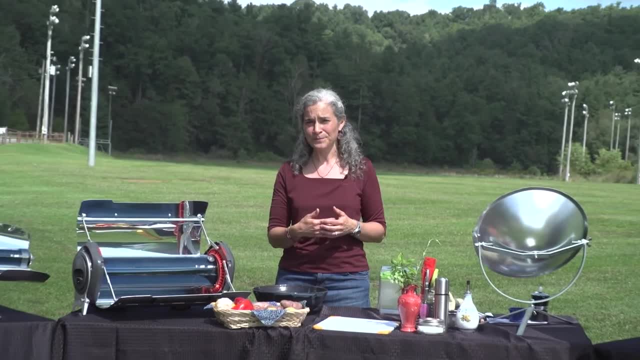 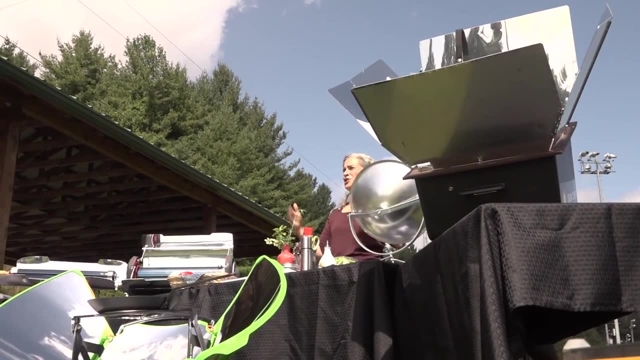 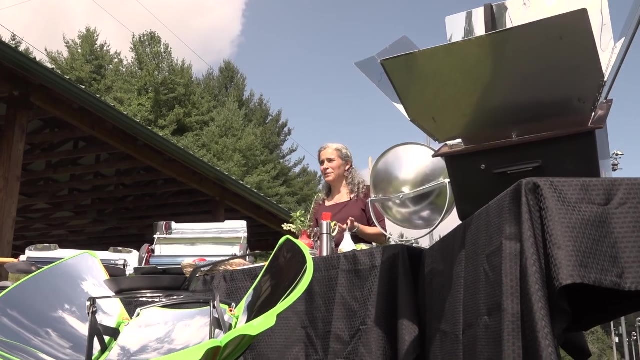 either fuel or electricity coming into them somehow On a beautiful day like today, we have about a thousand watts of solar energy incident upon the earth every square meter, and that's a pretty significant amount of energy. so a lot of people obviously are engaged in this topic of how. 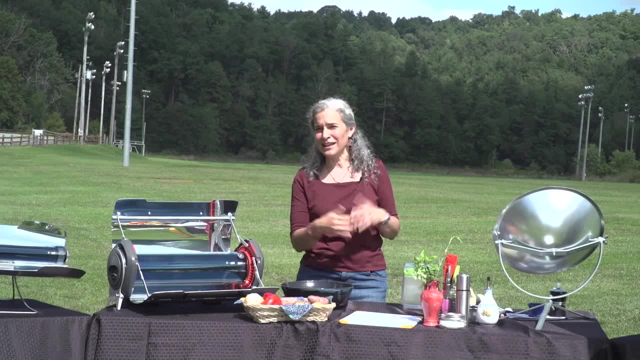 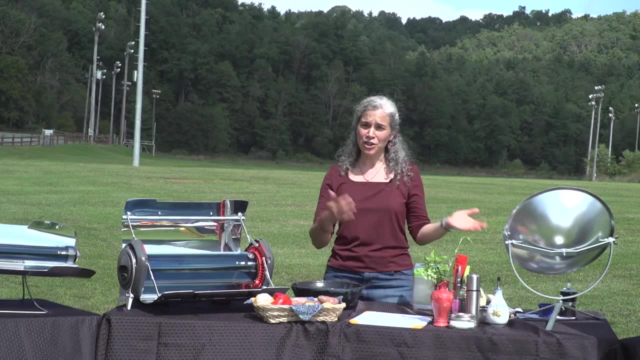 can we use that to cook for us, and so there's a lot of really creative solutions that we'll talk about and we'll get into the physics, but before that point I thought maybe it was a good idea to go ahead and just start cooking so that the food can cook while we're describing the physics. 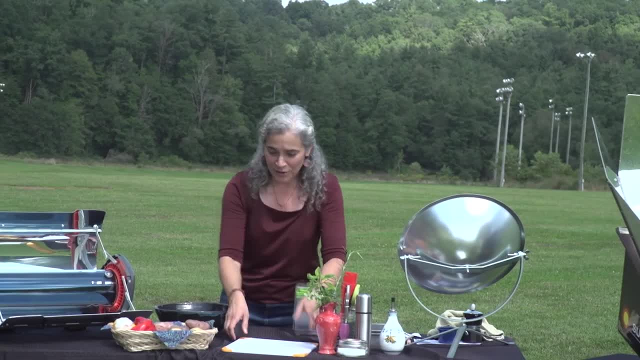 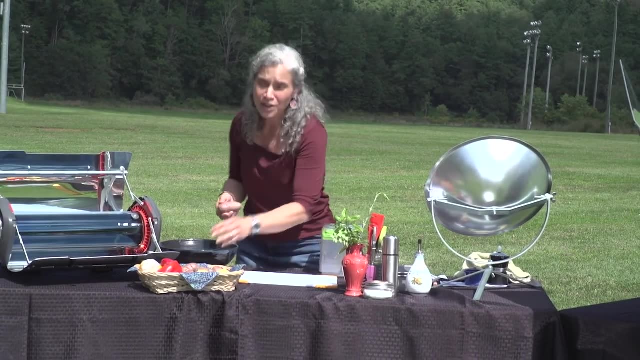 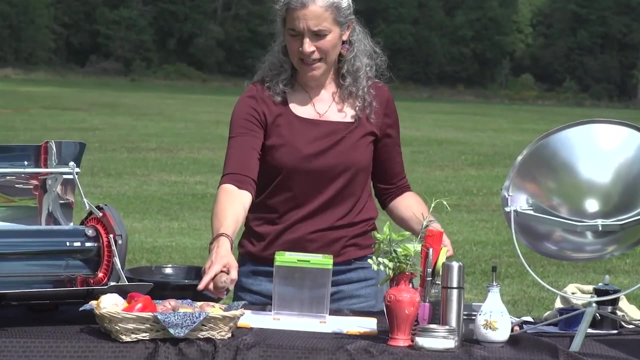 All right, I decided to stay really pretty simple here. so first of all, we're going to cook some potatoes and peppers, so the good chance to pause and talk about how we source our food right, how we get this energy source. And so all this, all these beautiful potatoes and peppers, except for 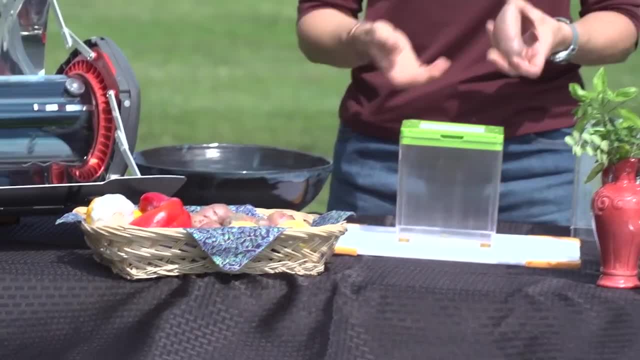 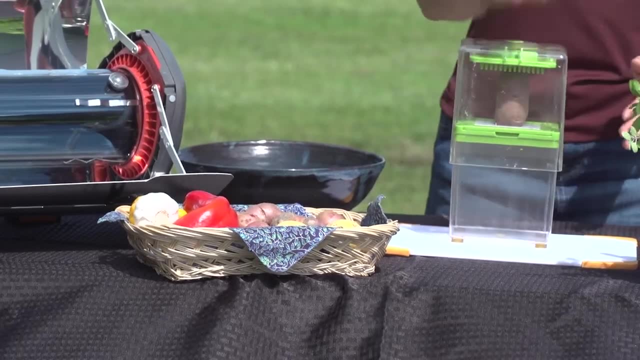 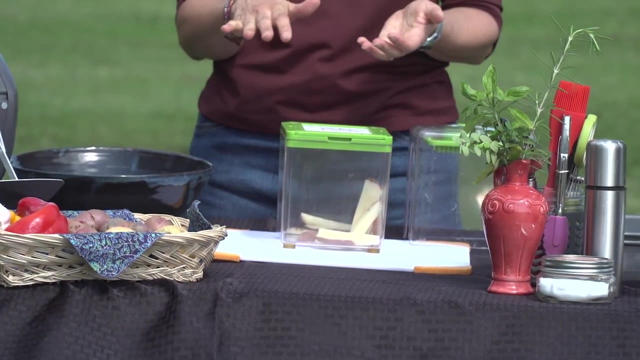 these two White ones came from the High Country Food Hub, so this is an amazing resource we have here in Watauga County. it's an online farmer's market. all the food is grown locally and so obviously we have this real benefit in that we reduce transportation energy. that's a super critical. 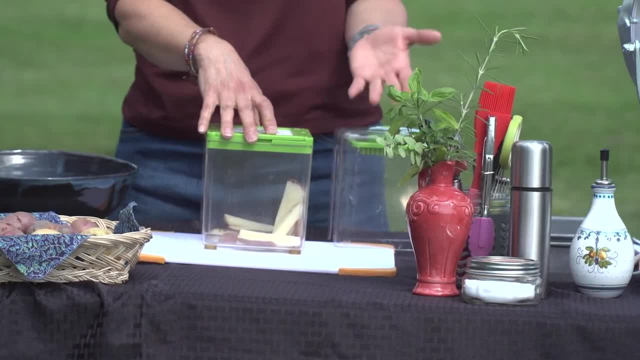 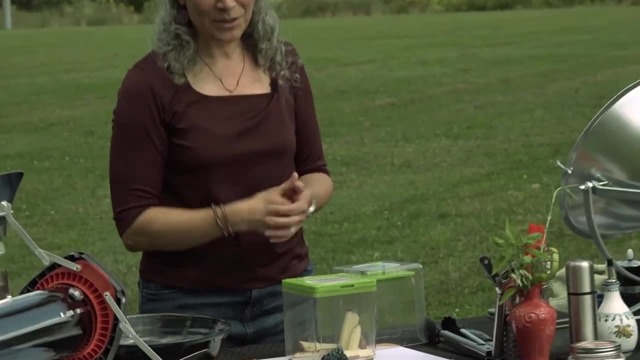 part of a local food system, but there's also a lot of other factors that may even be more important than just the reduction in transportation. We also we don't package them. so this was from Daffodil Spring Farm. So this is a local farm in Valley Cruces and they choose to package their potatoes right in a little. 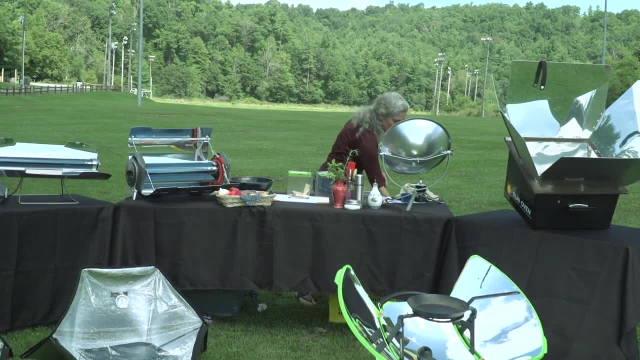 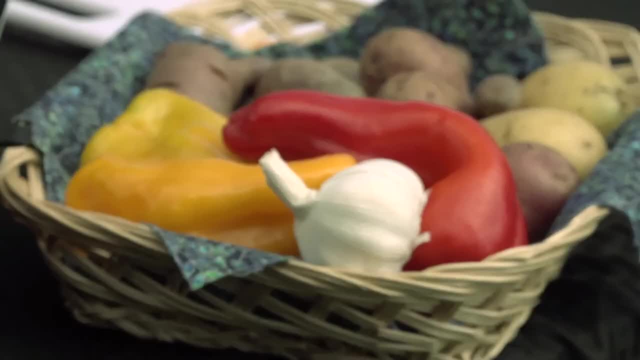 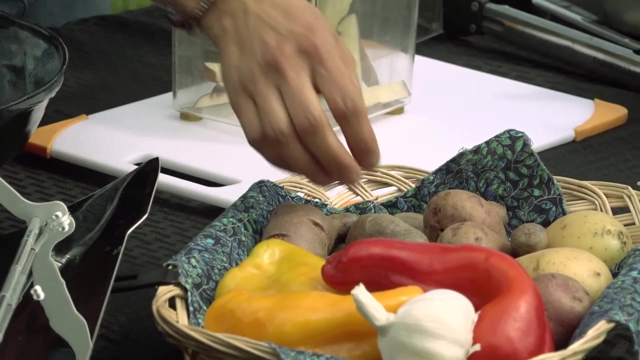 simple paper bag which will biodegrade- really simply so. if we put that in contrast to how we may buy a potato in a grocery store in a plastic mesh bag that will take 100 years to degrade. So packaging is a big advantage of choosing some local food. We have to kind of challenge. 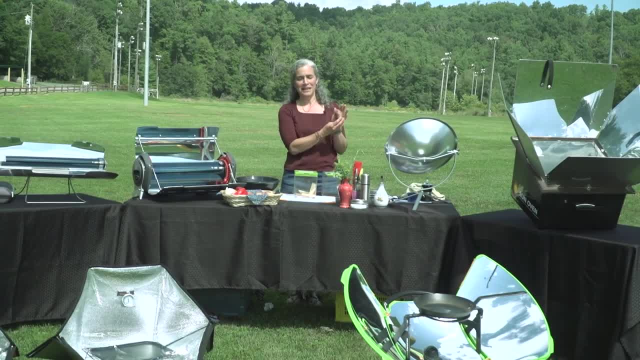 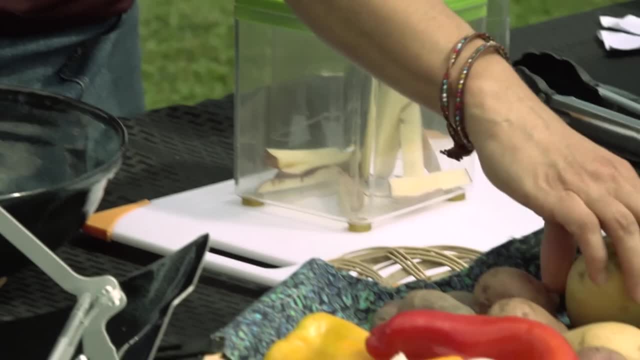 ourselves and be okay with food that's maybe not as beautiful as what we buy in the grocery store. We waste. 40 percent of the food that's grown in the United States never gets eaten. a lot of the times it just stays in the field because the farmer chooses that. it's not pretty enough for. 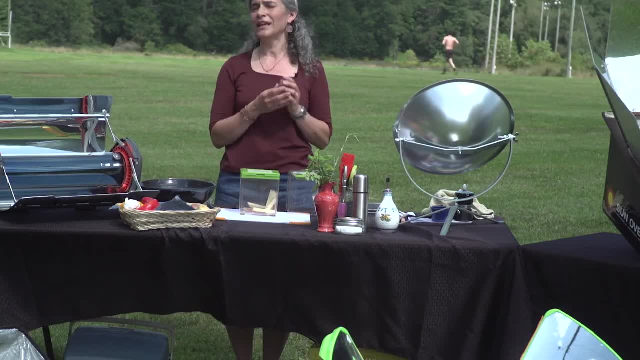 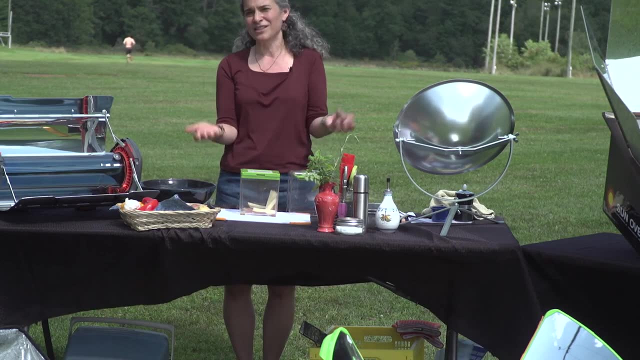 us to purchase, and so you know, it's okay. I kind of like food with a little bit of personality personally, but that's a way to recover an enormous amount of energy, because we've grown that food and then just to let it rot seems like an incredible waste. I'm going to stop talking, because this is. 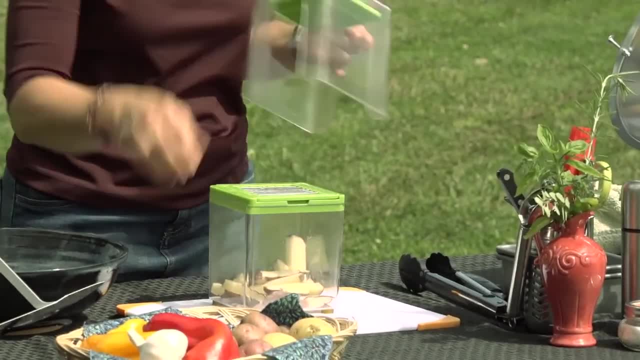 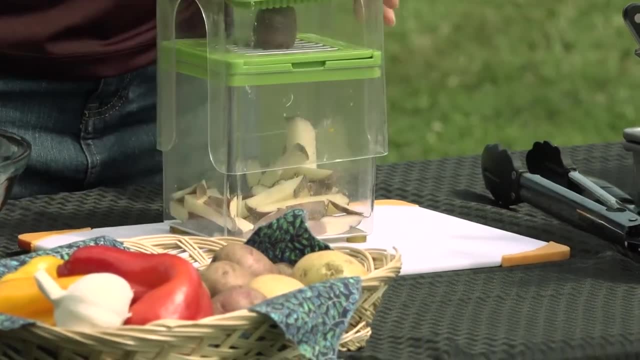 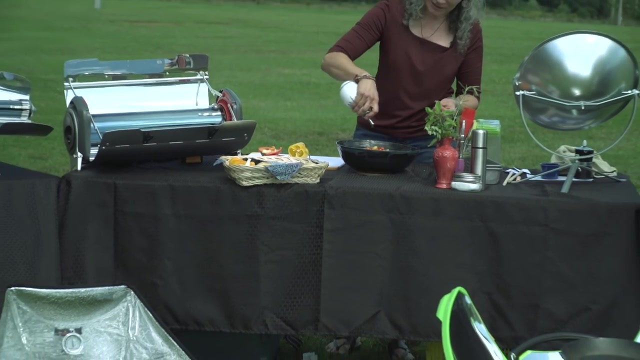 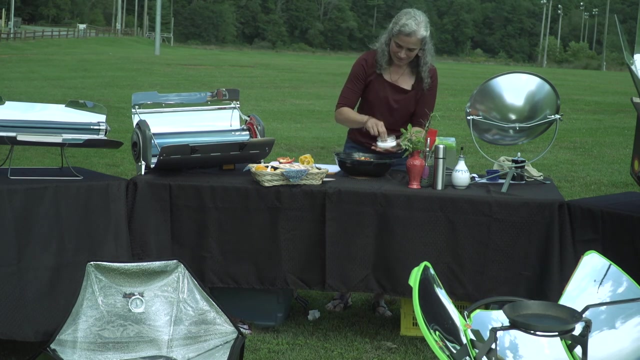 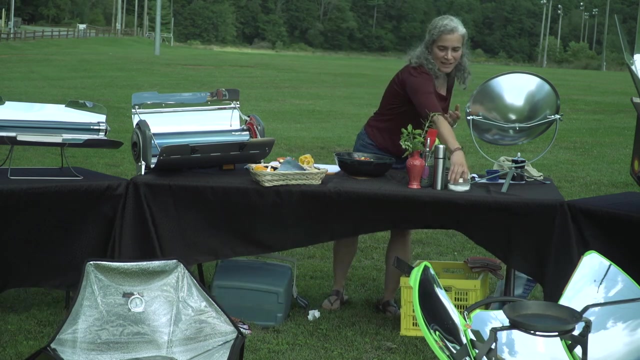 loud. All right, so we're just going to add a little bit of olive oil to that, because you know pretty much anything tastes better when you put some olive oil on it. We're also going to add a little sprinkle of salt, And a couple herbs also may be a good choice. so we have, you know, choices here as well. I harvested. 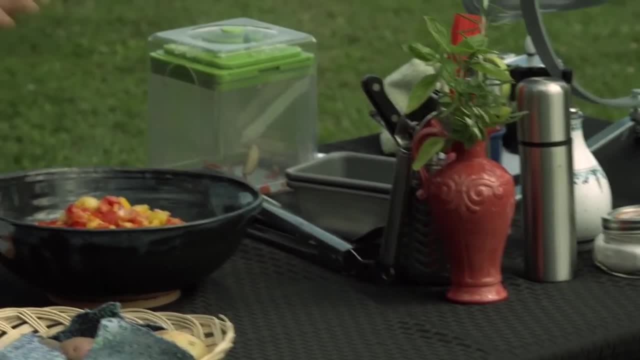 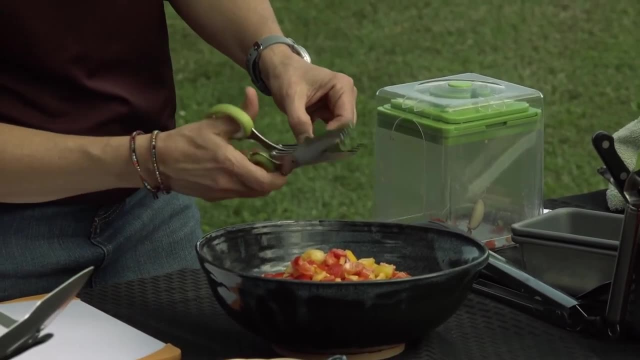 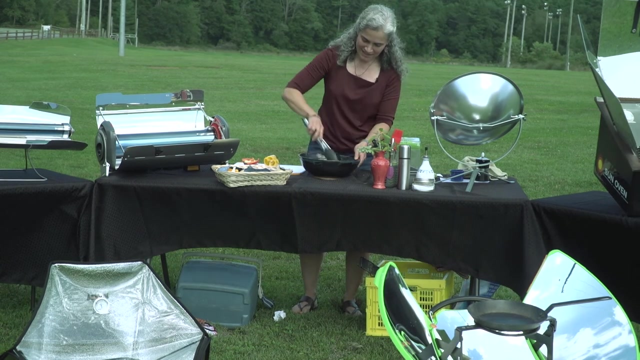 these herbs this morning from my porch right. so rather than buying herbs in a bunch of plastic packaging, this makes a really easy crop we can all grow at home, and these little scissors make chopping these things really super easy. I do wish you were all here and live so we could do. 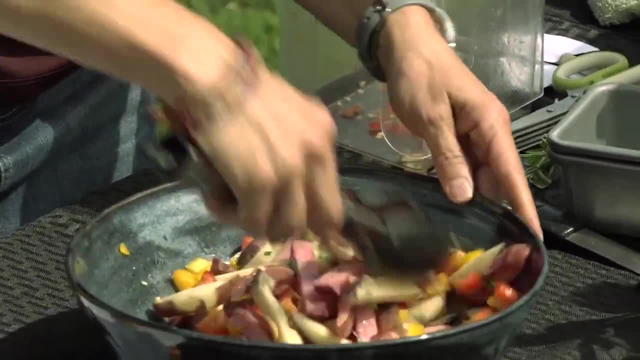 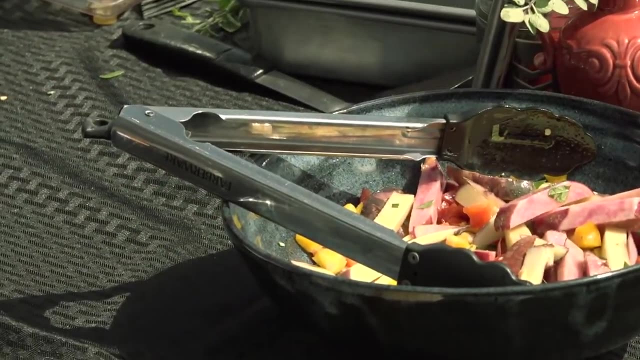 some tasting. at the end of this cooking demonstration, I'll let you know how it tastes. Okay, perfect. so that's one of our, one of the things we're making. The other thing is already made. so I also was going to cook some hamburgers, and so if we 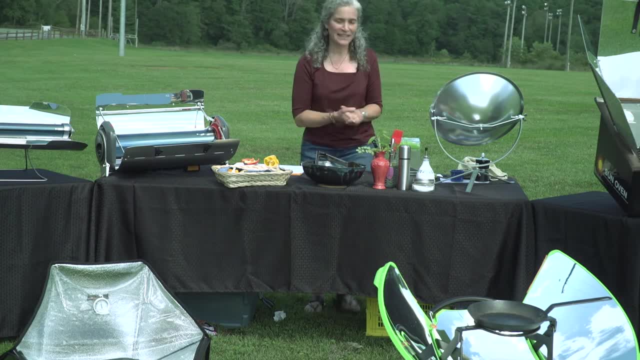 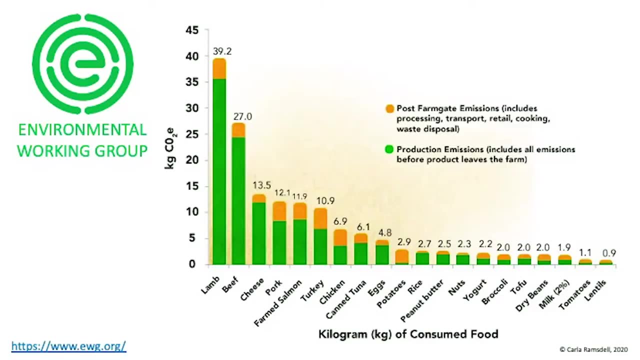 uh, look at this graph. it's a good time to talk about the impact of our food choices on our greenhouse gas emissions. So this graph is issued by environmental working group and it shows the range of our greenhouse gas emissions based on different food sources. So we see, beef is all. 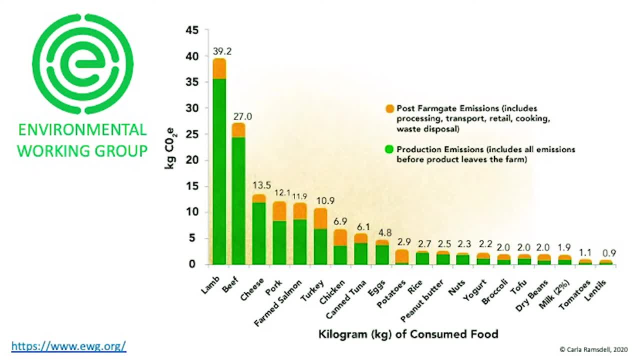 the way over on the left here with many kilograms of equivalent carbon dioxide emissions and we see on the right hand side we have lentils and a lot of our dry beans and legumes. So the further we can eat to the right hand side of this graph, we will get even more of the oil and the replicas and the. 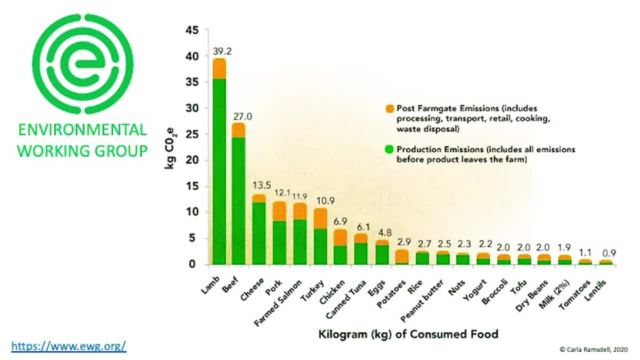 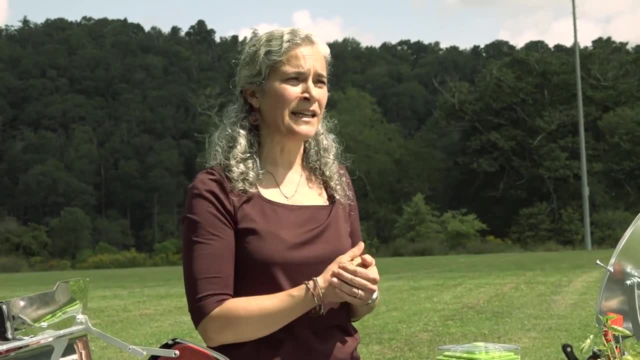 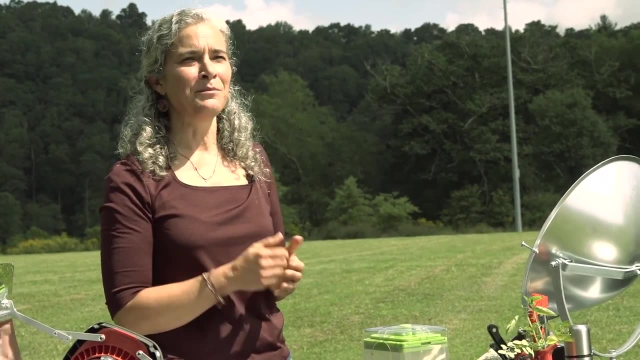 curve, the less greenhouse gas emissions are emitted from our food choices. So really good news is that lately a couple of companies have gotten behind this plant protein concept and created some burgers that taste remarkably like a beef burger. So Impossible Burger and Beyond Burger right now are the two companies, So I was going to go ahead and just cook some. 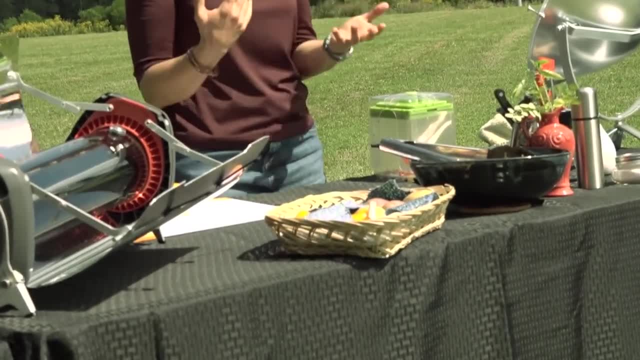 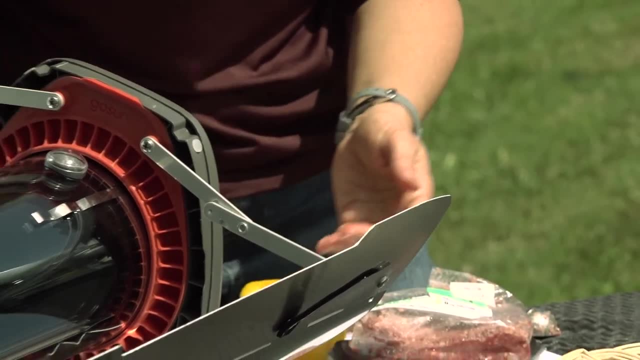 Impossible Burgers today, so we can see exactly what those look like and I will tell you what they taste like. If you haven't tried these yet, I would encourage you do so. They actually serve them at Burger King. right now. The Impossible Burger is available there, but you also can. 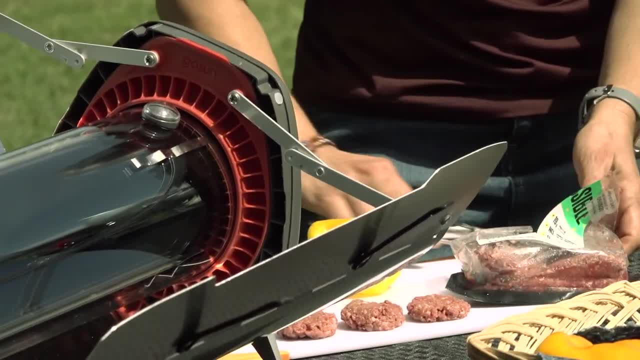 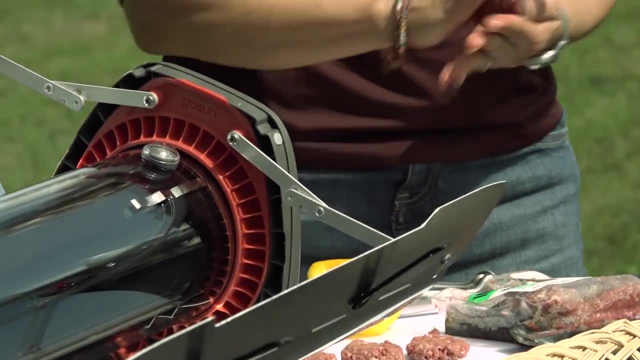 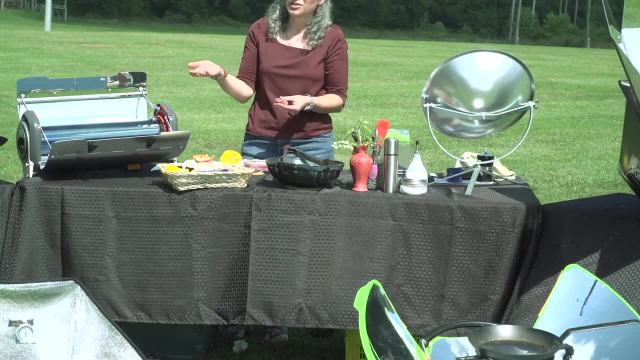 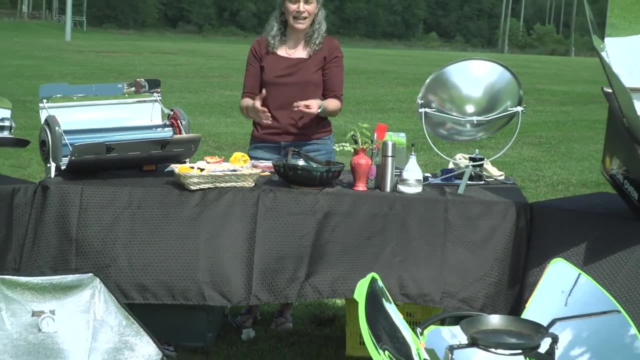 energy we need, And we'll get all the energy we need, And we'll get all the energy from that corn. But instead, if we feed corn to a cow- which we probably shouldn't anyway, because cows aren't supposed to eat corn, but if we did, only about 10% of it is converted into the cow's meat. that 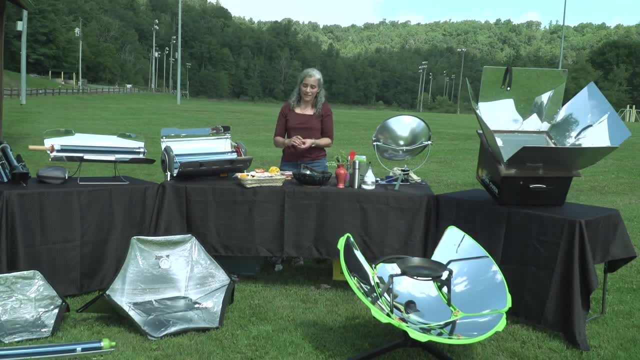 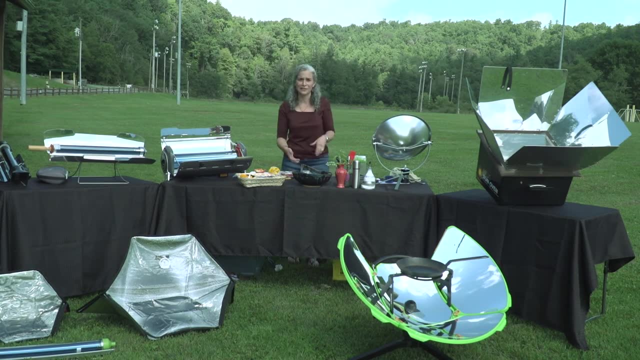 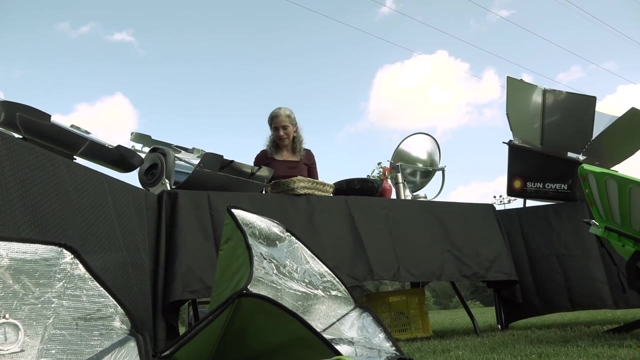 we may then consume. So we've had a 90% reduction in the available energy of that initial food source because the cow had to do all the things a cow does right, Like live and whatever So and breathe and move. And so, yeah, the lower down on the food chain we eat, the better we will be. 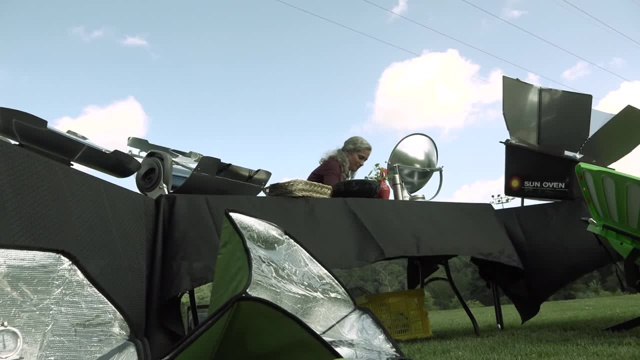 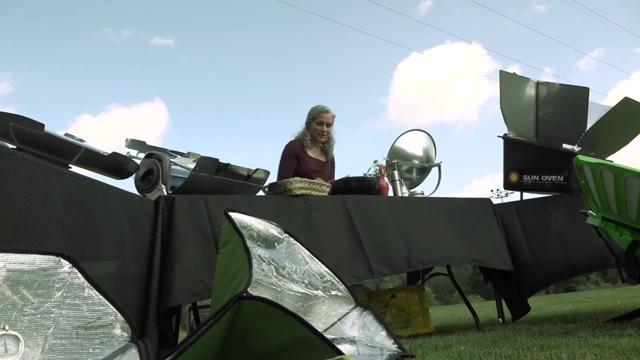 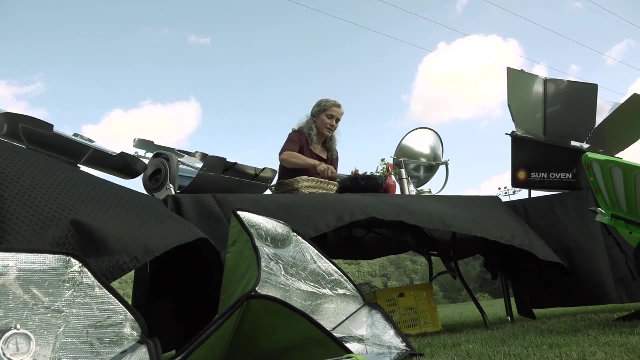 As far as our energy conservation. Okay, so I think we're ready. We're going to go ahead and load our ovens. We're going to put two burgers in each oven, And then also these potatoes and peppers. Split this in about half. We're going. 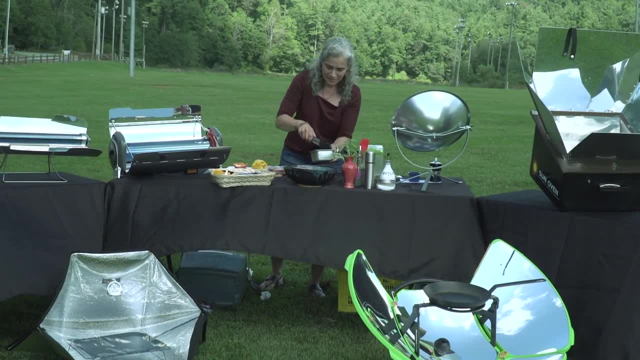 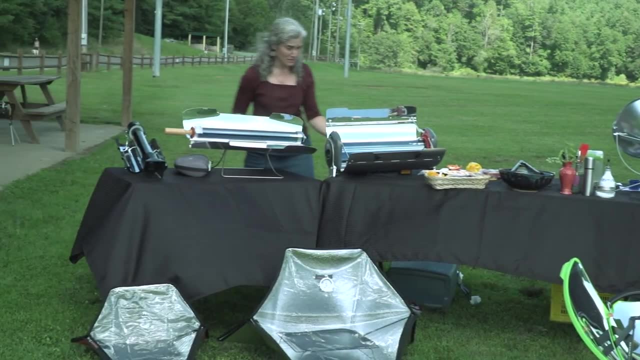 to talk about the different kinds of ovens that I'm using here in a moment, But again I'm just going to load these up. Unfortunately, we have had a cloud show up on our cooking scene. That's unfortunate, but that's okay. 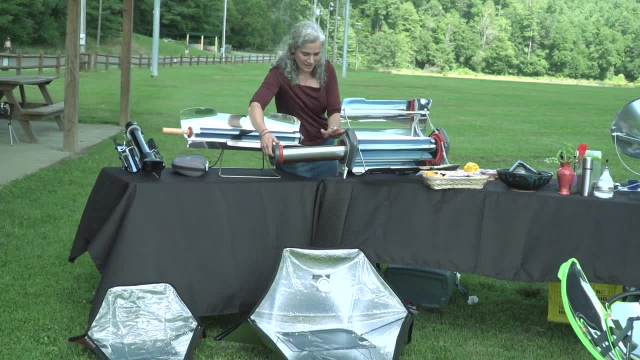 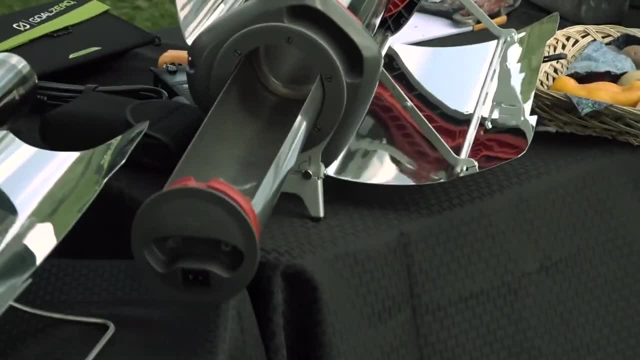 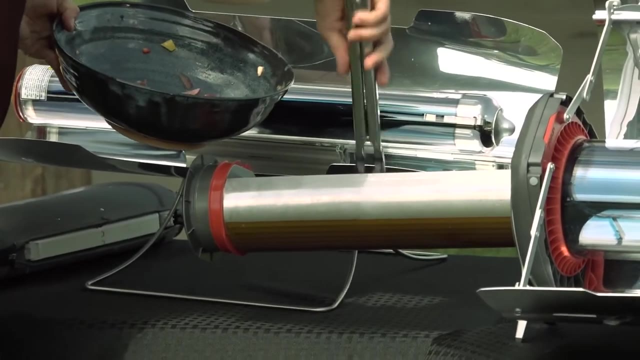 We'll see if we can pull it off anyway. So half of them are going to go in this evacuated tube oven. This is called the GoSun Fusion. It's the latest and most advanced solar oven on the market right now. Perfect, I think that's ready to go. I'm going to put another scoop of that in there. 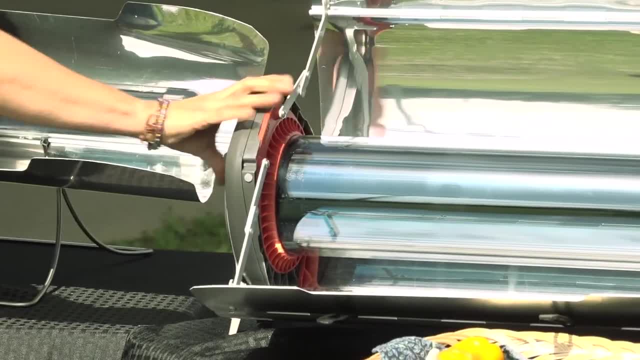 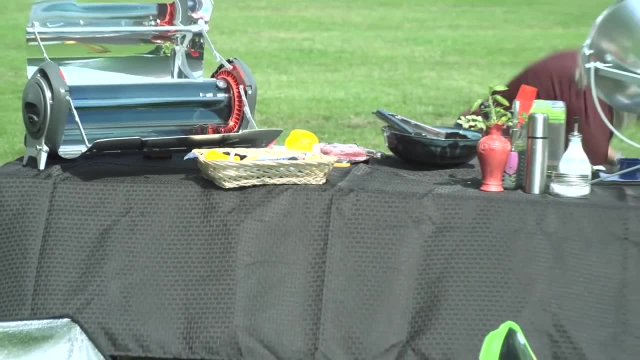 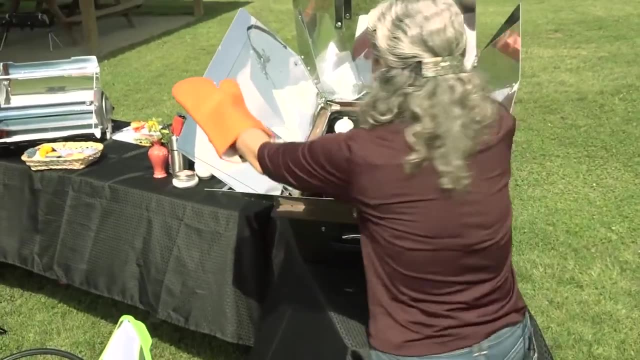 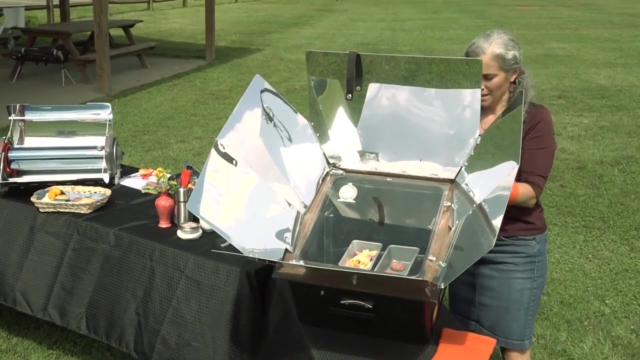 Okay, we're going to just close that up and give it a good seal, And then we're going to go over here to our box oven. Okay, We want to make sure both of these ovens are focused well into the sun, Casting a symmetrical 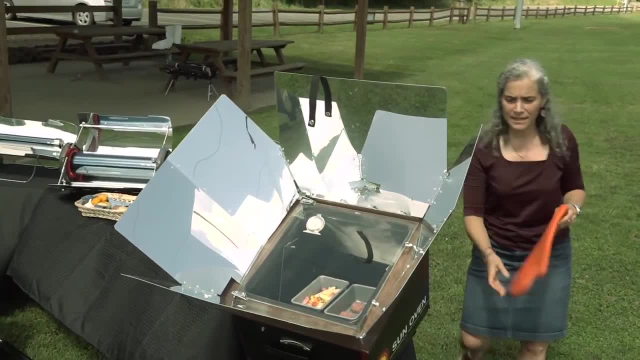 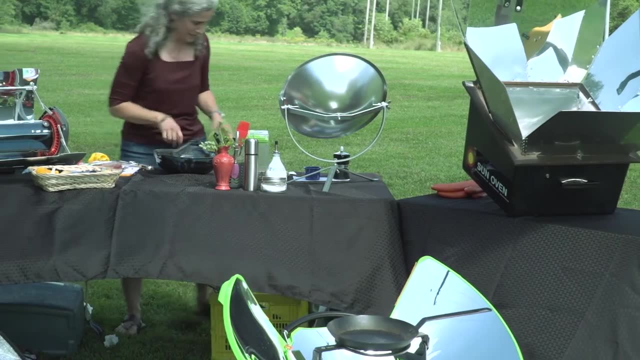 shadow. There's a lot of different mechanisms these ovens give us, so that we're sure that we're focused properly, All right. So that's that, All right. All right, There's our main course, but no meal would be complete without a little bit of dessert. 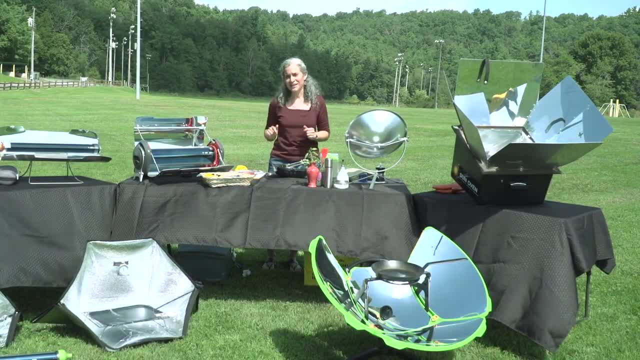 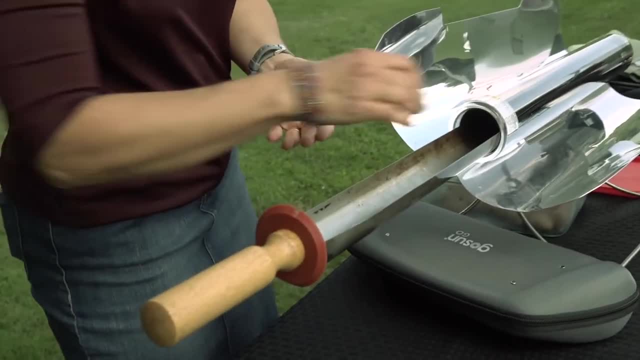 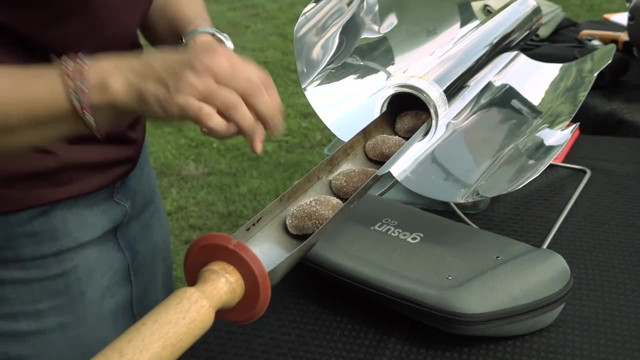 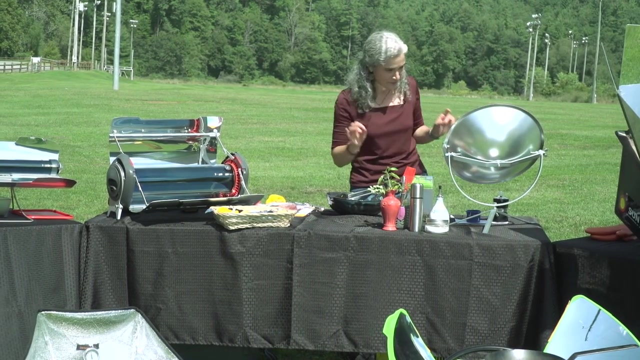 So I also made some ginger snaps ahead of time that I'm going to go ahead and cook in this evacuated tube down here. So All right, so we're just going to load up these ginger snaps And, you know, just to make the meal complete, we need a little bit of coffee. 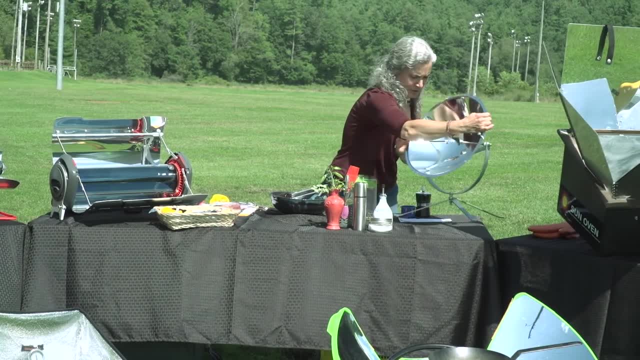 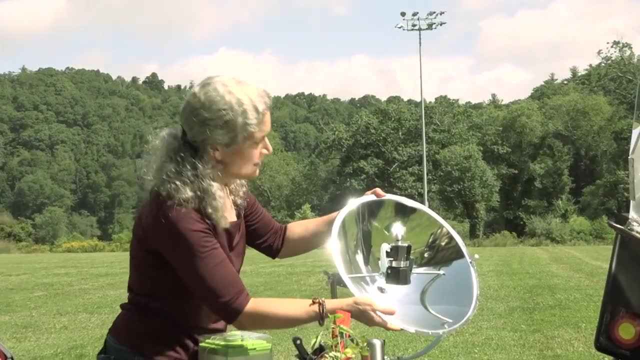 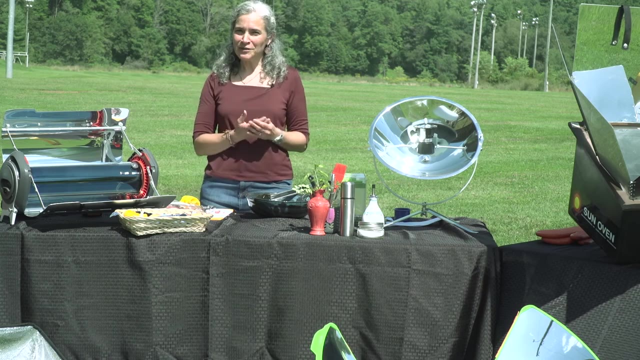 And so I'm additionally going to to brew a cup of espresso in this parabolic reflector. Get that focused right as well, All right. So while that's all cooking, let's talk for a bit about these different kinds of solar cookers. 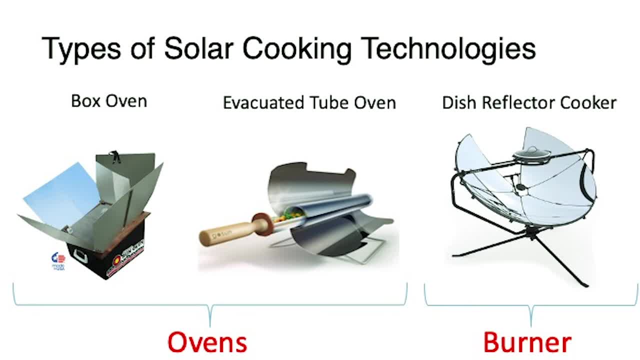 In general, solar cookers can be divided into two categories. One of them are solar ovens, Right, These are things that are designated to replace the oven In your home. So, and among the ovens, we have kind of two categories. 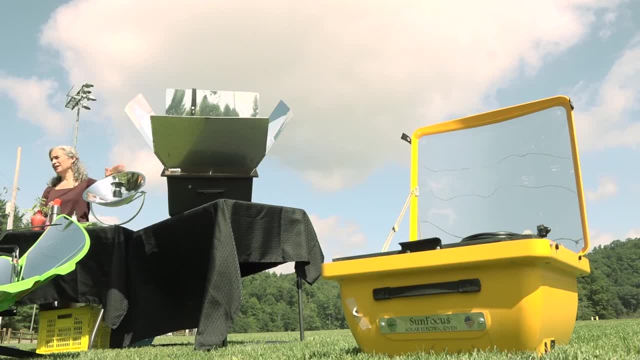 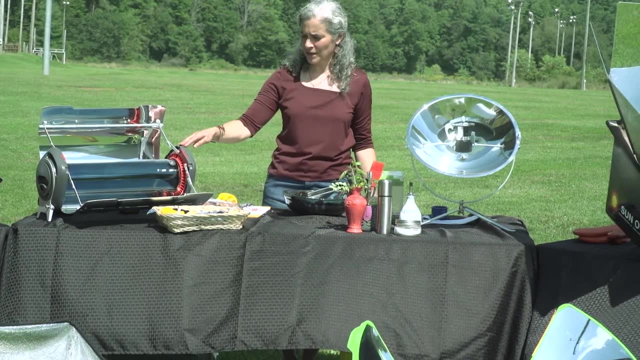 So we have box ovens, which would be that one over there, the sun oven, and then also this yellow one on the ground, And then the other category would be evacuated tube ovens, And that's what we see over here. Most of these are by the company GoSun, which is definitely the leader in this kind of technology. 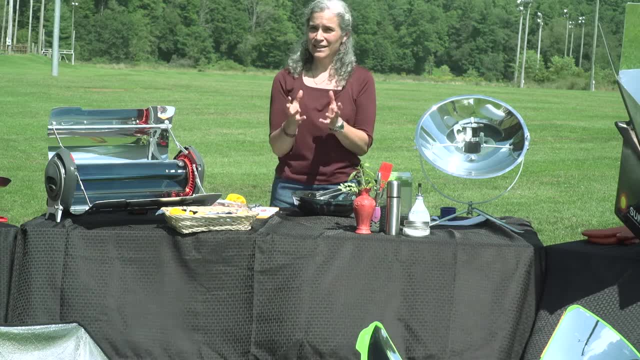 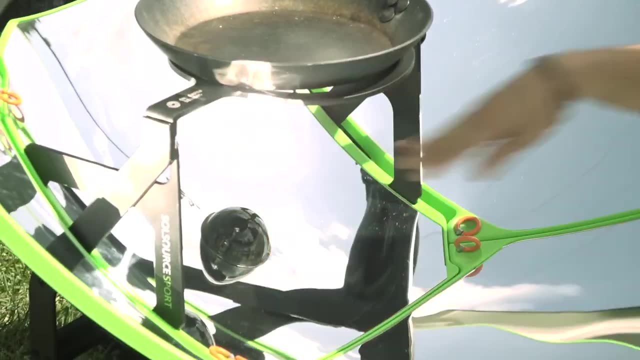 And the other category of a solar cooker is a reflector And that is more to replace your cooktop or range, And so we see down there. So it's a solar, solar source, And also we have a couple of these solar flares. 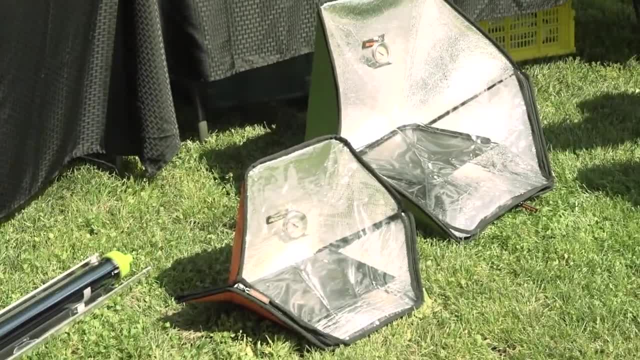 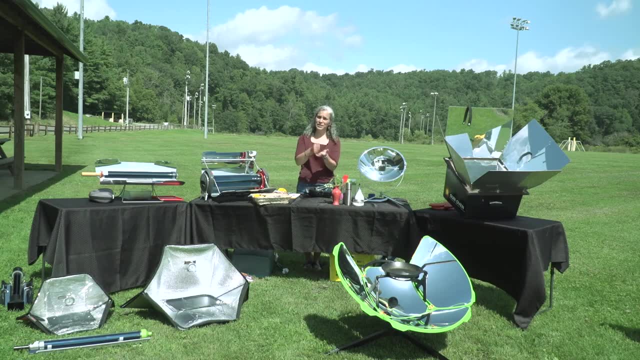 Those are more about reflecting onto a cooking surface such as a skillet or a pan or something along that nature. This, right here, our espresso maker, is also like that. You would normally put the espresso on the range top, And so this is replacing the range top. 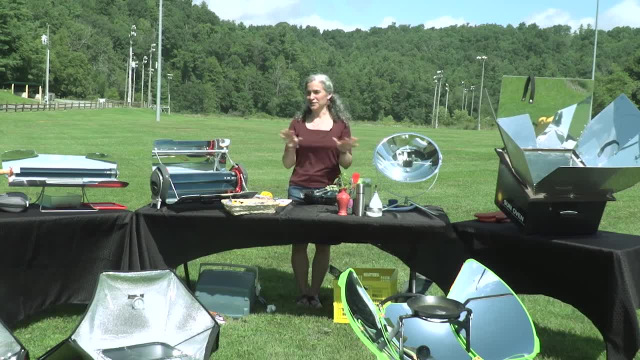 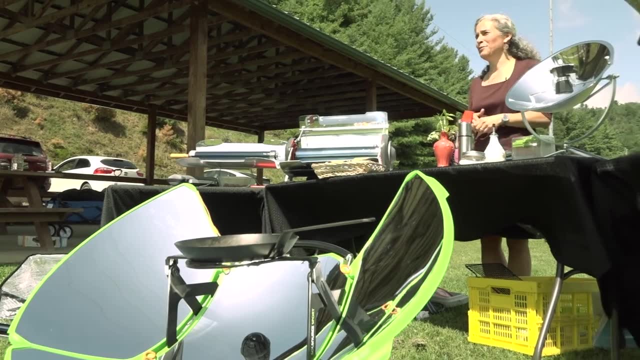 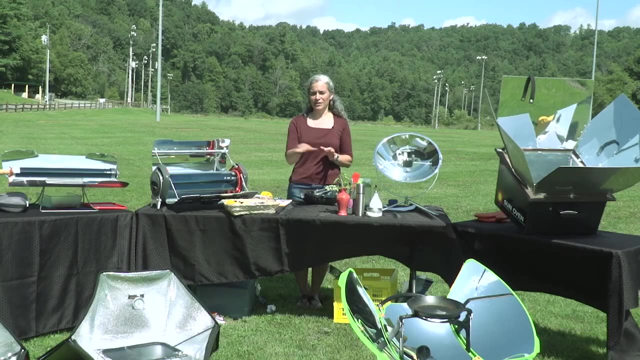 So let's start with talking about the physics of the ovens first, Right, So any of these ovens? the keys are to obviously maximize solar incoming radiation. Right, We want to try to scoop up as much solar radiation as possible. As I mentioned, there's about a thousand watts per square meter on incident on the surface of the earth. 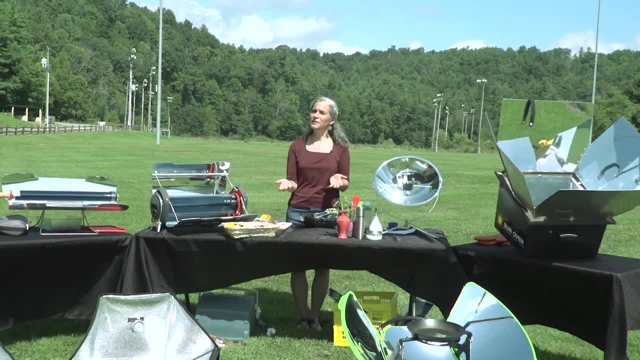 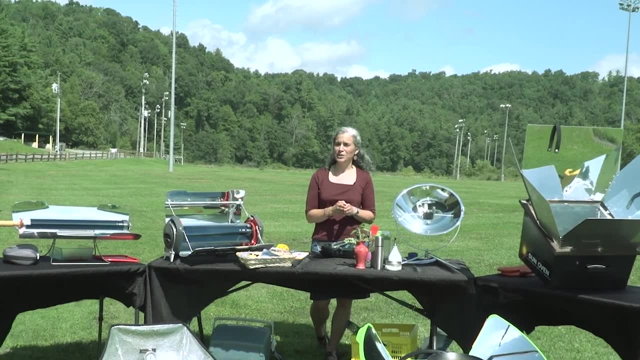 But when you turn your oven on at home to you know, bake at 350, it probably is about three thousand watts of power that it draws to accomplish that. So there's a couple of things that we do to make these more effective. 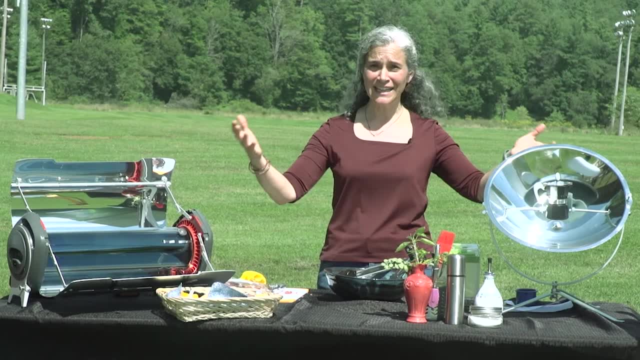 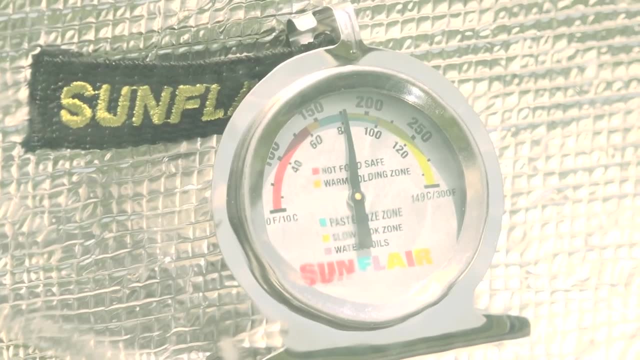 One of them is to make the volume of the oven smaller, Right? So if we don't have to heat up the 30 pounds of steel that's the oven in your home, Well then that helps us, You know, and if we have a smaller volume, obviously we're trying to keep a smaller space. 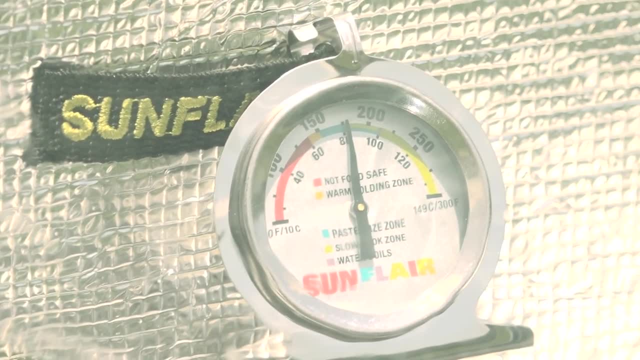 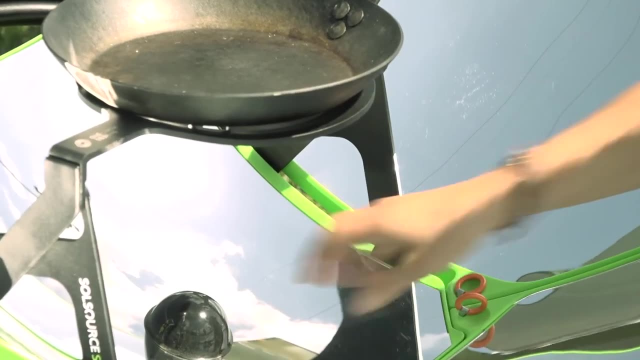 So you see, most of these ovens are pretty small in space. And then the other thing we do is we try to scoop up more sun than what is just incident upon the oven itself, And, as you can kind of see, that is done predominantly with reflectors or mirrors. 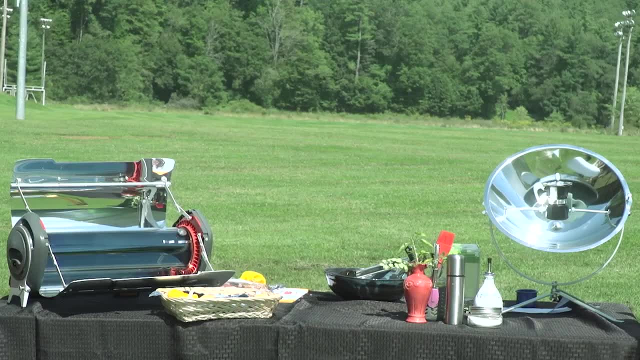 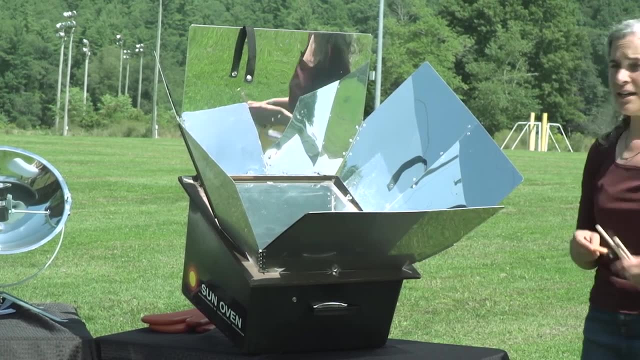 So let's go to the physics of that just for a minute. in order to to understand how these mirrors are reflecting thermal energy into this oven, We are going to rely on this, This nerf dirt. So if I put the nerf dart on one of these reflectors, 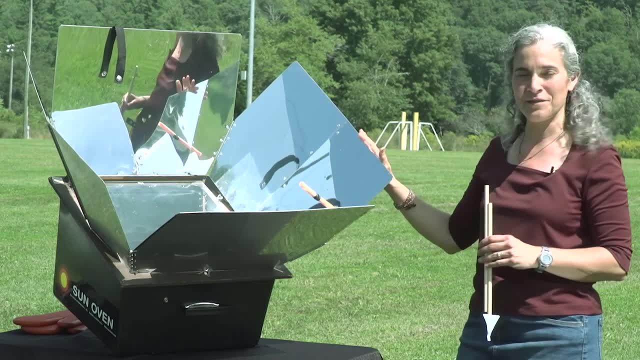 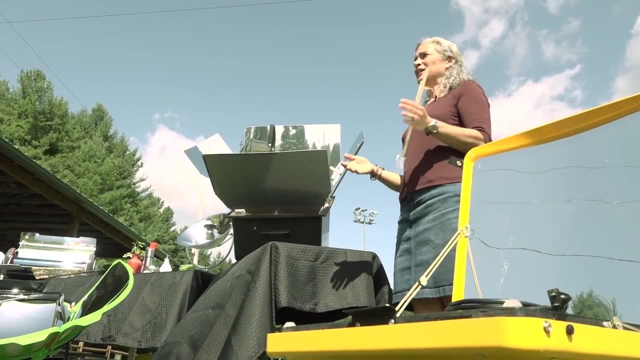 Right, I show what is the perpendicular to this reflective surface. And then we rely on, in physics, the law of reflection, And that says that the angle of incidence equals angle of reflection. So if the solar radiation is coming into this oven perpendicular to the surface, 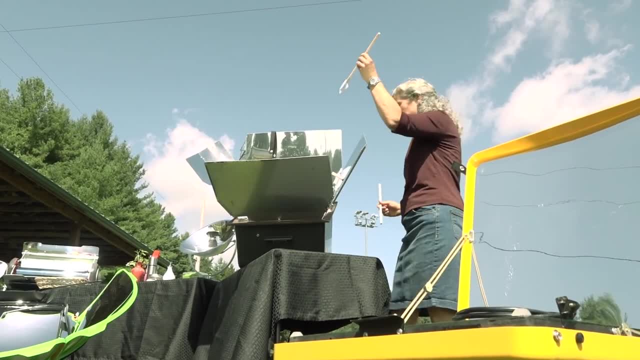 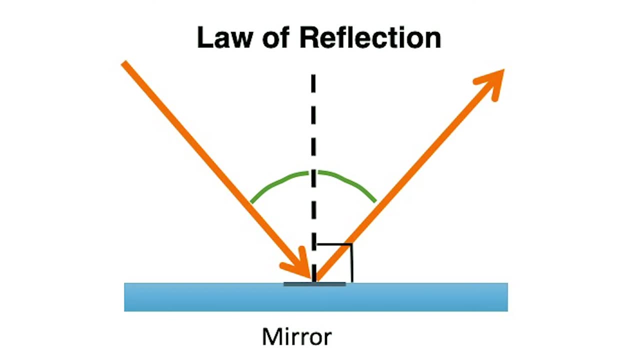 Right, We can imagine that as this sunray right here, Right, So we're going to come in sort of perpendicular to the surface and is going to be incident upon the perpendicular to the surface, to this reflector, And then what we know is, whatever angle this incoming beam is making with the 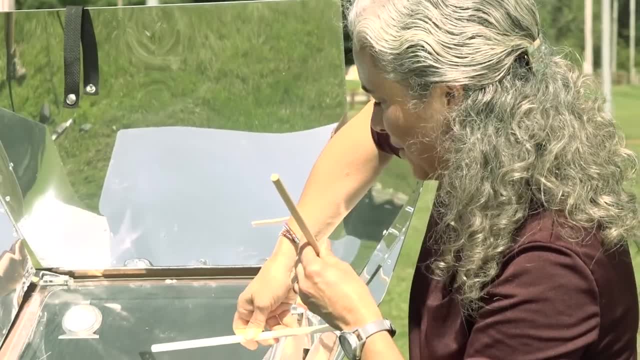 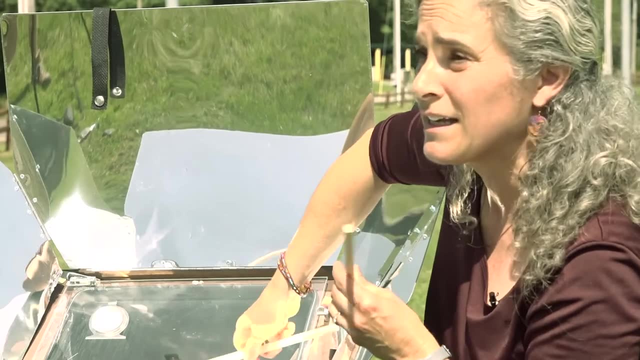 perpendicular will be the same angle on the other side of that perpendicular. So the angle of incidence is equal to this angle of reflection, right, And so we see if this is coming in parallel. well, this guy is going to make it into the 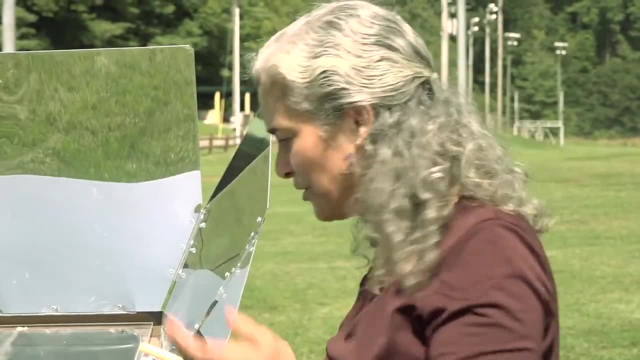 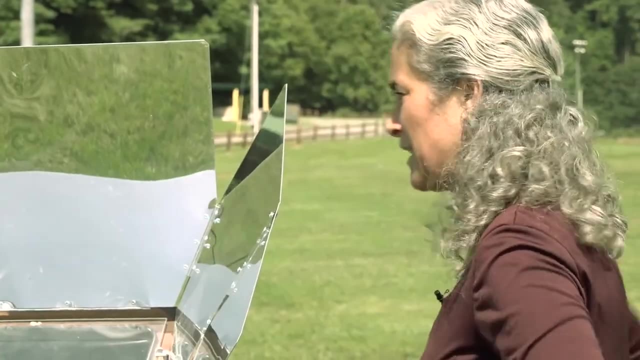 surface, we do lose- lose a little bit of energy upon a bounce, but not much right. And so, rather than just relying on the energy hitting this glass surface now, we can scoop up a much bigger space. we see the same thing happening down here. 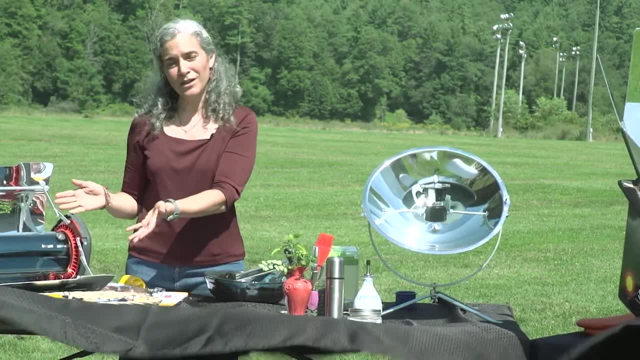 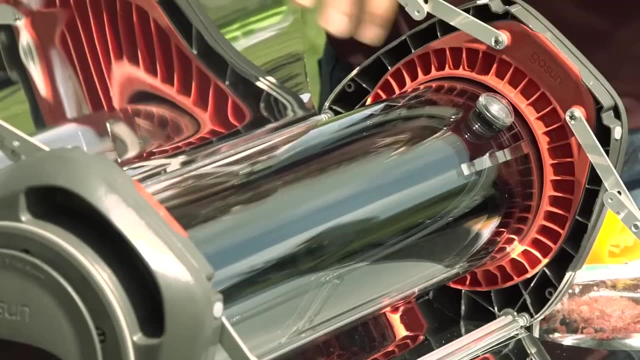 with our evacuated tubes. this gets a little more complicated, because we're no longer just reflecting onto a flat surface, But we want to reflect on this, this line here, And so what we rely on there, then, is a parabola, And if you don't, 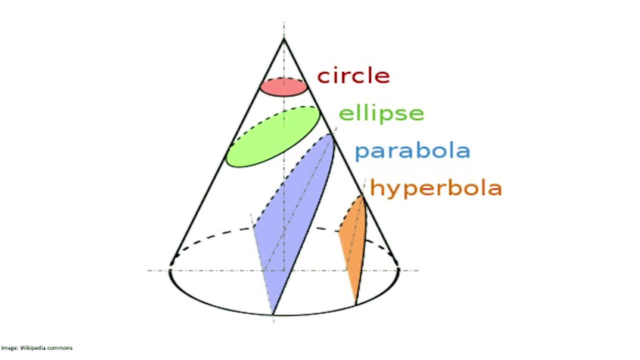 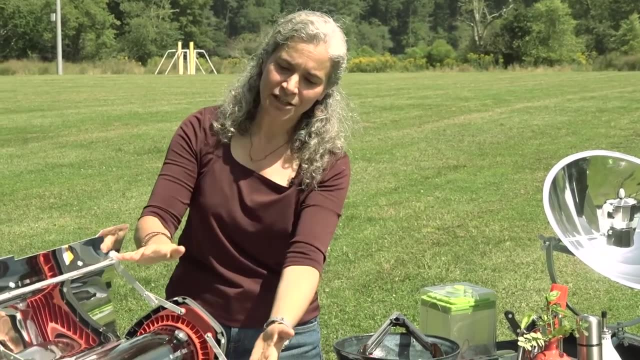 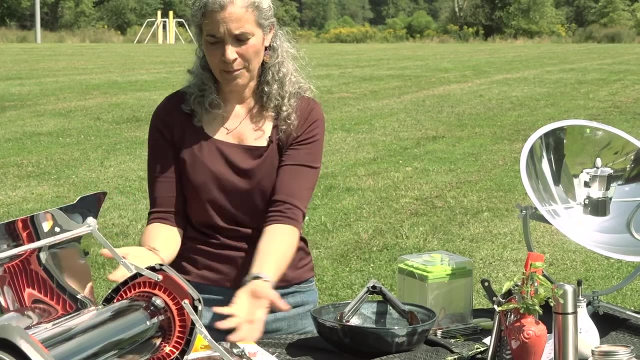 remember from geometry, a parabola is a slice through a cone And it ends up that, maybe counterintuitively, if you have incoming radiation coming in straight, in sort of perpendicular to this whole oven arrangement, then the focal point off of a parabola shape 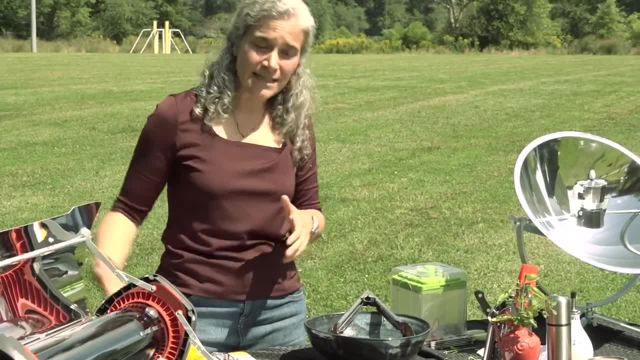 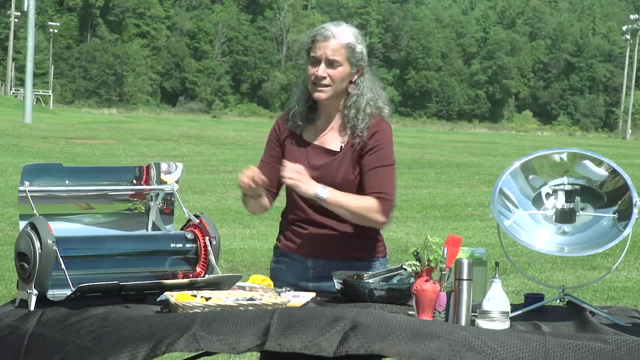 will be on to a central point. If you instead chose a semi circle, well, the focal point then would be along a line, and some of the reflection from the surfaces would miss the oven completely. So it's important that all of these circular 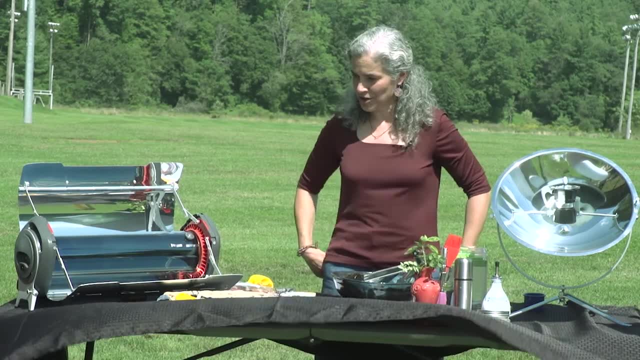 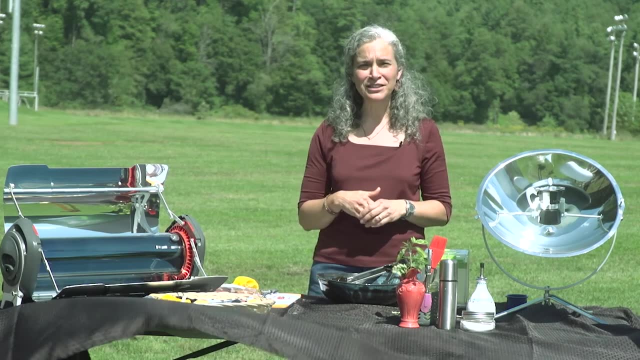 reflectors are based on a parabolic shape other than a circular shape, Alright, so we want to make sure that we maximize radiation gain. Part of that is by these reflectors. Also, in the case here of the evacuated tube. this is a really fun thing to. 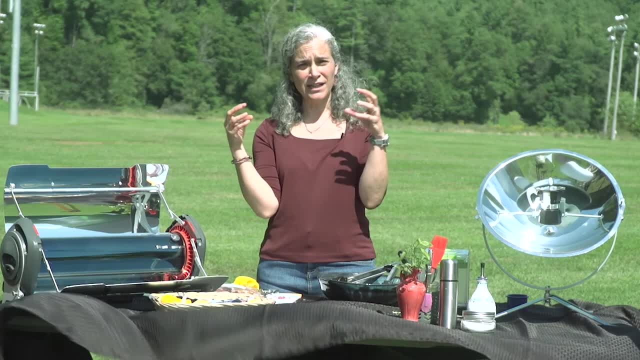 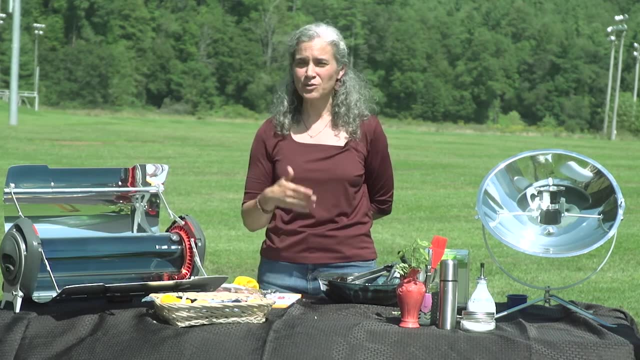 talk about. So evacuated tubes are two concentric cylinders inside each other. The outside is all out of borosilic glass, which is what most of the Pyrex in your kitchen is made out of. It has very good transmissivity, which means it allows the solar 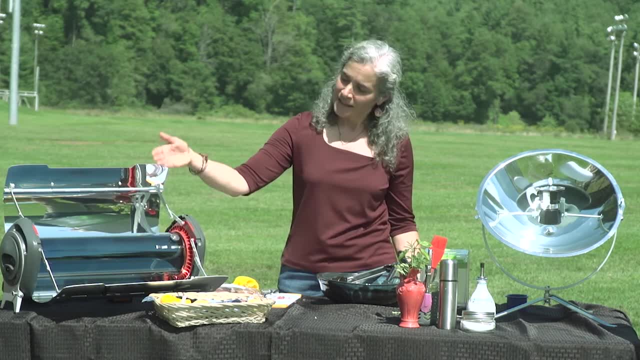 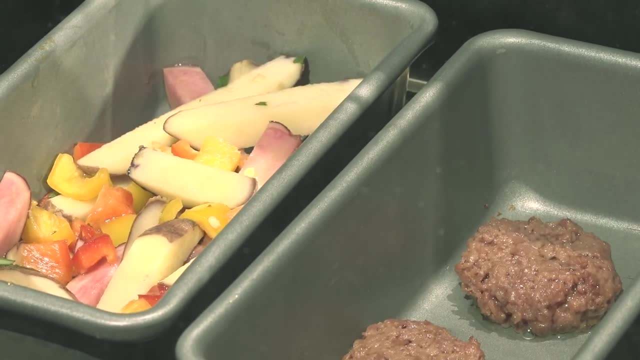 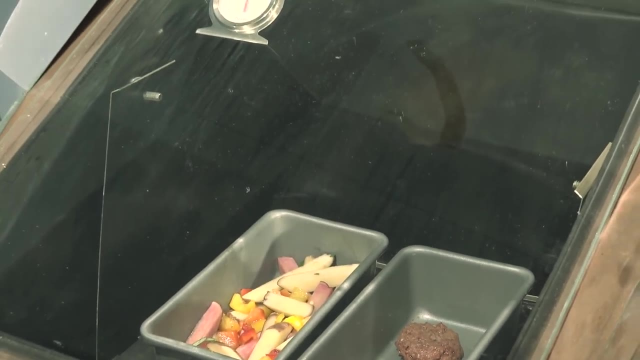 radiation to pass through this outer surface very easily. Then we coat the inside cylinder with a solar selective material that is very effective at absorbing solar radiation from the Earth's wavelength, from the sun's emitted wavelength right. So what we know about radiation is that the intensity of the 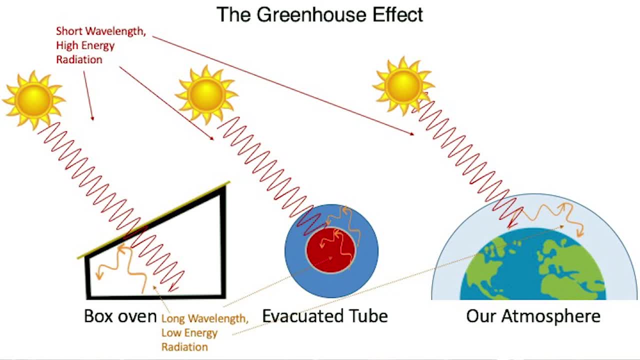 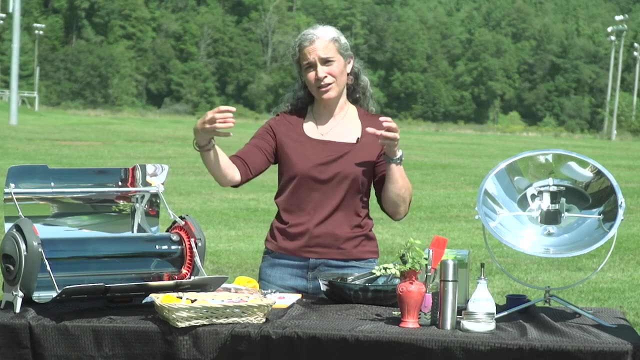 radiation is dependent upon the body that emitted it. So the sun that has a 9800 degree Fahrenheit surface temperature emits radiation that is very intense, very short wavelength. So we want to make it through this outer cylinder with no problem and gets absorbed by the coating on that inner cylinder. 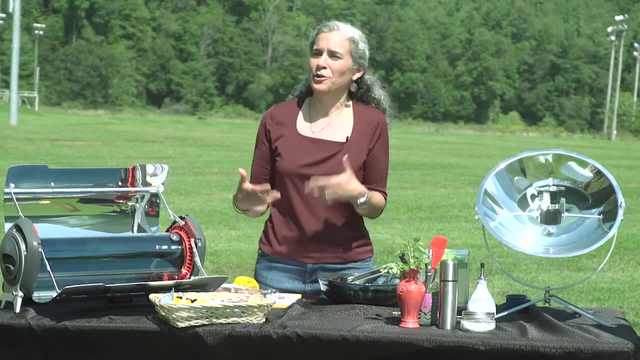 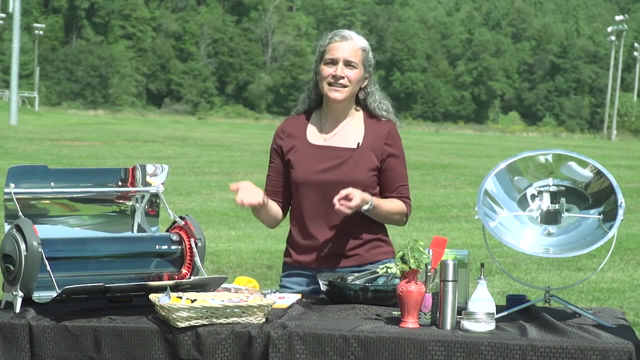 That then warms the oven. The oven then re-emits its own radiation, right, But because the oven temperature is significantly less than the sun, the solar radiation it emits is at a much lower intensity. And so now, as it tries to make its 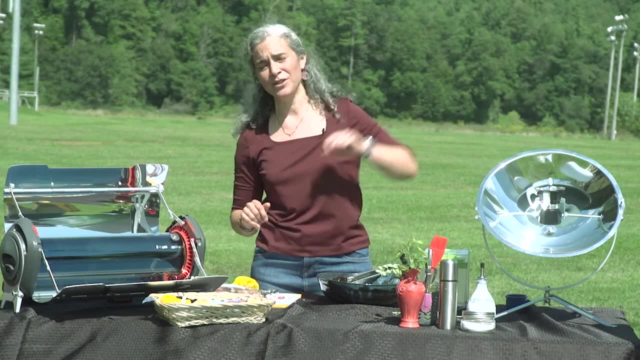 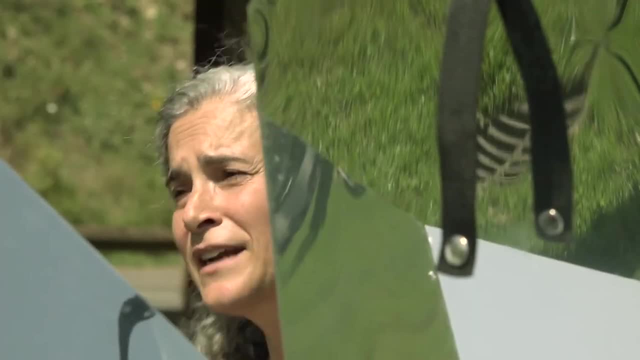 way out it's blocked by the outer glass surface. or, for example, in that in that oven the glass top of the box right it gets blocked- The greenhouse effect. it's the same way a greenhouse works. It's why, as we throw more greenhouse gases into the atmosphere, we 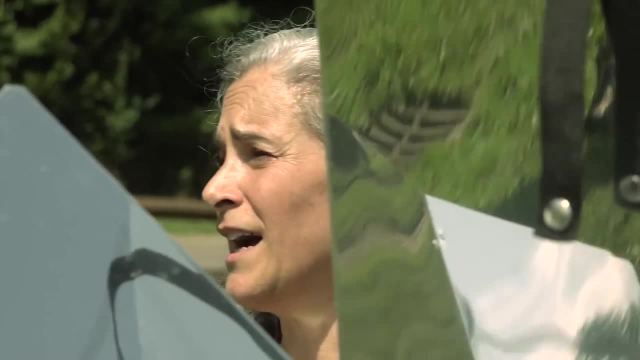 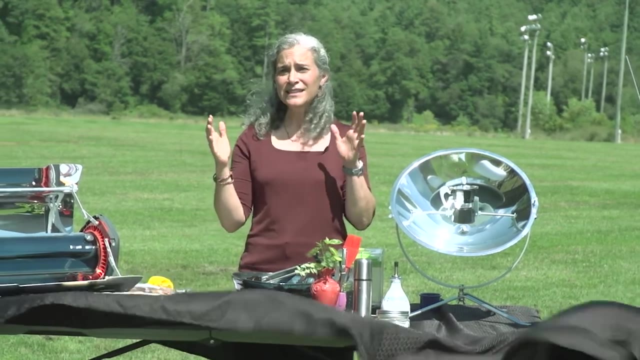 have this buildup of thermal energy because the short wave high intensity radiation can make it through without much trouble, warm the Earth's surface, But then, as this longer wavelength radiation tries to make its way out, the greenhouse gases or glass on the oven trap it and keep it within the system. 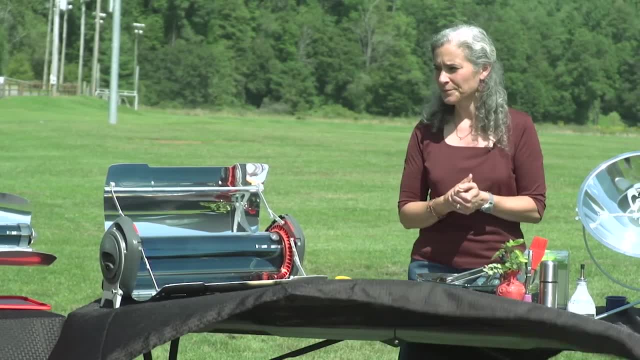 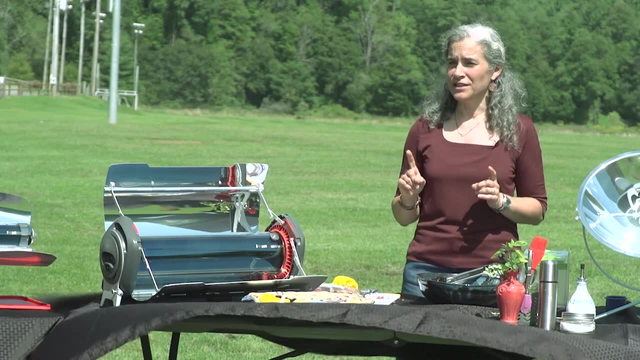 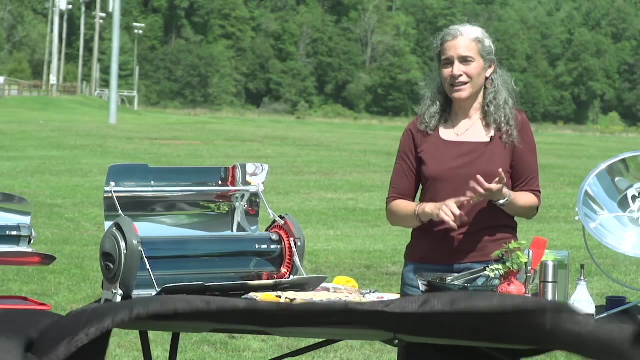 And that helps to circulate this energy and warm it more and more. Perfect. So the other thing that we we do here. so while we're maximizing radiation gain, we're also trying to minimize heat loss, And heat can be lost through conduction, convection or 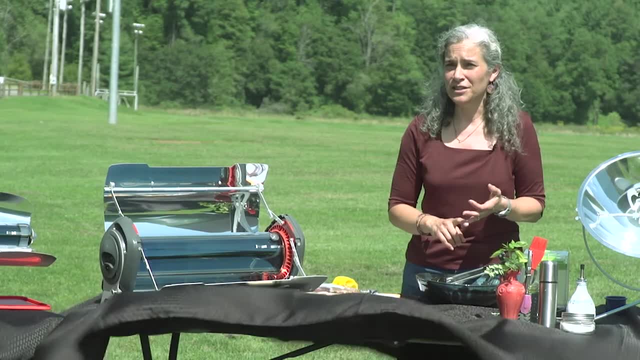 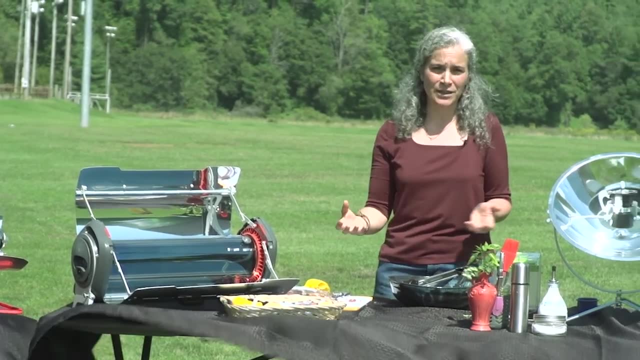 radiation. It ends up conduction and convection. both need a medium. they need some things right. So conduction is the transfer through a medium without the movement of the medium itself, And convection, we know very well as the wind is. 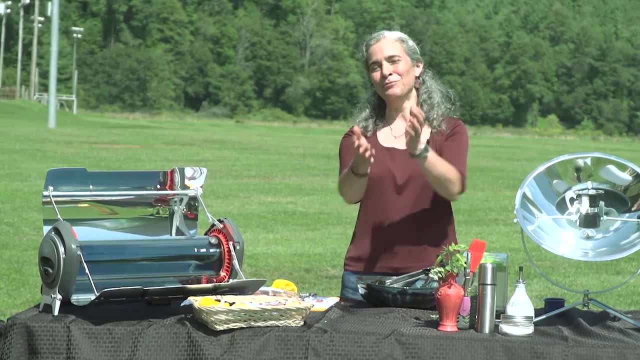 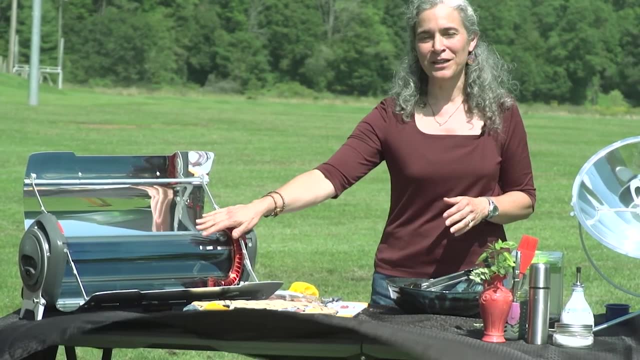 blowing is the transfer of thermal energy because of the movement of a medium right. So, as this wind blows, it's cooling me off on this sunny day, which I am appreciative of. So what we do in an evacuated tube is we evacuate it, that space between. 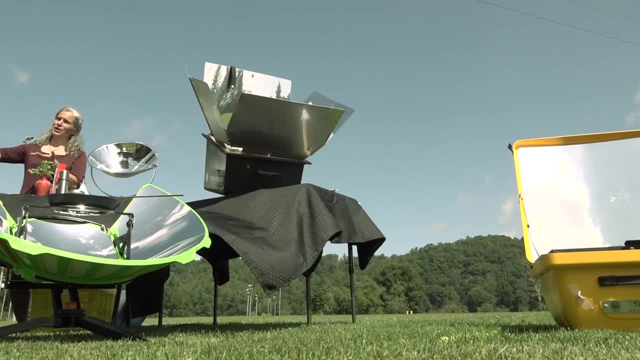 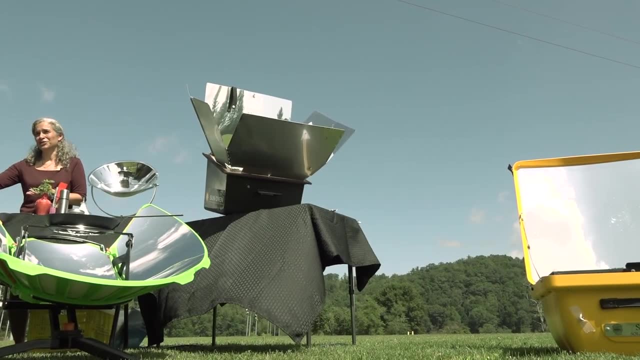 the inner and outer cylinder has all of the air molecules, everything sucked out of it, removed. So there's a negative pressure between these two cylinders. It's why it has to be cylindrical, because we couldn't hold that kind of a vacuum in another shape, like a square. 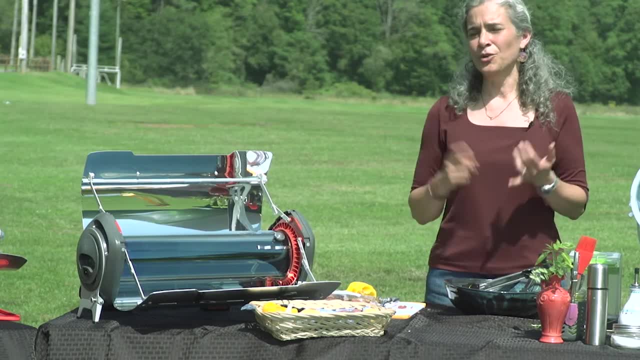 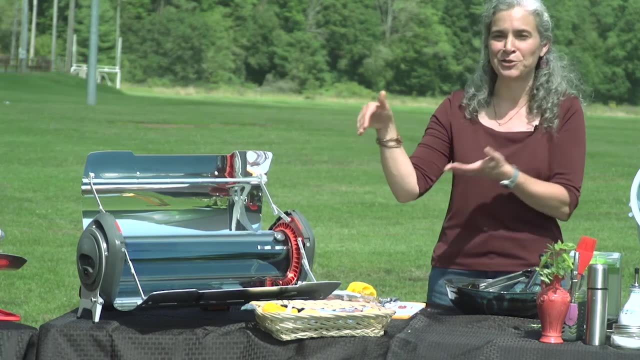 So by doing that, by removing the molecules, we've removed the medium. So once we gain that radiation in the middle of the oven, we can't lose it by conduction and convection, because there's no stuff in between these two layers to 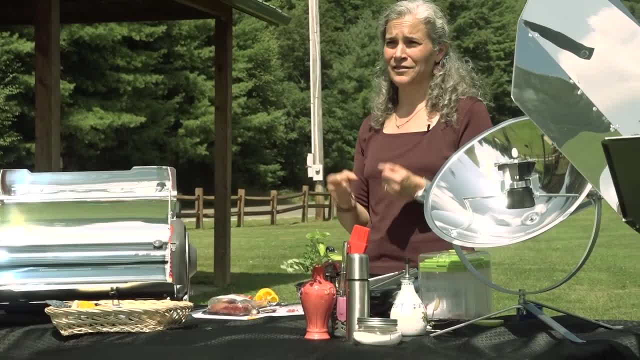 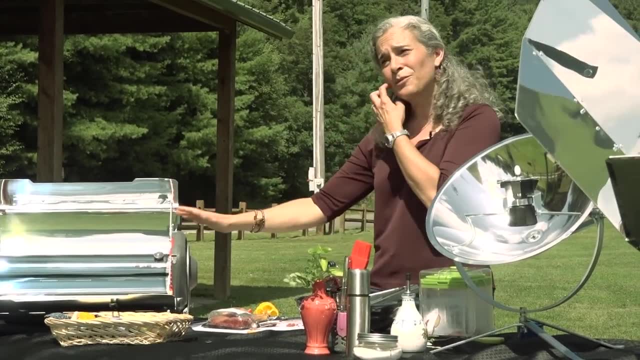 accomplish that. In the same way, your mug right may have a vacuum sealed mug. the same thing we're trying to block the loss due to conduction and convection. So that's really what makes these rock stars on efficiency right, All these. 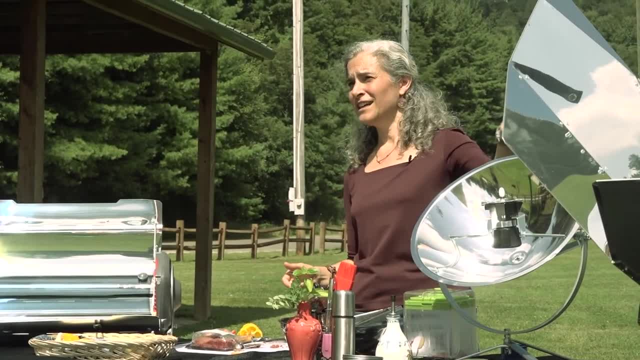 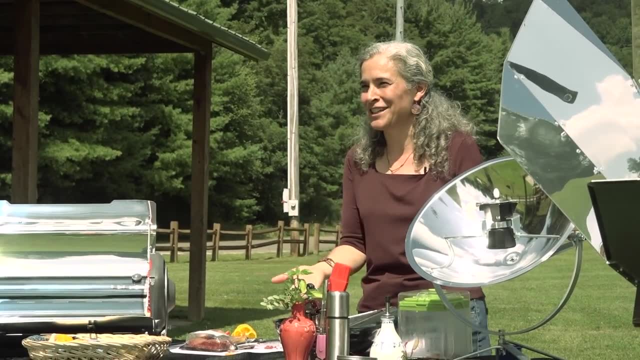 ovens have their pros and cons Pretty clearly. the Sun oven's advantage is its volume. You could put a cake in there. you could bake your Thanksgiving turkey if it was a small turkey, right. So it has this great big space, but it does lack in. 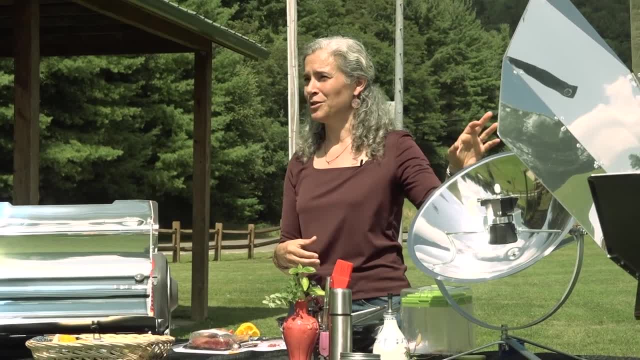 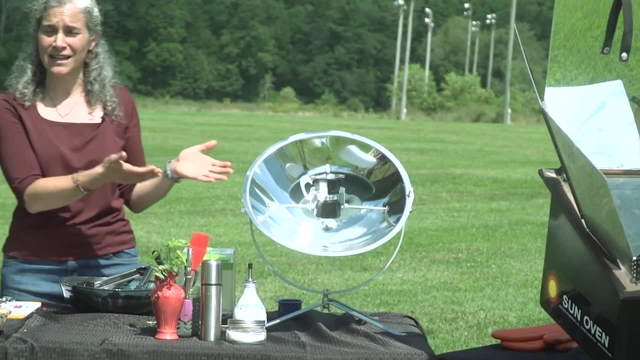 efficiency. So on a super sunny day like today, we'll probably do pretty well. But on a day that has a dapple of shade or some clouds roll in, you're pretty much immediately out of luck with that kind of technology. The evacuated tube on the other. hand, one of the biggest consequences is actually that it can get too hot on a really hot day. They're just so incredibly efficient. I've actually cooked in that one on a day that was rainy and I was stuck under a tent and it still got to just under 200 degrees. So they are. 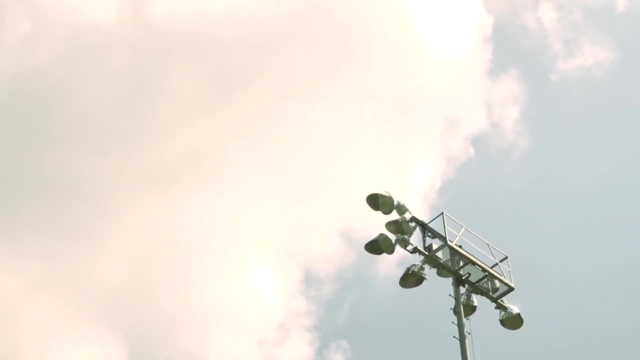 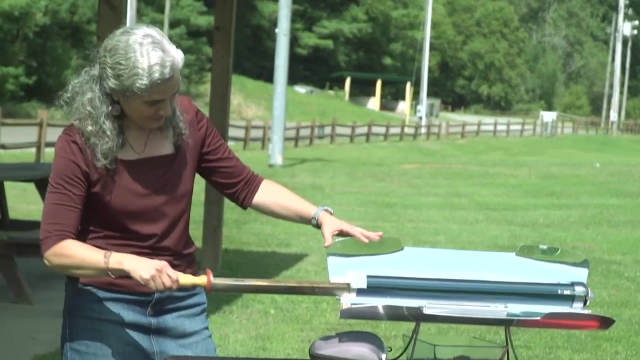 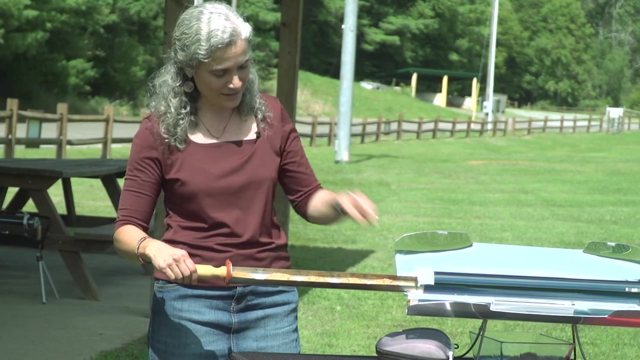 just super efficient. I'm going to pause for a moment because I smell gingersnap, So I'm going to check to see if we've burnt our cookies already. Yeah, So we see here we have this beautifully, nicely cooked gingersnap down here, One of 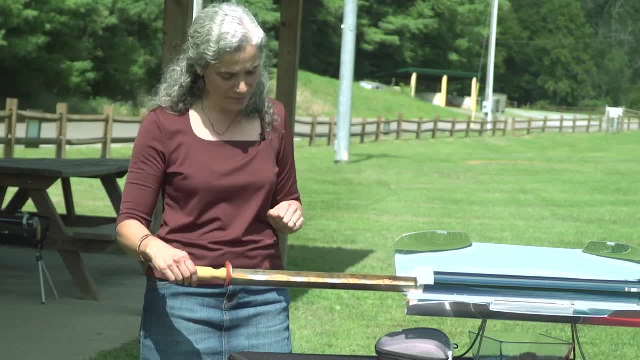 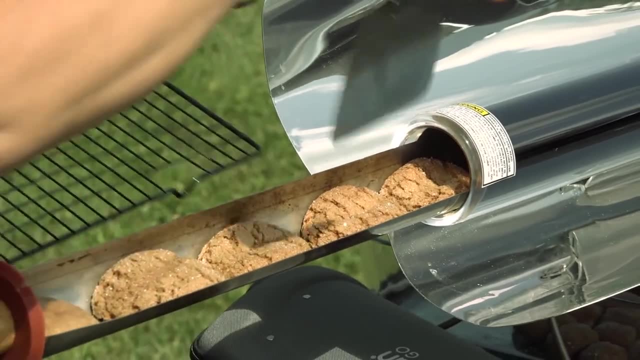 the things about evacuated tubes is they tend to get hotter in the deep part of the oven than they do here. So we see, out here we're still a bit raw, whereas down here we're pretty well cooked. Oh yeah, this smells so good. I completely wish I could. 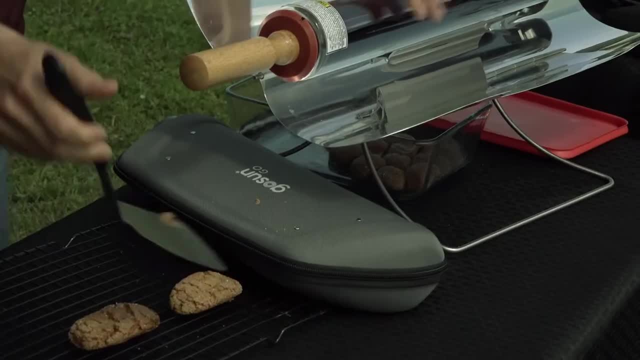 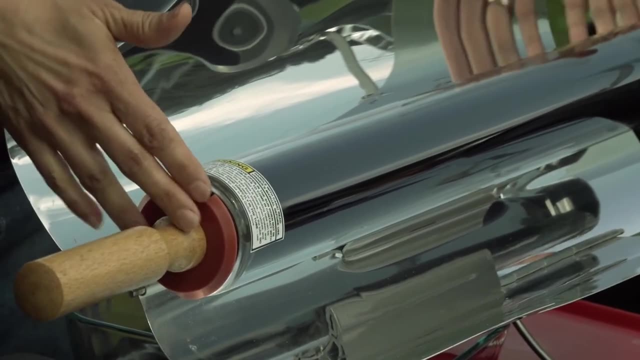 be sending these good smells out to the audience right now. Obviously hot in there, but this outside is still completely cool to the touch. So we see the the impact of that evacuation between those two layers there. So I have several evacuated tubes out here. Let's just go. 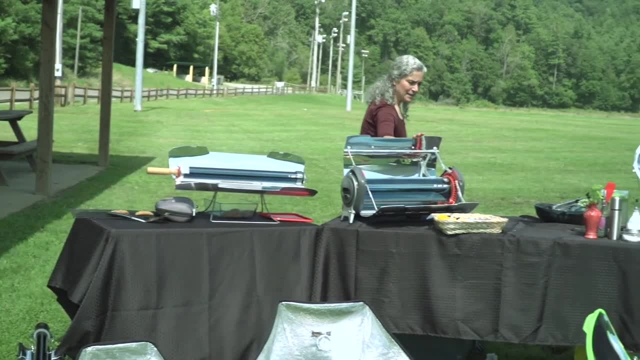 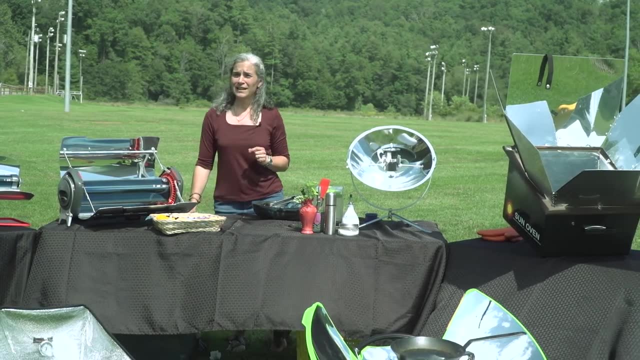 through The fusion is the latest and greatest. So let me tell you another something special about the fusion. It also is about this yellow oven on the floor, And that's that they're called hybrid ovens, And that means that they work with the. 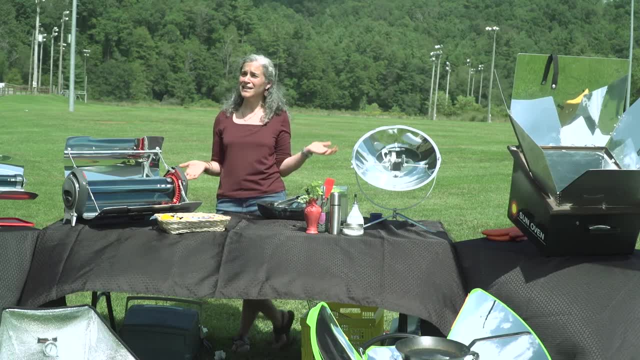 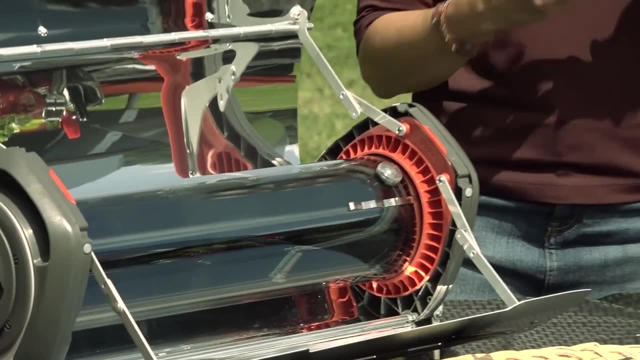 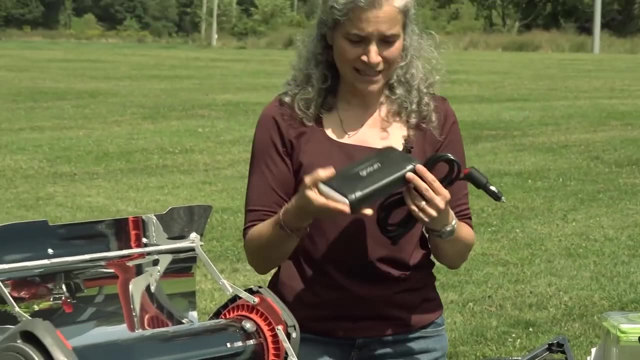 sun, Yes, but I can't tell you how many times I've been out cooking in the sun and then the really thick clouds roll in. So this also has the advantage of an electric strip. So it comes with a power cord Also, you can buy this, this solar battery that comes with it. 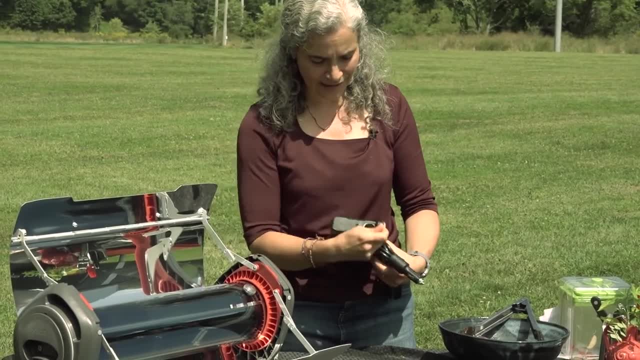 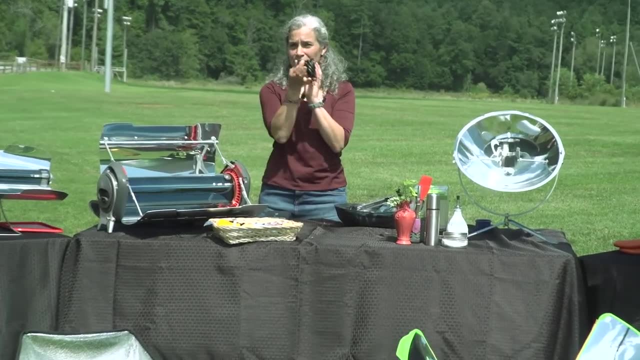 right, And so you have an output here, a 12 volt outlet, So you can use this battery or you could use your car or an RV or a boat or whatever also, And this plugs into here. And then this plug here plugs directly into the tray of the fusion, And I'll 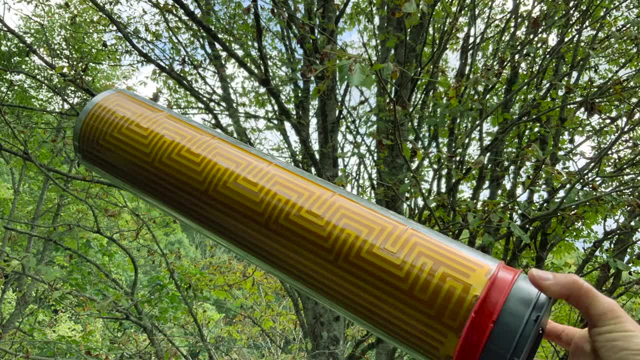 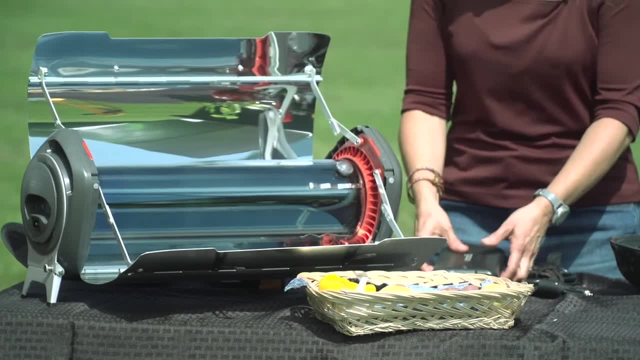 show you when I take the food out of there. on the bottom of the fusion there is an electric resistance heater, And so that allows this space to be heated even in the absence of sun. So one of the great things about the fusion also is that you could. 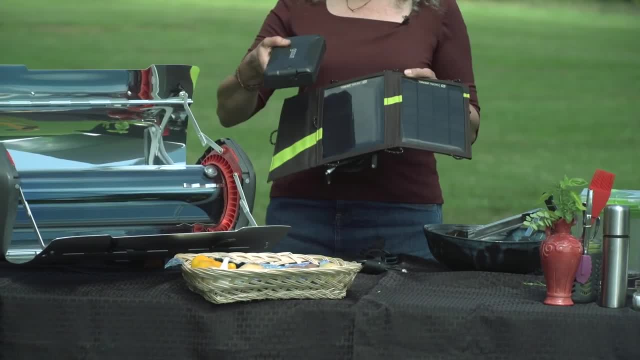 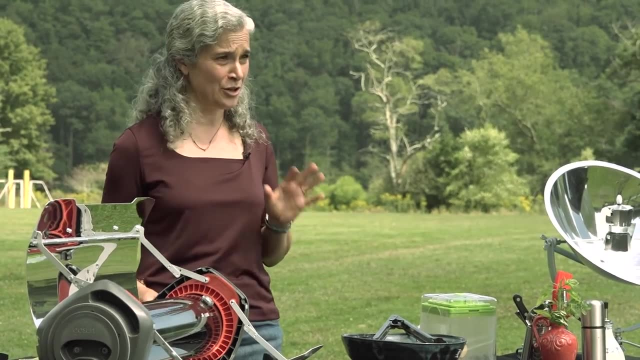 get a solar panel and charge your battery during the day with the solar energy And then when you come home at night- because usually dinnertime is not an ideal time to solar cook, which is one of the drawbacks. But now you could actually plug your. 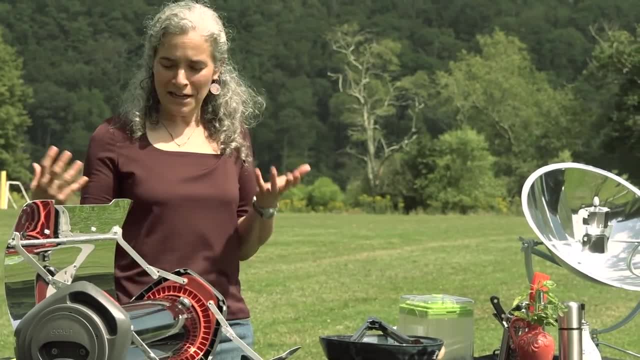 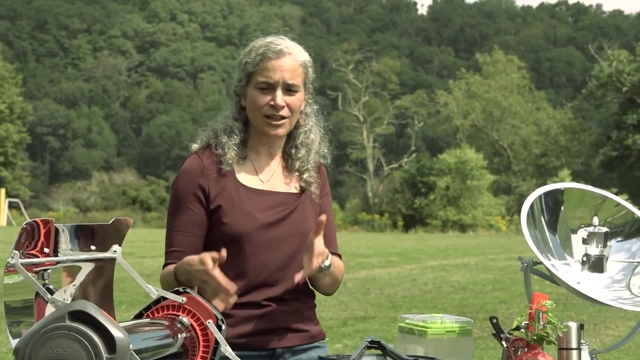 oven into this battery which had stored solar oven, solar energy for the day and then cook in the evening. So it's a brilliant solution to both trying to augment when the sun is not really bright and also be able to cook at night. So if I'm 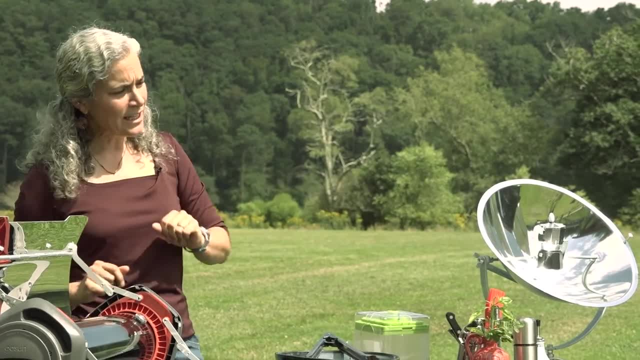 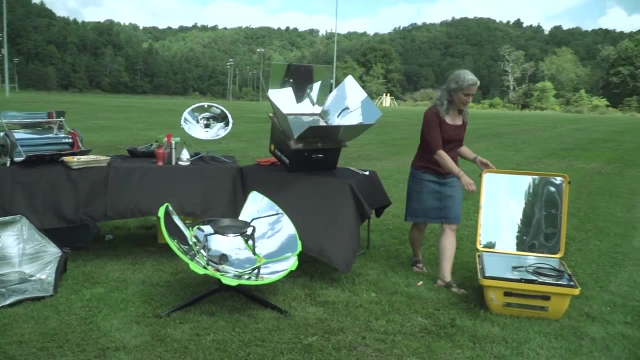 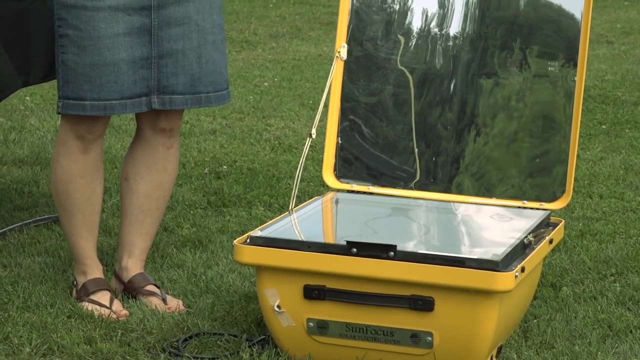 so super excited about that new technology. That yellow oven on the ground is a box oven equivalent, so this is also a hybrid oven. It also comes with a plug and there is an electric heater in here, so this is a great way to show that it's important that we are designing our 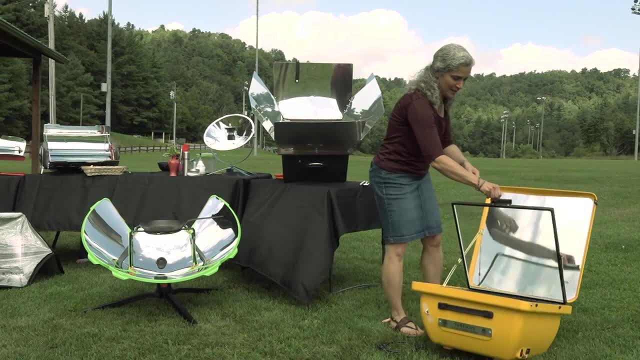 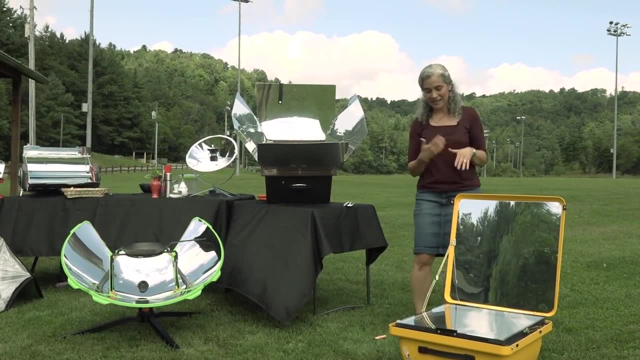 products really well. You see, as you open this oven, however, we get a significant right tipping, so it's a very difficult oven to cook on, but it did have the advantage of having this hybrid element, which I thought was really smart. So the leader in the box oven would be. 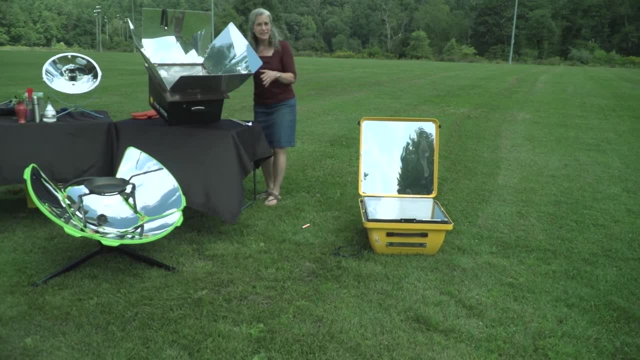 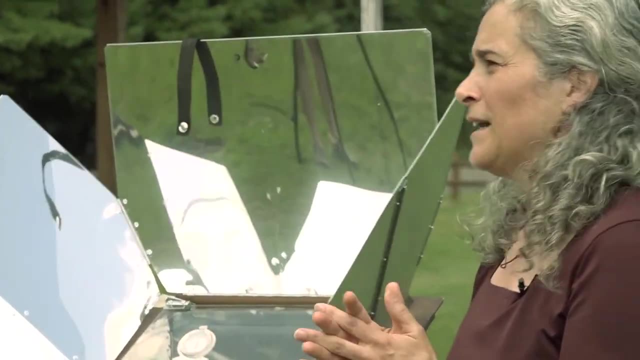 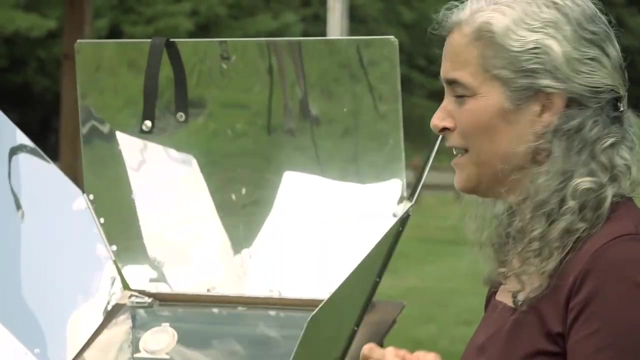 this one, which is the sun oven, and the way that it contains the thermal energy is by this. there's an inside aluminum liner. right, It's black obviously, because any of the solar radiation that comes in, you want to make sure that you have an absorbing surface there so it can heat up. 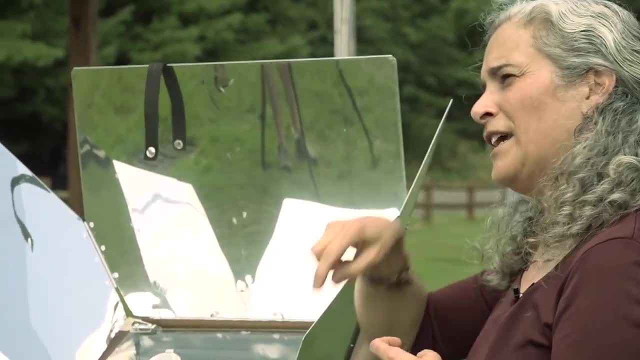 You want to make sure that you have an absorbing surface there so it can heat up. You wouldn't want a reflective surface inside the oven because that short wave radiation would come through the glass and then bounce off the surface and then, since it would stay pretty high intensity. 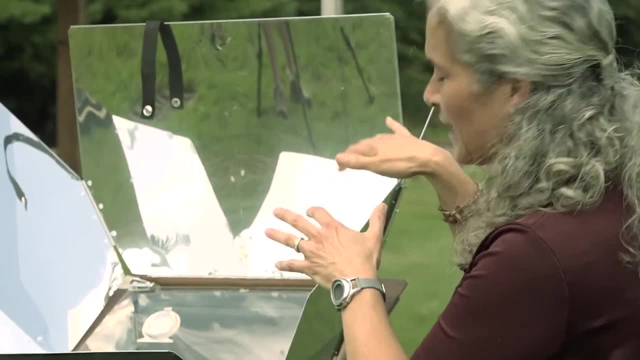 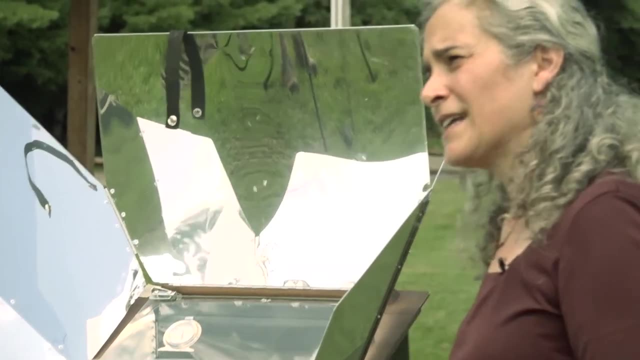 short wavelength. it would just make it right back through the glass. So you want to make sure on the inside you're putting some really dark absorbing colors. and then the outside. here is just a plastic surface on the outside of the oven and between the inside aluminum and this. 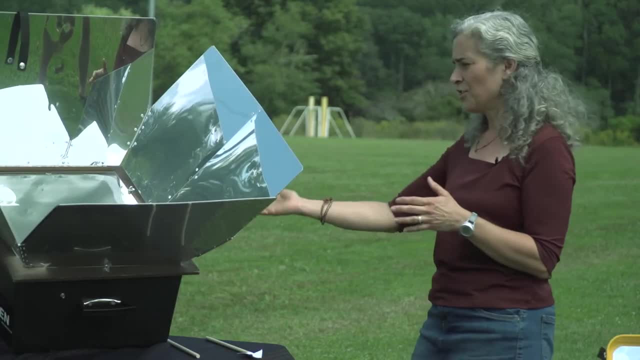 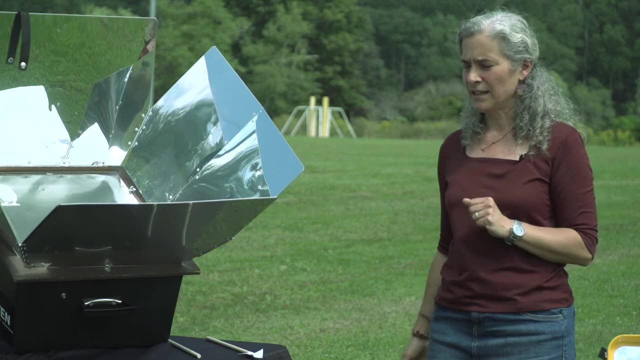 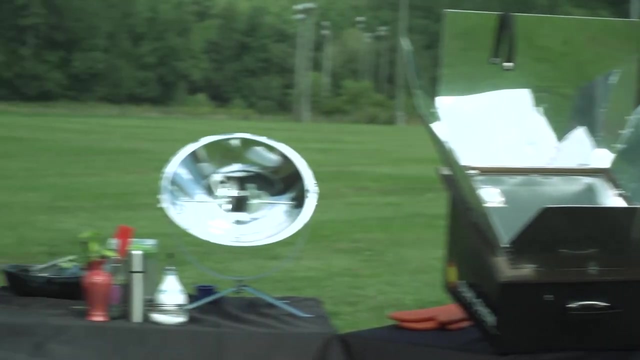 outside plastic. there's fireplace insulation, So I could cook on this all day long and I, the outside, will always be cool to the touch, So it also does a good job of keeping in that thermal energy. Okay, a couple more ovens, So many ovens. So here's another example of one of 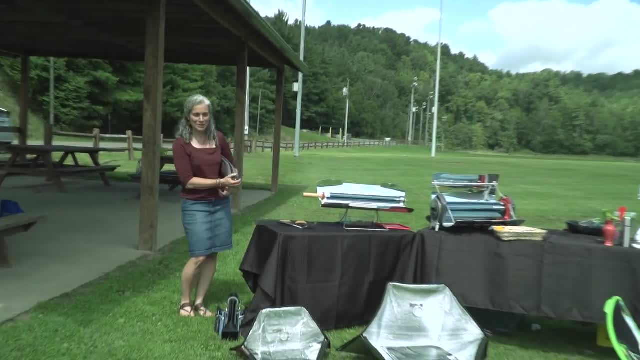 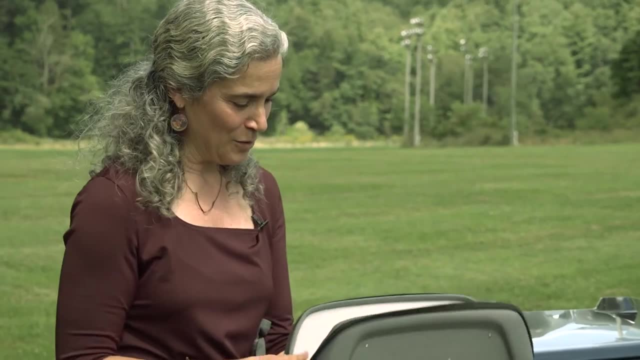 Go Suns. This is a great example of a portable oven you could bring with you to the next barbecue while everyone else is slaving over the coals. You could just open this. So this is a teeny tiny. It's great for one or two people. Here's the tray They come with, these little silicon. 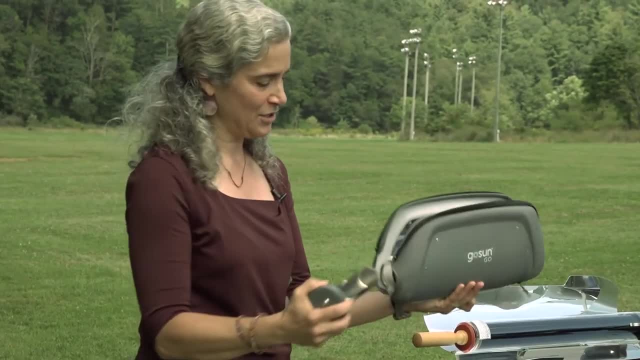 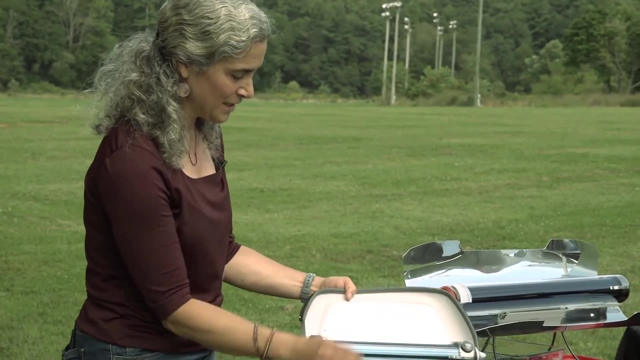 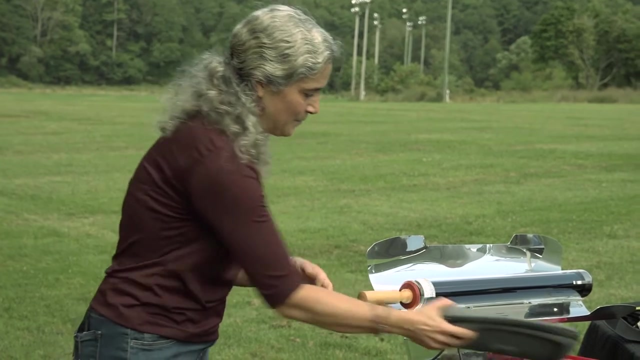 baking pans which you can choose to use, or you can just go right into the pan itself. This is actually pretty much as effective as the Sport that we're using here. So really small, It has a little lock there and, again, really fun, great introductory to solar cooking. I have another example down here. 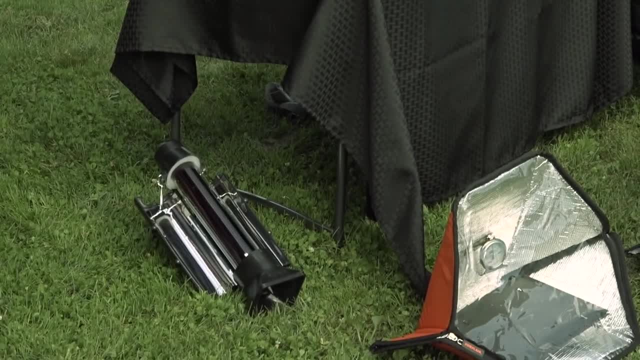 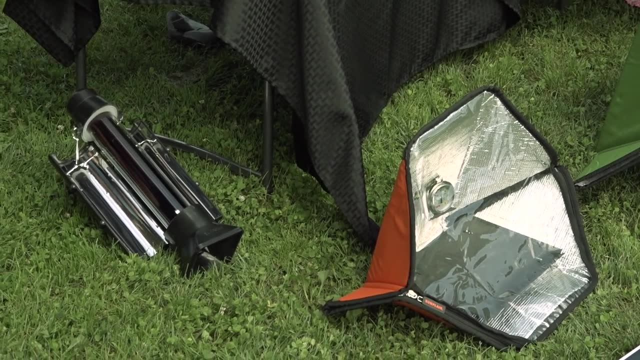 This is a solar kettle, So that's filled with water currently and it's a great way to boil water. It boils about two cups of water in about 20 minutes on a really sunny day. Again, the reflectors are just built in there. You see that this actually can then close all up, so you could. 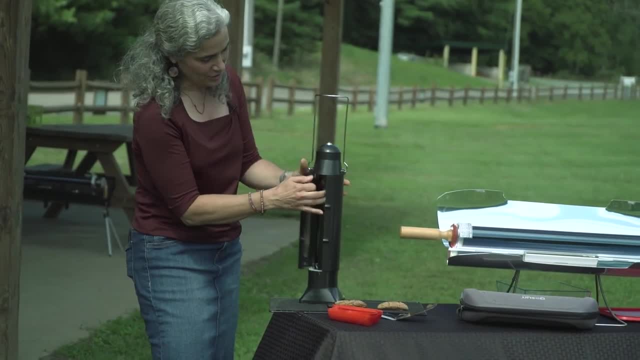 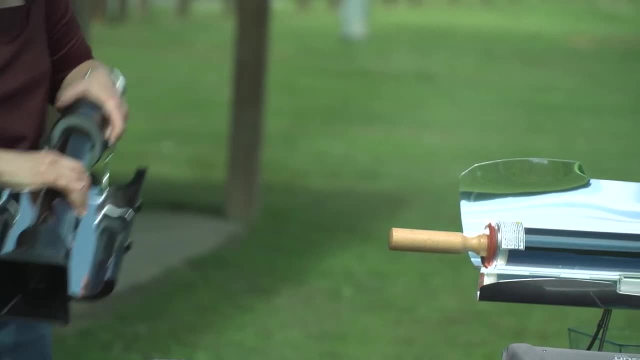 bring that with you somewhere and then, when it's time to cook, you can just open up these solar panels and then this becomes the stand and the reflectors Like that Beautiful, And there's also a little another example of an evacuated tube. that's really, really, really tiny. 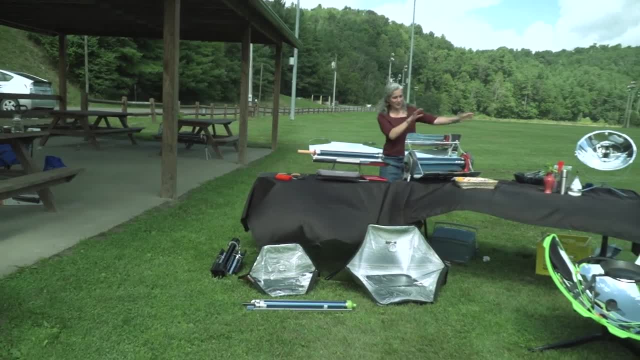 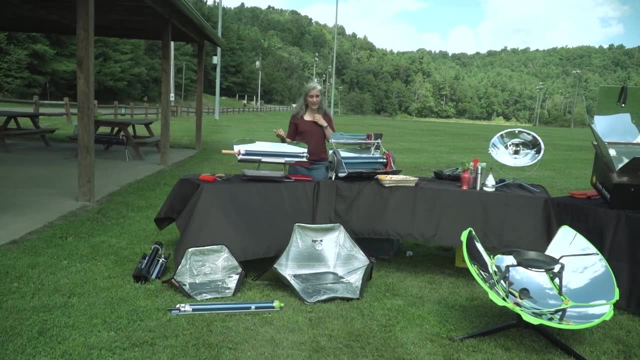 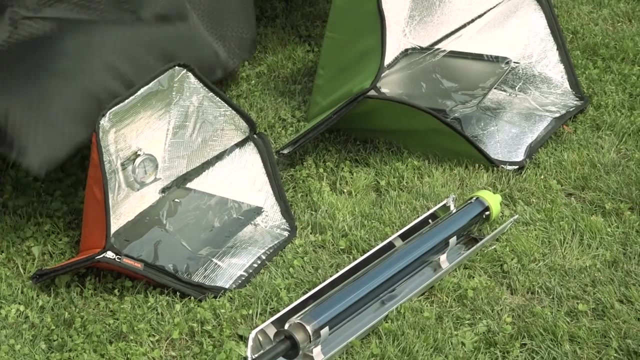 Okay, so the next category, So all these things we've been talking about, are things that replace your oven. The other category of a solar cooker is something that would replace the range or the stove top on your in your kitchen, and that's kind of what these things down here are doing. They are also, you know, concentrated. 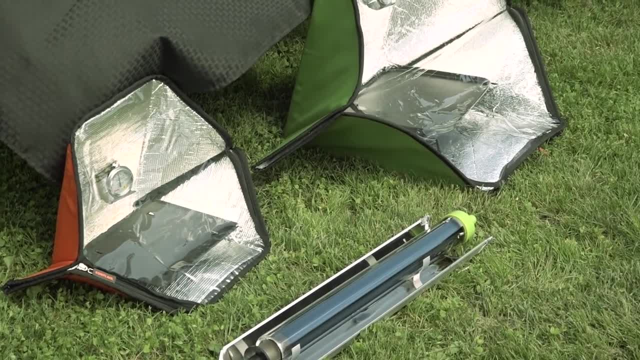 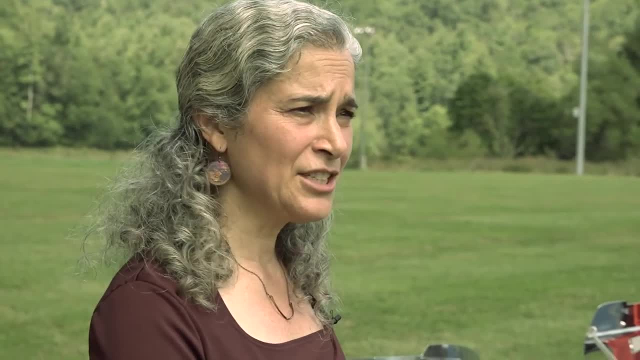 on making sure that we're grabbing a whole bunch of solar radiation, but they're not good, obviously, at blocking conduction, convection or radiation. So the advantage is that the cooking environment is very familiar. So, if you're using a stove top, if you're using a stove top, if you're using a stove top, 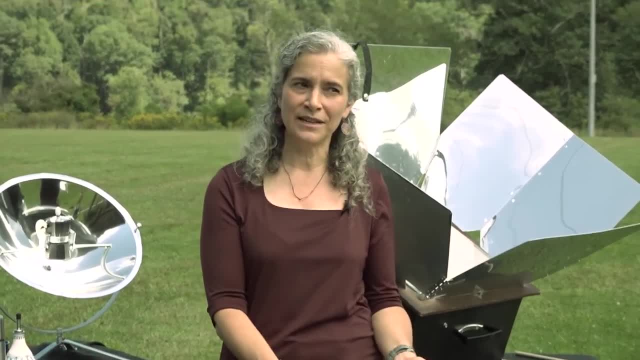 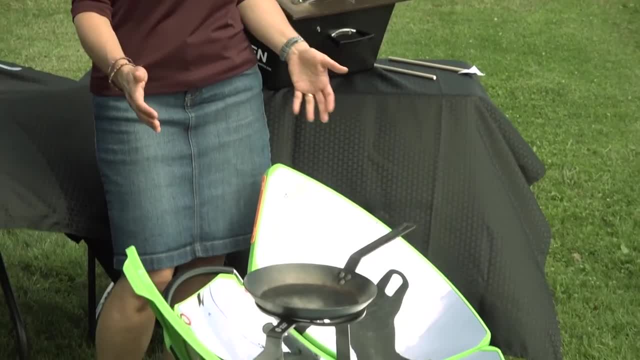 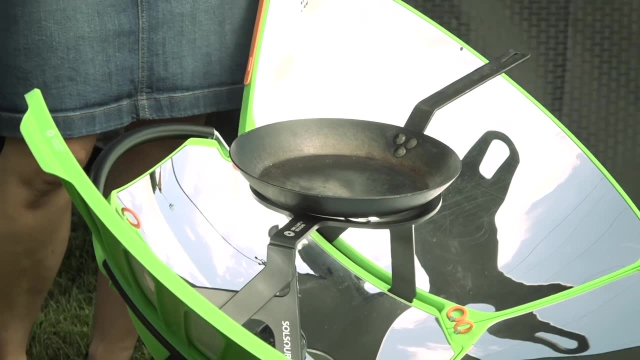 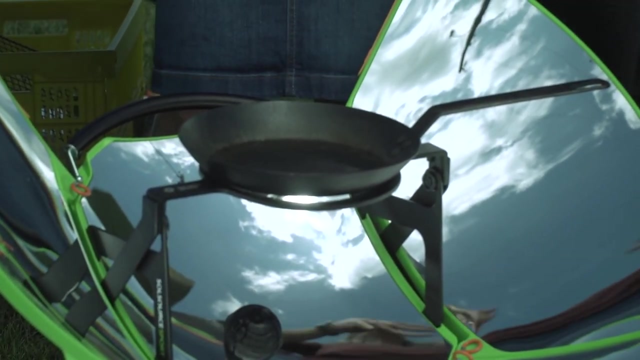 this the, the resistance burner, or the flame with the sun, And so actually in some tests they've done in third world countries, these types of cookers have the highest adoption rate, because you could genuinely kind of replace a three stone fire with this reflector and all the cookware and methodology that you. 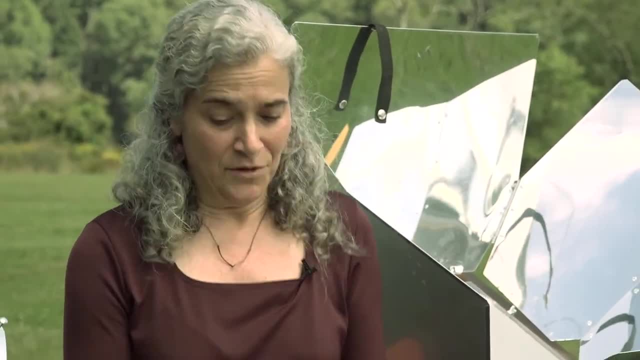 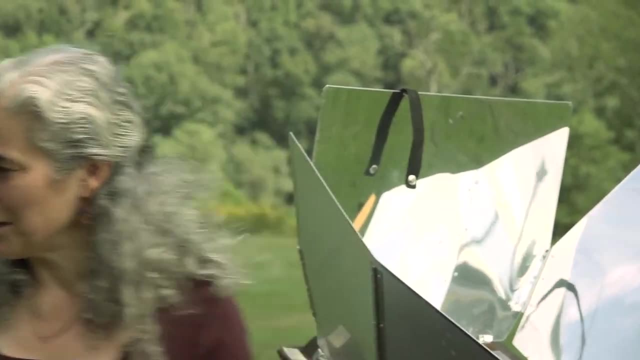 sort of were used to doing culturally remain the same. So they're not nearly as efficient, right? But so we have to consider all these other factors to make sure that we have good, to make sure we have good adoption. So we are going to test the temperature of the skillet here. I have an infrared. 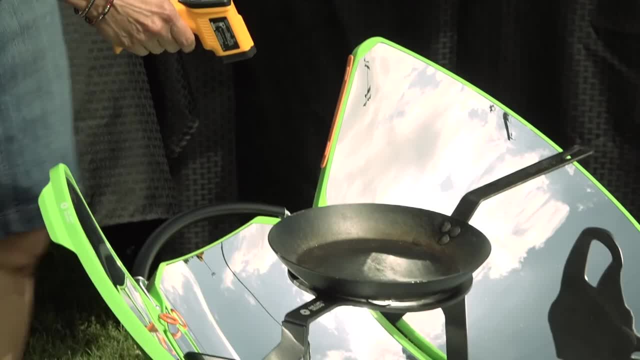 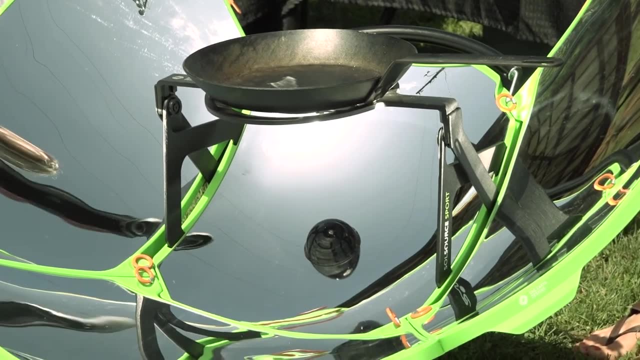 Thermometer just to see. it's been sitting out here for I don't know 20 minutes or so at the focal point. We see all these different ovens have different mechanisms for us to make sure that we are Focused properly with the angle of the Sun. this has this little. 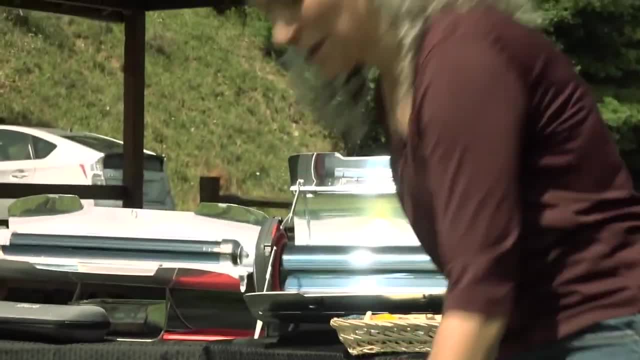 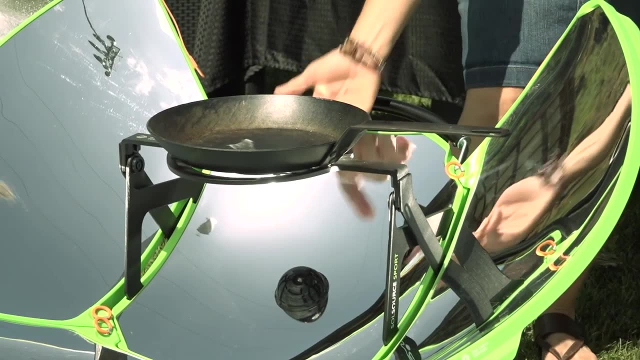 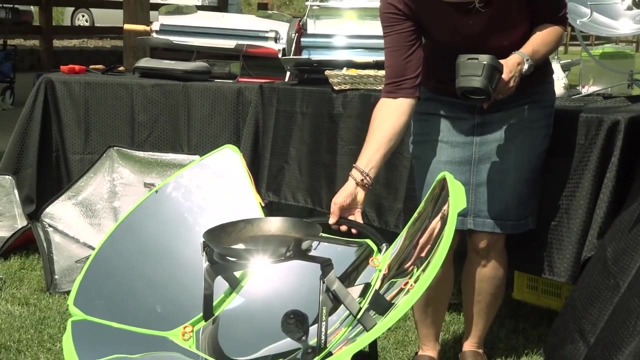 this little concave Reflector here, and so we put that right at the bottom of the that reflector, and as the radiation comes in, it actually splays A bright spot on the bottom of the pan and that shows us how we're focused. So see as we pull this out of focus. 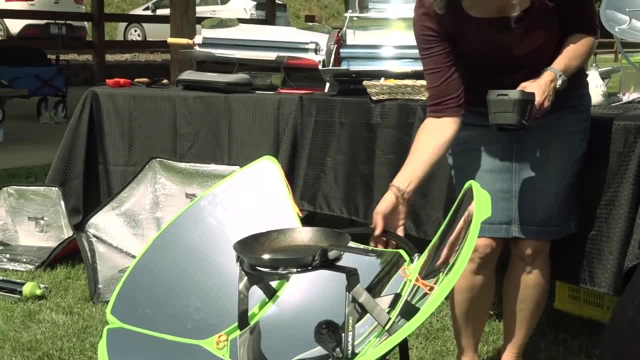 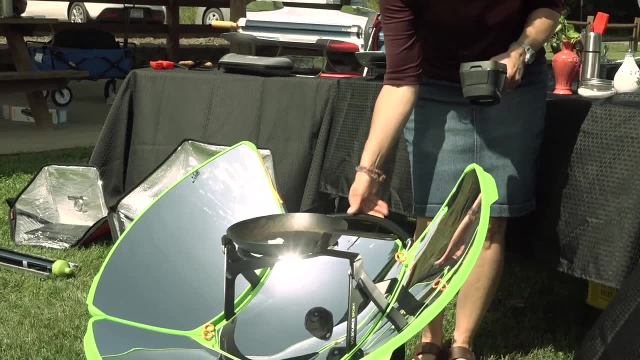 We see that little spot that we can see on this change, So it's actually like a little bit of a mirror really. that little thing acts as a mirror, So it helps us to see Where the focal point is on the bottom of this pan, so we can make sure that we get it both right and tilting. 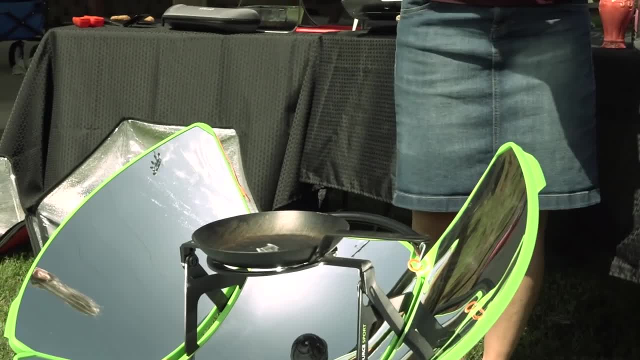 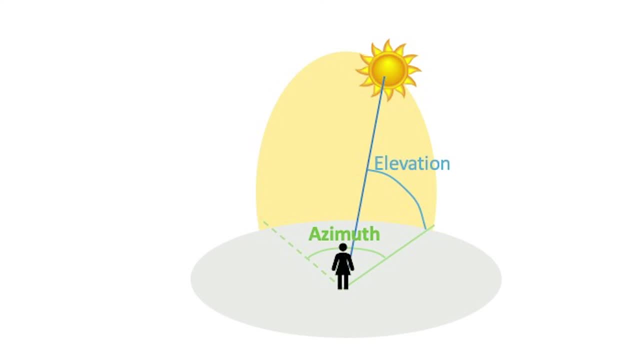 angle, And also so we want to make sure, both in elevation and azimuth, that these ovens are aligned properly. And so right there we see from that little plastic thing there that Projection of the focal point of this on the bottom of that pan looks about perfect. It's right in the middle. 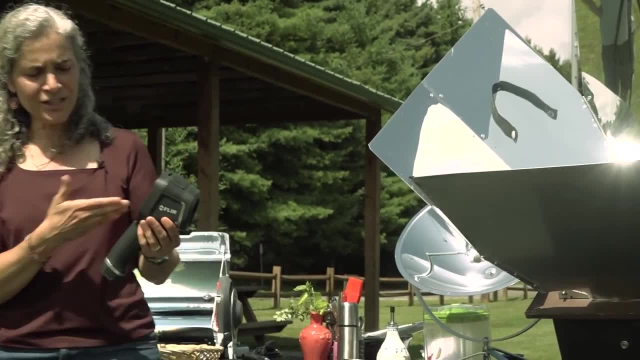 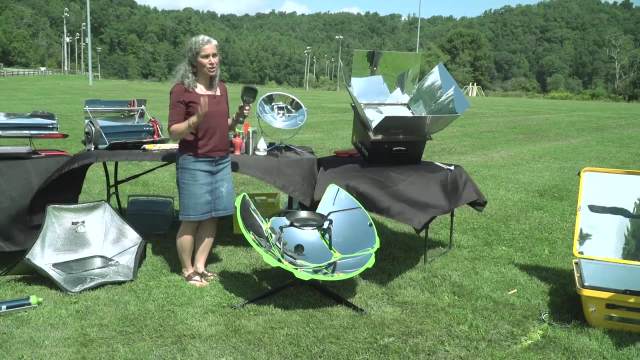 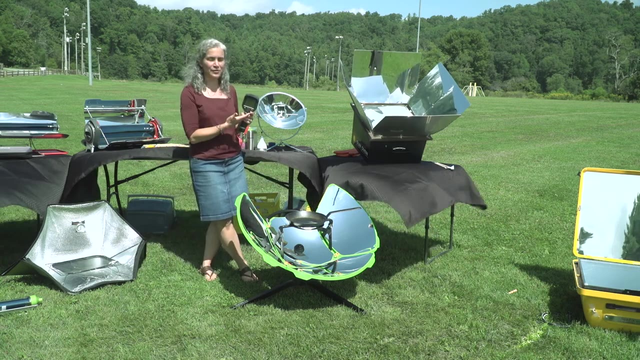 So I'm going to use this infrared thermometer. It's actually an infrared camera, So this allows us to see heat, so it allows us to see wavelengths that are a longer wavelength Than the longest wavelength that our eyes can see. So the longest wavelength we can see is in the is red, and this is called an infrared camera. 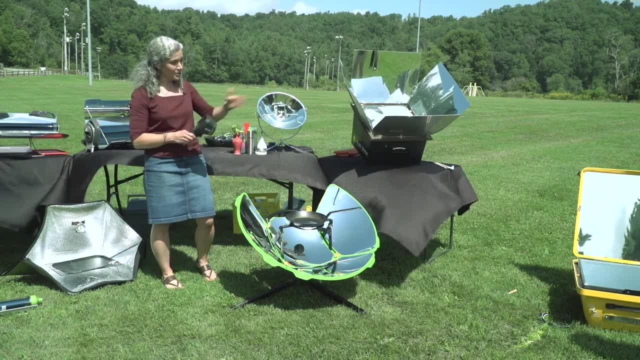 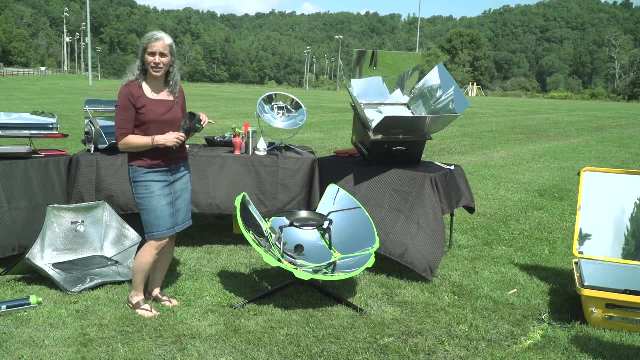 So it's these wavelengths that are longer than the red wavelength, And so it's really cool because we can see where where our heat loss is in our home. These are great diagnostic tools for energy efficiency. It really works well in our in our work here as well. 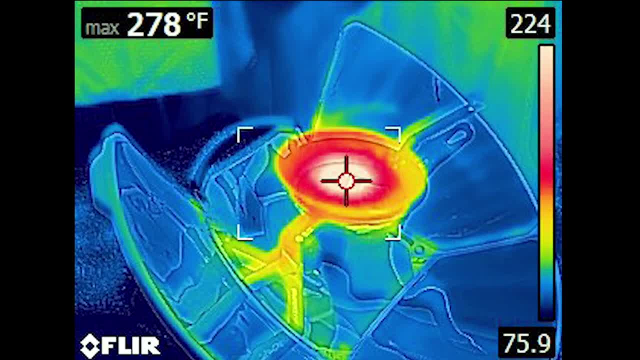 So if we take a picture there, we can see very clearly this White spot right in the middle shows that the pot is definitely The hot spot. so we see Right there in the middle and that's showing a temperature right now about 224 degrees in the middle of that pot. 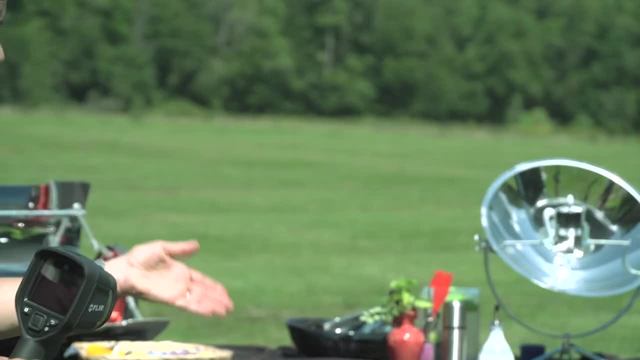 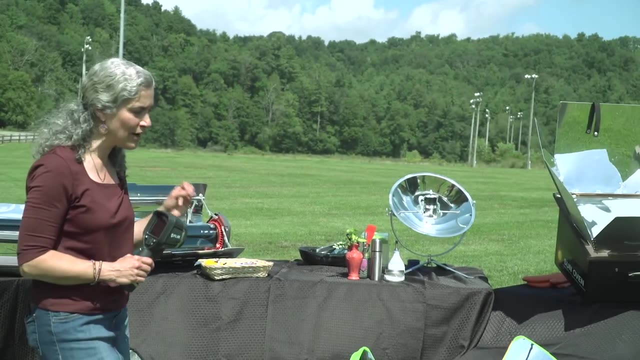 So clearly we could boil water there, but it would be hard to do anything like searing right, something You have to get to the Maillard reaction, Which is about 380 degrees. that browning we get on fish or on Caramelization on vegetables occurs only when we get to these higher temperatures. 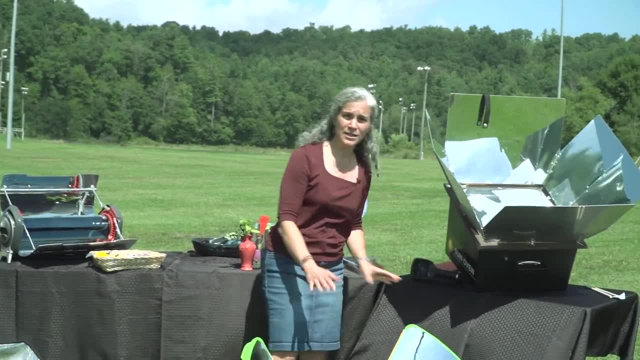 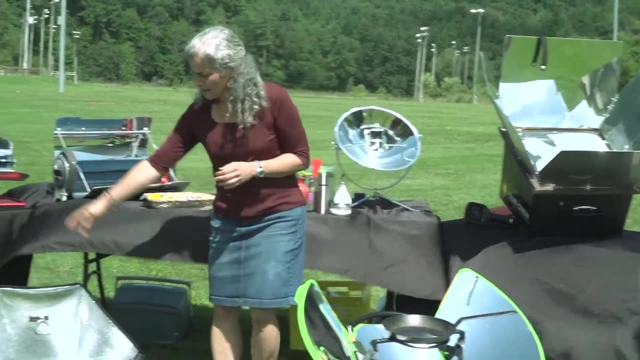 So I have struggled to get these reflectors up to temperatures to accomplish that, but certainly if I had a pot there and left It out long enough, I could see that I could could boil. These are also Reflectors. they're intended to reflect the radiation onto these. 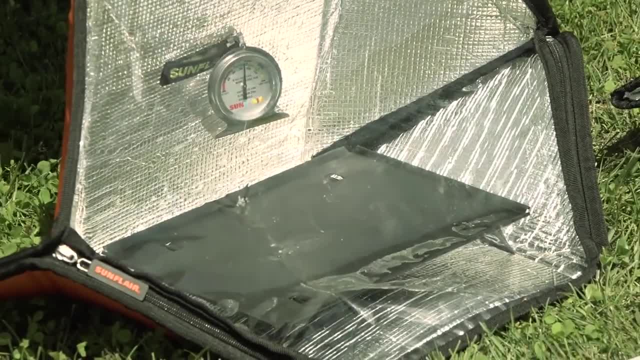 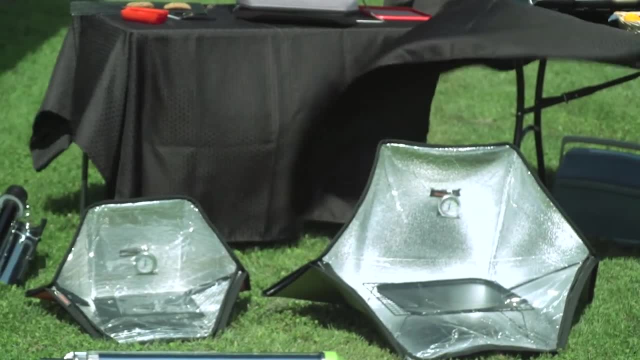 Aluminum absorbers that are up on these trays Obviously the least efficient of what we're talking about here. I have definitely cooked quesadillas in here, So we get hot enough to melt cheese. You can make s'mores all day long. It's enough to melt the chocolate and make the marshmallow nice and mushy. 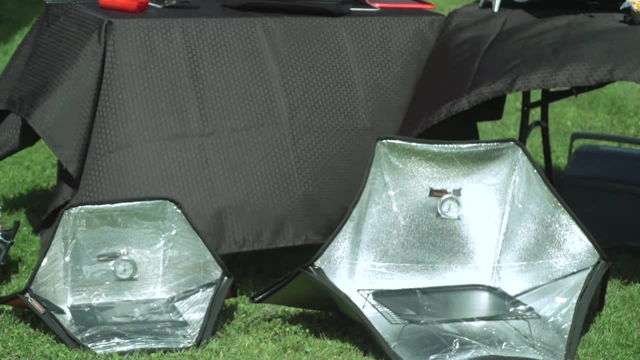 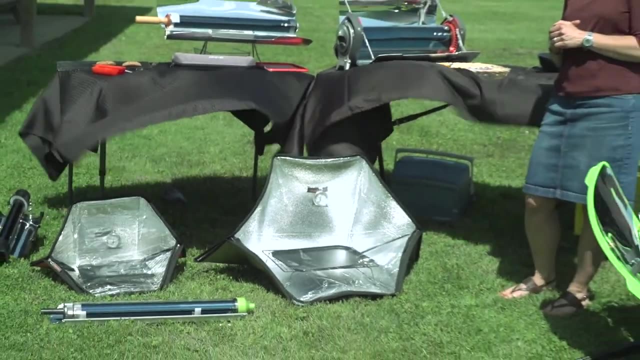 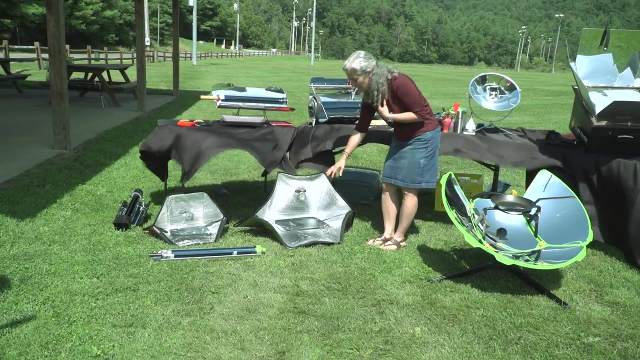 But, but trying to cook other things Becomes a challenge. there are- I've actually done- some pasta and kind of boiled pasta in there. boiling probably is an aggressive term, But I got the water- pasta water- hot enough to cook it. It took about an hour to cook a single serving of pasta. but yeah, so they actually have this. all that this. 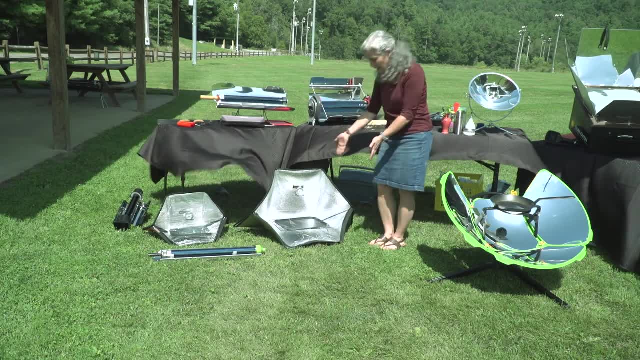 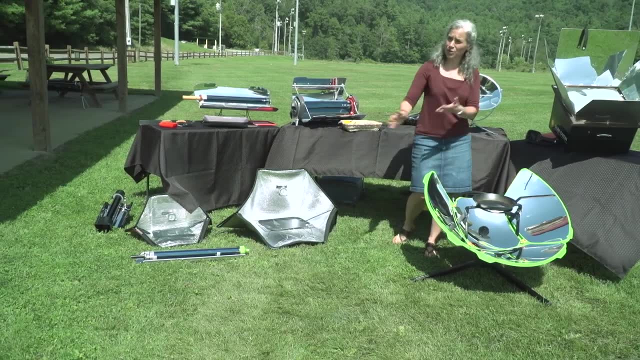 Surrounding sort of shade here is trying to do is to block convection right right now. So they- This is what a problem here is- I think what we're gaining by radiation we're losing by convection and those kind of try to Surround it to avoid that. I smell the ginger snaps again. 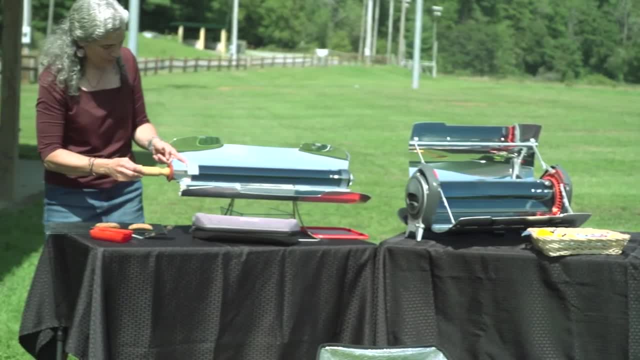 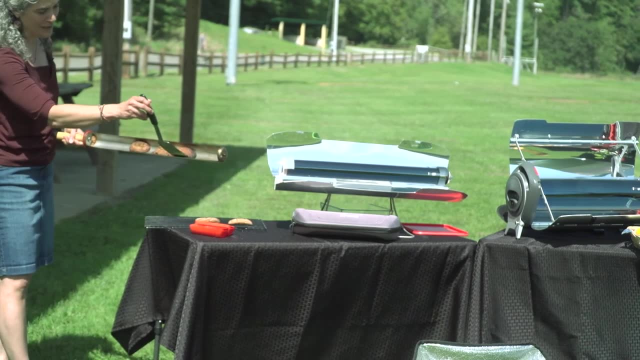 So let's hop over here and see how this goes. some sport is doing. Oh, yes, Potentially we have waited a little bit too long for batch number two of our ginger snap. So we definitely see we have accomplished our caramelization We spoke of earlier in this oven. This oven is just incredibly efficient. 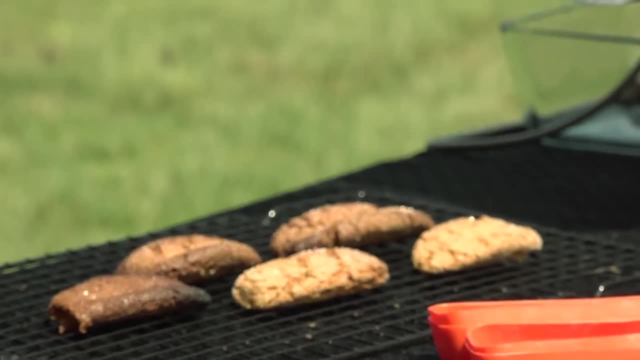 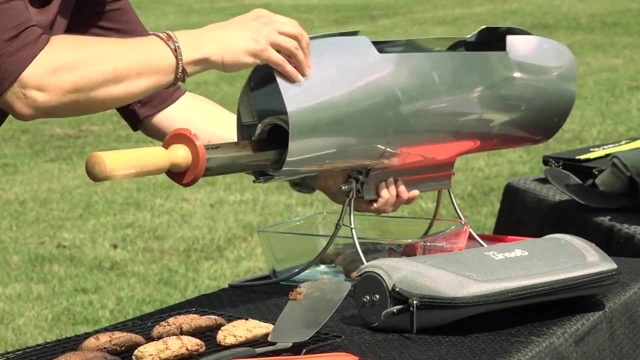 So those are our ginger snaps that we can enjoy later, and we definitely see the steam coming out of there. So I'm just gonna take this now out of the Sun. We're gonna close it up and allow it to cool down. So we see that our burgers appear to be definitely brown. 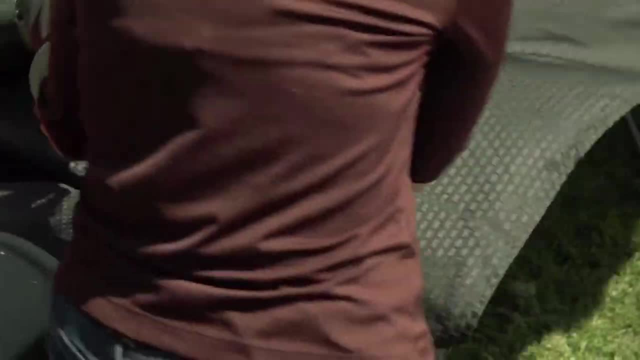 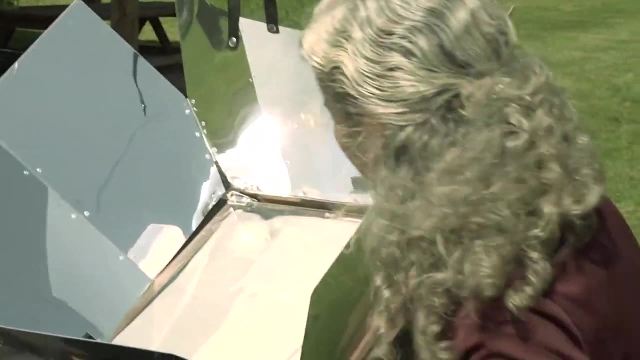 We see a little bit of sizzle going on down there, just like the other evacuated to see. one of the drawbacks of, Well, a lot of these ovens is that they really retain a lot of the moisture right. They have to be sealed up so that we're not losing a tremendous amount of thermal energy. 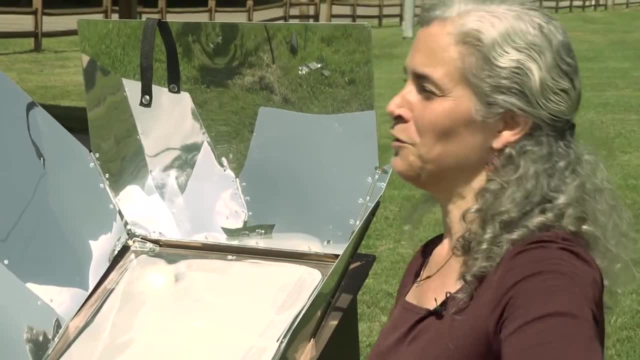 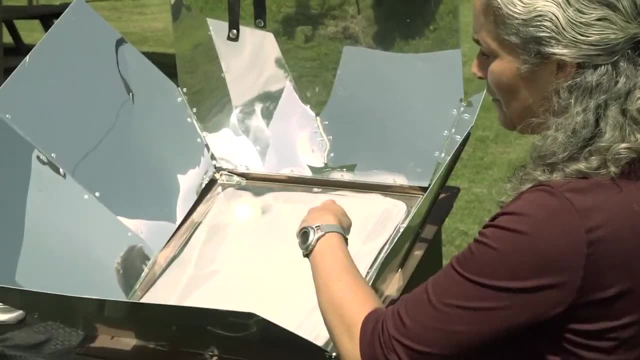 But as we cook food right, the water that's in the food vaporizes and becomes steam, and then what happens is that the steam recondenses on the Surfaces. so we see, in the case of a box oven that really degrades the performance because now we have this sort of 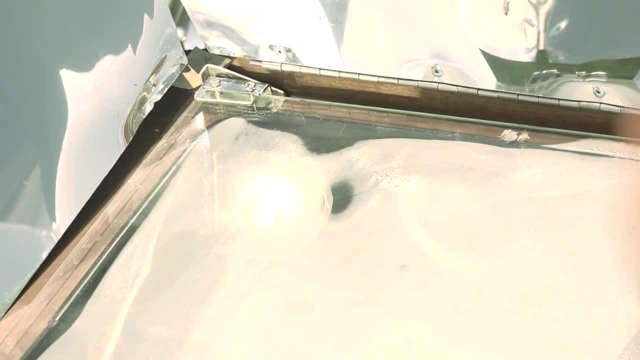 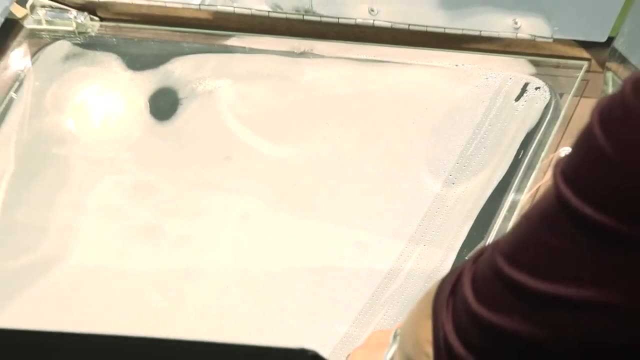 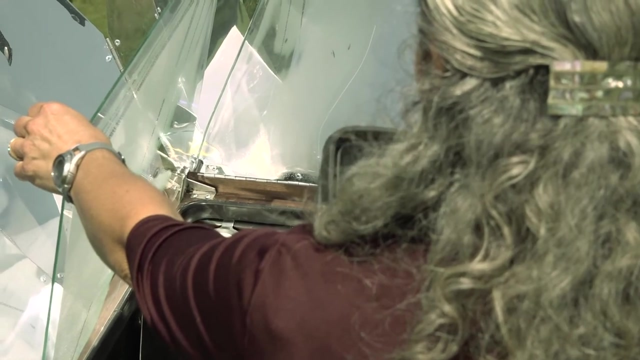 Film of steam or condensed water there That is now blocking some of the incoming radiation. So I'm going to open this and allow some of that steam to escape and also check the temperature while I open it. Okay, so also, I see the burgers are looking like they're coming along pretty well. 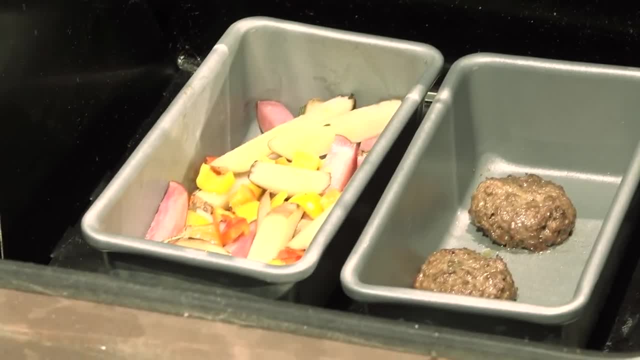 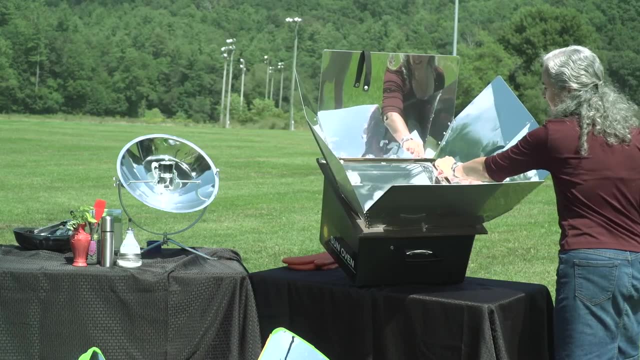 We can even see a little bit of sizzle there on the edge of the burger, like we did on the other one, And then the potatoes are are on their way to cooking. One of the things that's curious to me about these ovens, these box ovens, is they open from the top right and 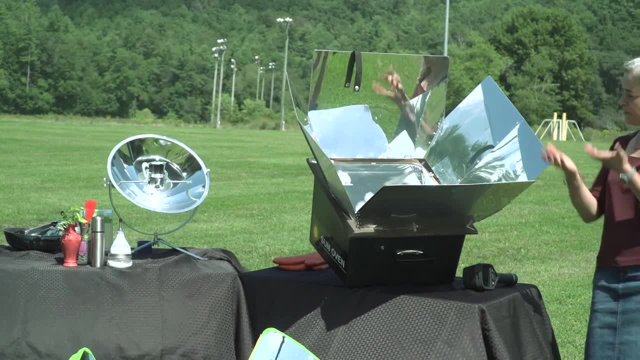 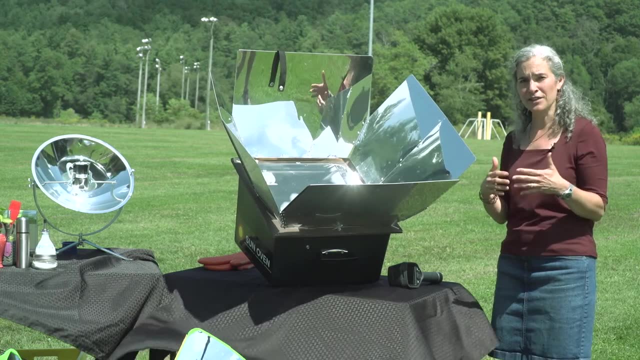 I mean heat rises or colder air sinks, right, And so what ends up happening when you open these ovens particularly, is that you get a huge belch of the thermal energy and it takes A while to recover that. because this is at the top. I'd love a box oven manufacturer to come up with a door on the side. 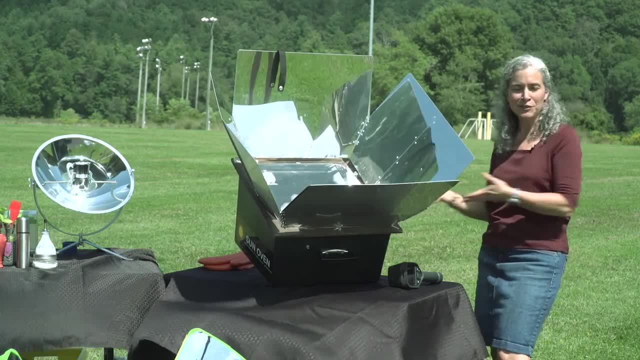 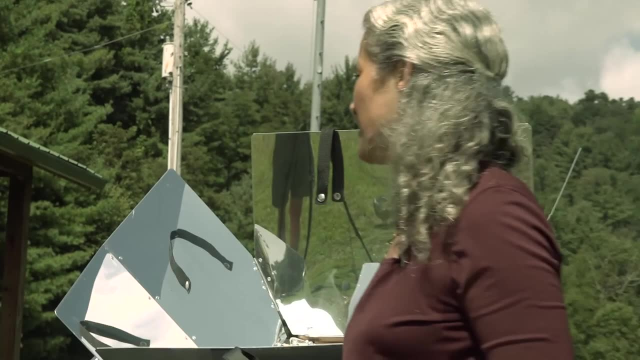 Like you have in your oven at home, so you can open it and replace food without really sort of losing this enormous amount of energy. the evacuated tubes right. you open them from the side, and so that does definitely help to not Drop the temperature so significantly as you check on the food. 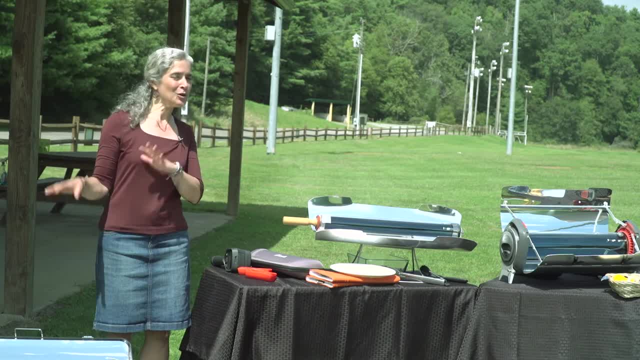 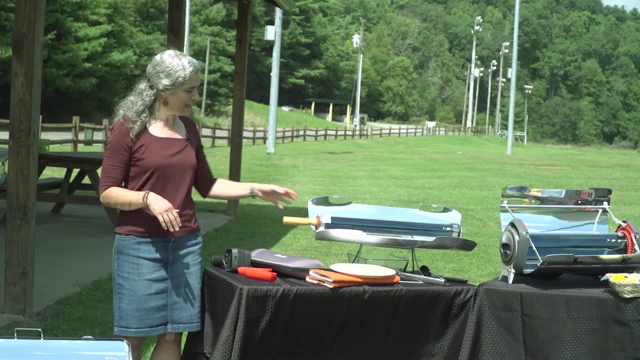 All right. so I think we've waited a little while. we keep having sort of the clouds rolling in. so We've had a little bit more of a weight than typical, But I think we're going to go ahead and pull this food out of the oven. I just wanted to make a note quickly that you know. 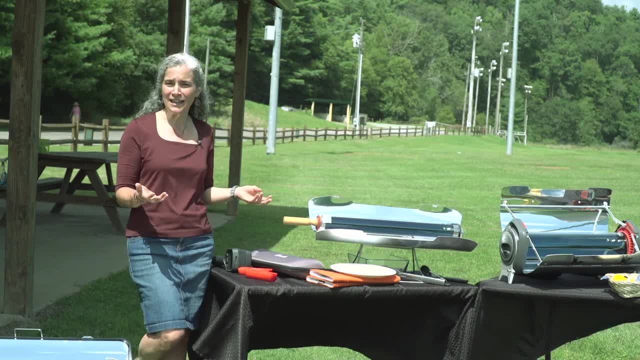 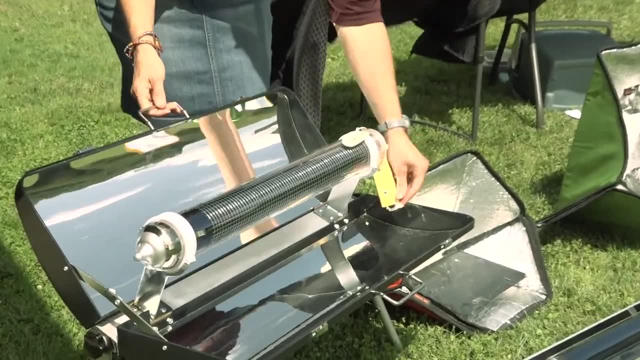 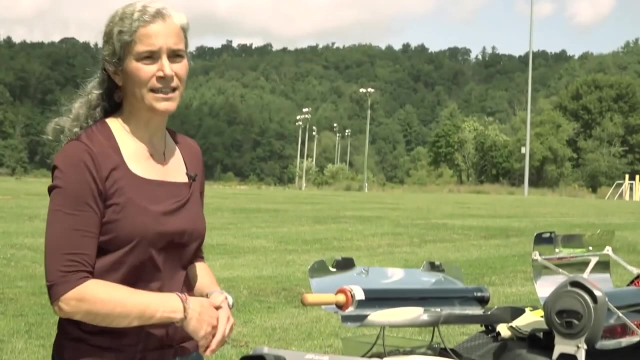 We've talked about the effectiveness of evacuated tubes, but I have learned that not all evacuated tubes are created equal. So, for example, this solar oven I was really attracted to right because it has a really nice hard outer shell Which is protective. but I know from outreach events that I can do cookies in. 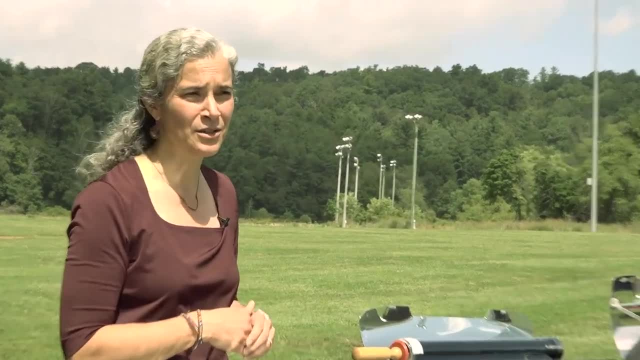 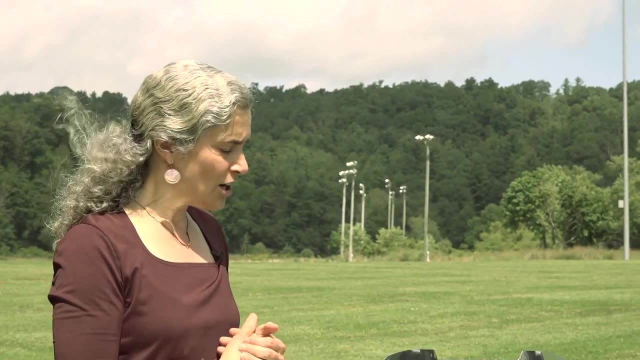 This one about four batches of cookies to one batch in there. So, whether it's the difference in the coating or evacuation, or reflectors Maybe aren't parabolic enough or what have you just want to be cautious about that- that there's a lot of Factors that have to come together for all this technology to work as well as it does. 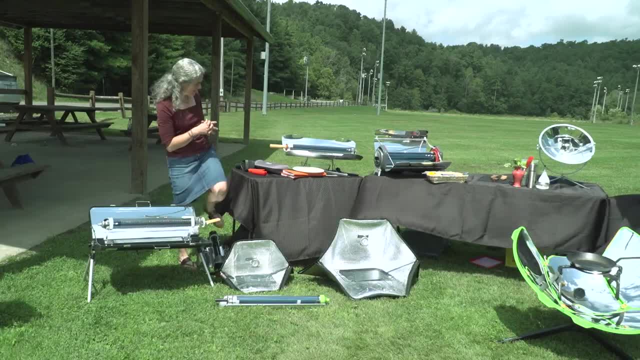 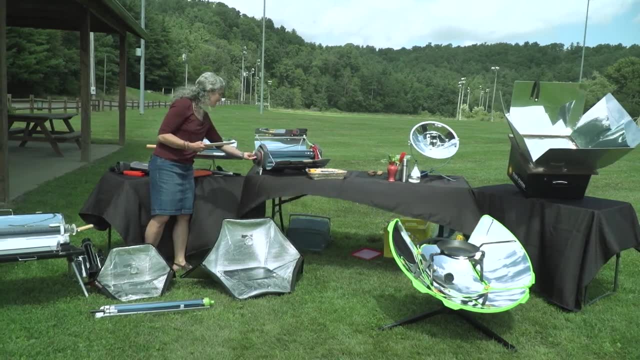 All right. so let's go ahead and open the oven and see if we can do some eating, which, again, I really would love to share, but I'm just going to have to do it all myself On a day that we weren't struggling with the sun so much. 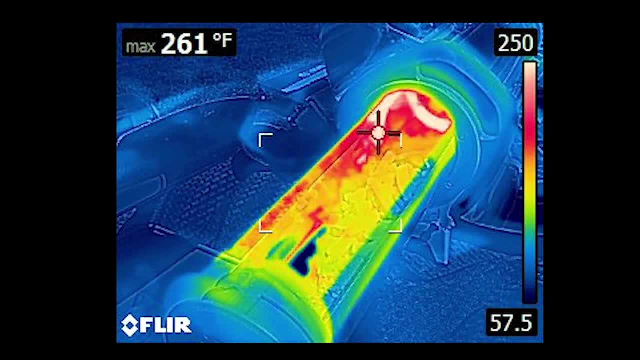 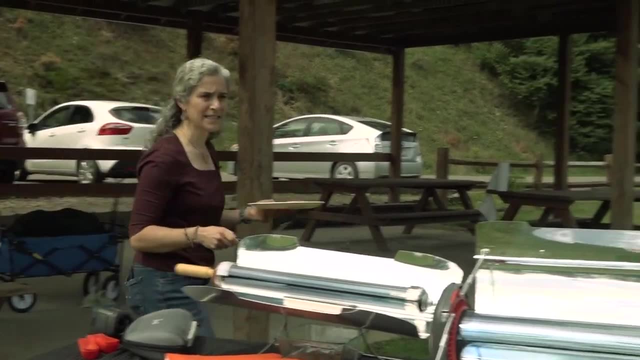 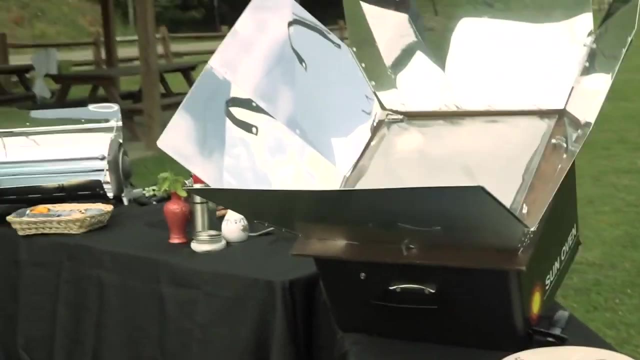 We definitely would have a little bit more browning on those. I've cooked them in here before and gotten a nice, nice browning, And then let's head over to our box oven and see how That's doing And open this up. Might be nice to take a infrared image so we're showing about. 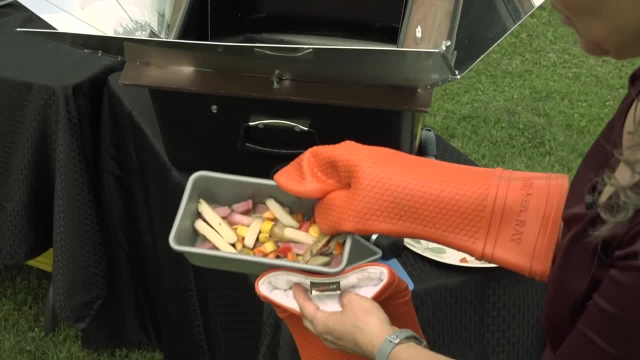 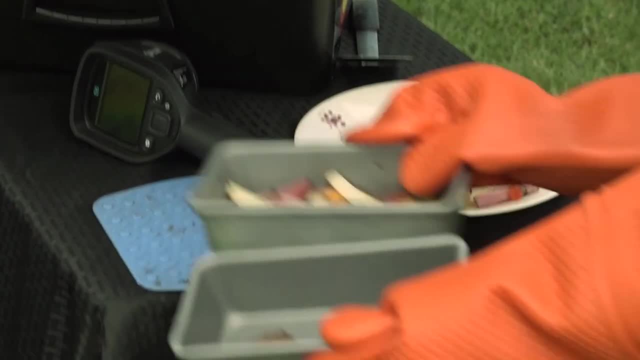 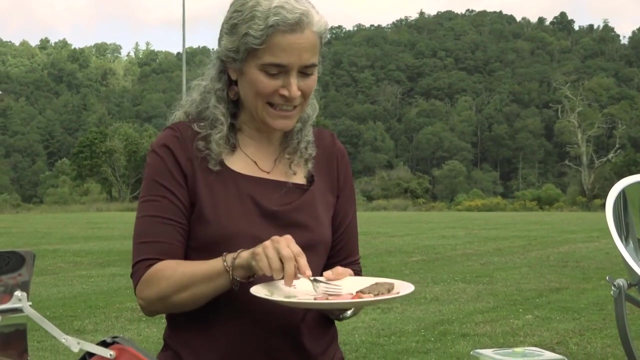 238 degrees inside this oven right now. the vegetables also, and the burgers seem to have done quite well. There we go. let's take a taste and see what it's like, Right? so again, I wish you were here to share this with me, But I'm going to take a little taste here and see how, how everything went. 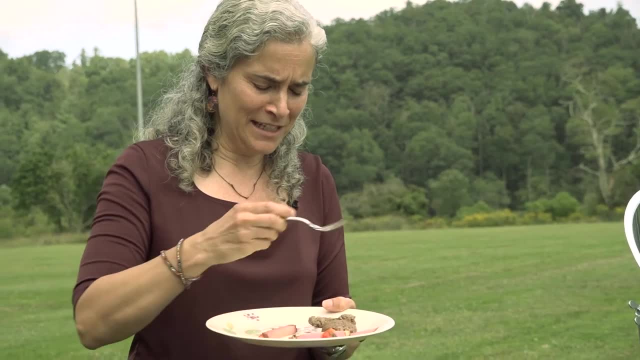 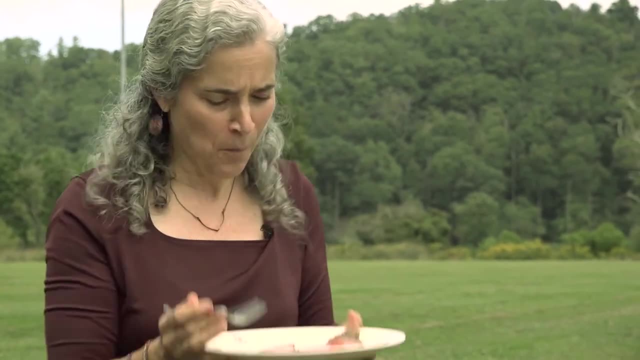 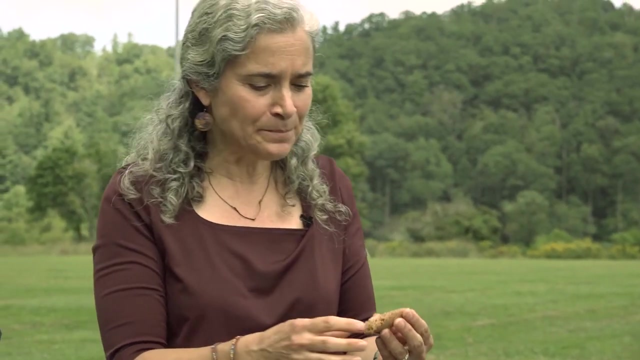 Peppers are delicious. a little bit of this burger. We see that it did cook all the way through. we have no more pink. Really, really good you. I would super encourage you to try these new burgers. Don't necessarily need to be all vegetarian. Any part of our food system that we can shift as a help. and then, lastly so one note about evacuated tubes is you have 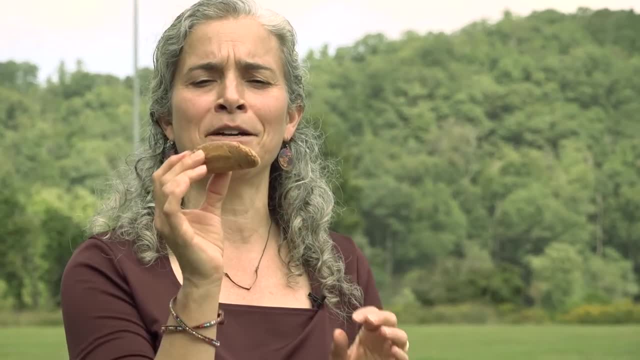 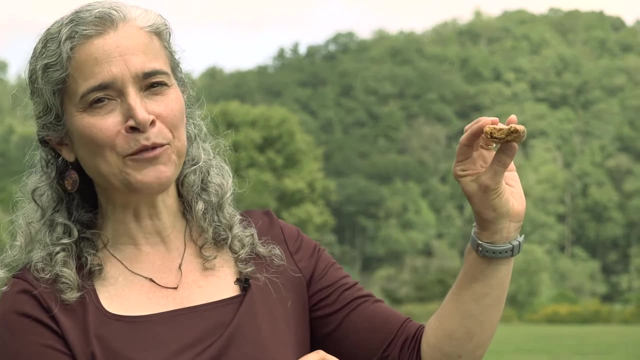 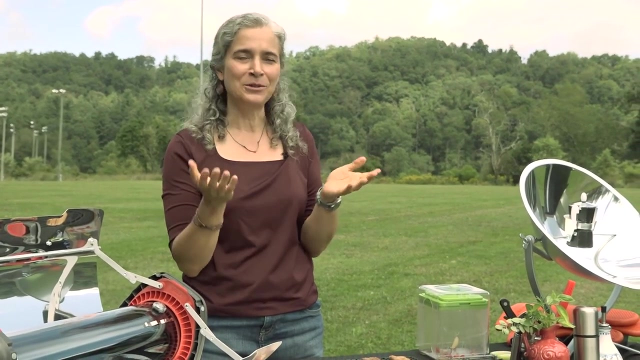 To be okay with your cookies being a little curved, which is okay, because you know what they fit in your mouth a lot better, right? Hmm, really really good, cooked perfectly. so Thank you for joining me. Get out there and cook and I'm happy to answer any questions You might have. have a great day. 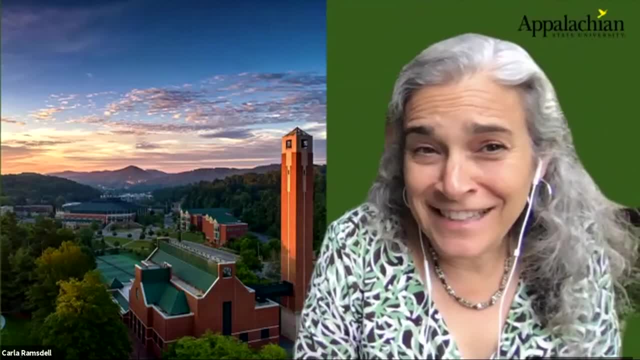 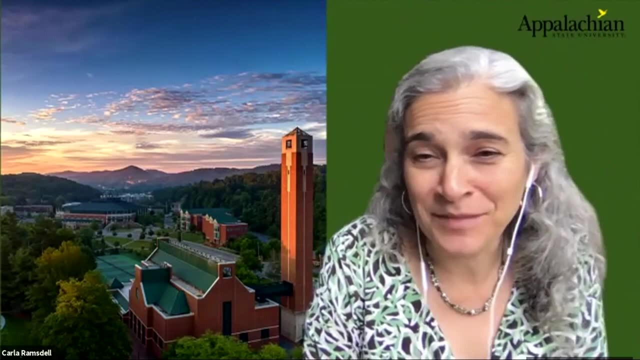 All righty, So that was it. it was a pretty nice day. We did get some clouds here and there, but we were able to do some cooking anyway. so, Yeah, just happy to answer any Questions. welcome to those of you who joined a little late. 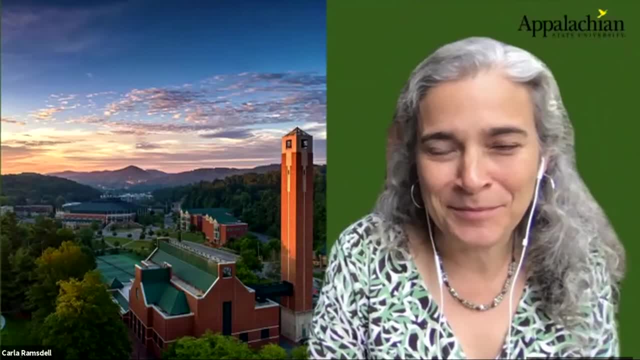 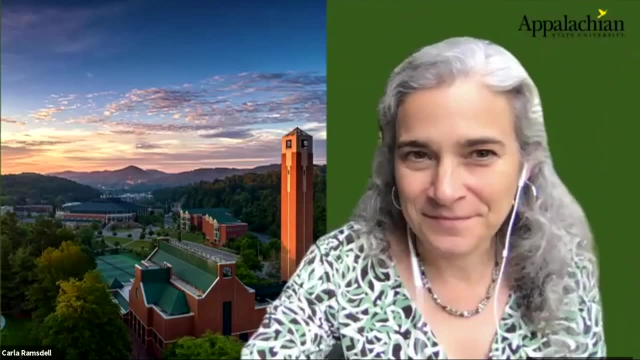 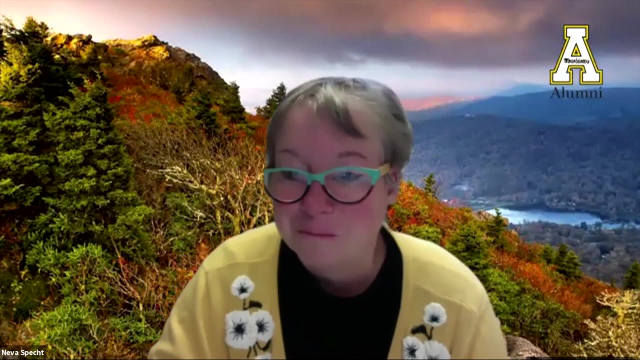 I hope you got enough of it to to see what was happening there, But we were trying all kinds of different solar cooking technologies. It's great. so, yeah, let's open it up. if they have a question, go ahead and ask. I wondered about the approximate cost of those various ovens and 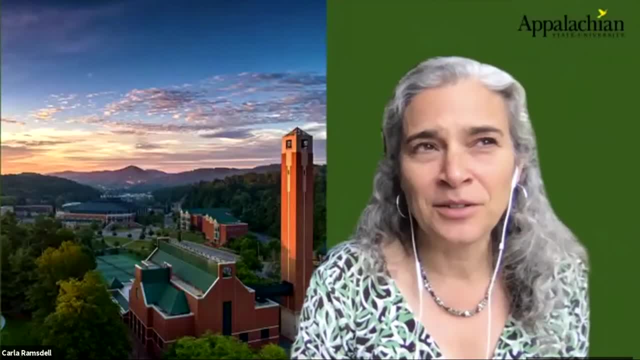 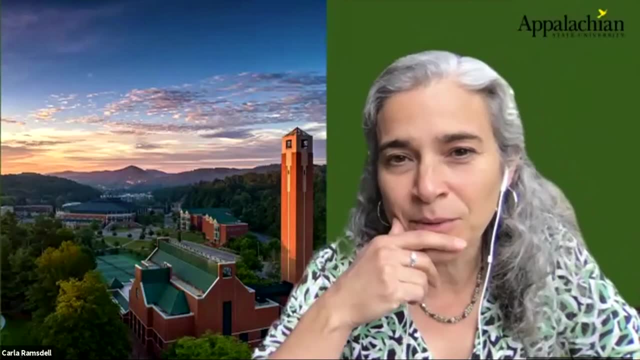 ones, yeah, so I'm not totally up to date on the cost. the the what we did is the What we did- the cookies in the ghost on sport- is probably the most popular one. It's really effective. It's in the two hundred and thirty dollar range, if I remember correctly. I think that's about the same as the box oven, the Sun oven about that same price. the fusion is the latest one out. if you get that without the Battery backup, you know it does come with the electric strip still, but not the battery. I think it's in the $400 range, somewhere like that. 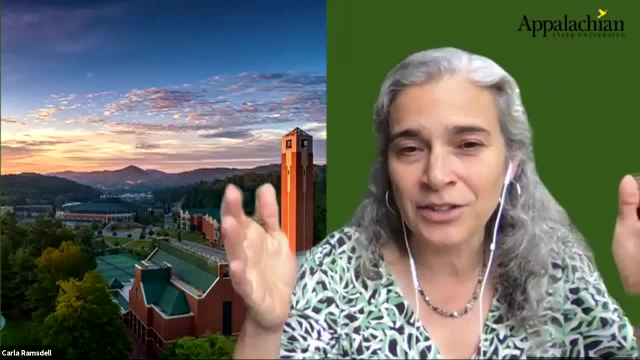 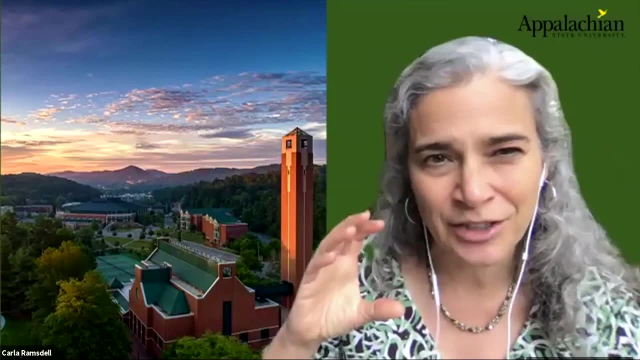 They actually made an even bigger oven at one point that they call the ghost on grill, Which I've tried also it's. it's really slow on heat up. once it gets heated It's great, But has a big chunk of aluminum in it where the tray is and that thermal mass really slows down. 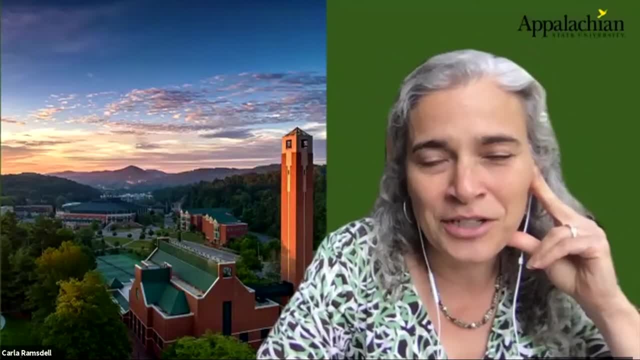 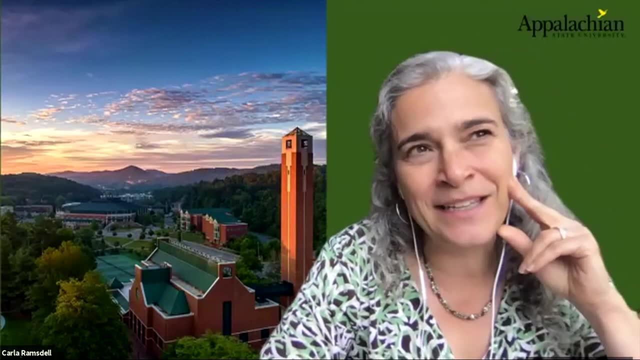 It's, it's heat up because that specific heat is huge. That thing was eight hundred dollars, So they they definitely kind of missed their price point there. They intended that to be an oven you'd keep on your porch all the time to replace your grill. But and then those solar flares. That was on there were on the ground. Those are sub $100, But you know they just don't work that great. So I don't know. the little handheld one, the go, Sun zippered, the go, It's like low hundreds, a hundred hundred twenty. if you sign up for the a lot of those sites though. 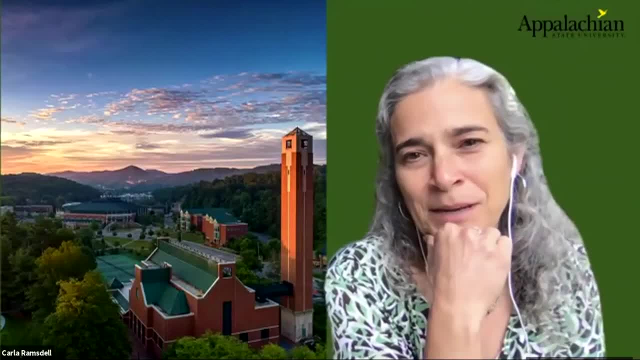 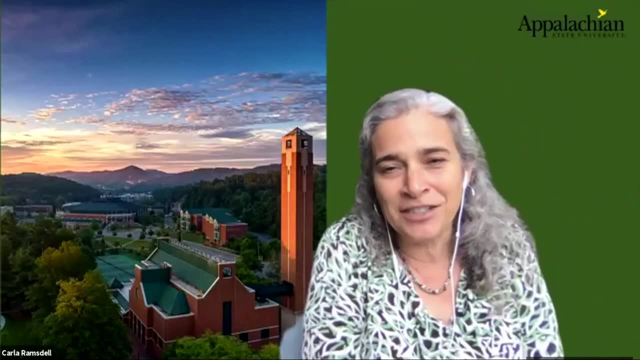 They will tell you when they do these refurbished Specials from time to time, and so a lot of them that we've purchased, we just wait till they do the refurbished. They work the same, maybe just not in the original packaging or something. So I think we got that little zippered one for $80. 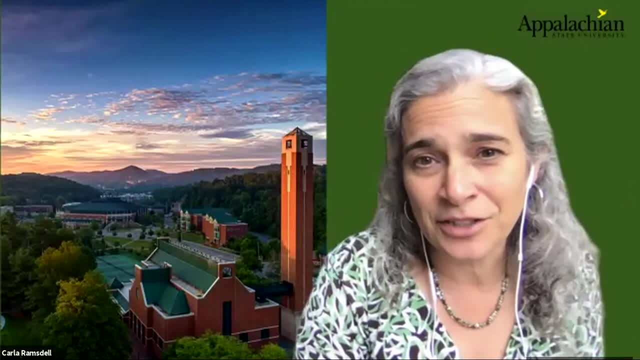 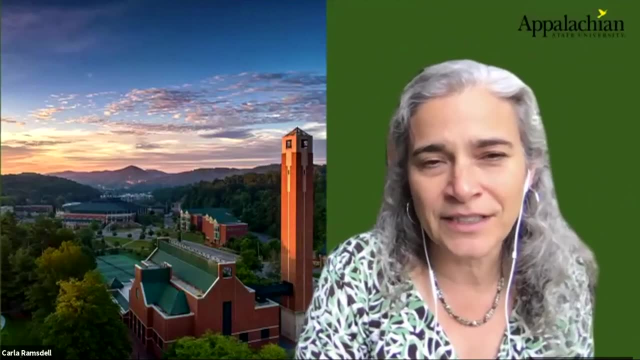 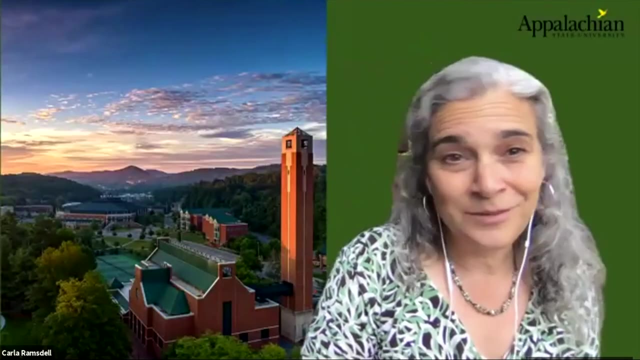 And it really does work as well. It's just not as big, so it's not good for any more than two people. would be a struggle. But you know, and all those companies are pretty actively involved in Distributing this technology and third-world countries as well. So you know, I mean, I love cooking with this, It's fun. 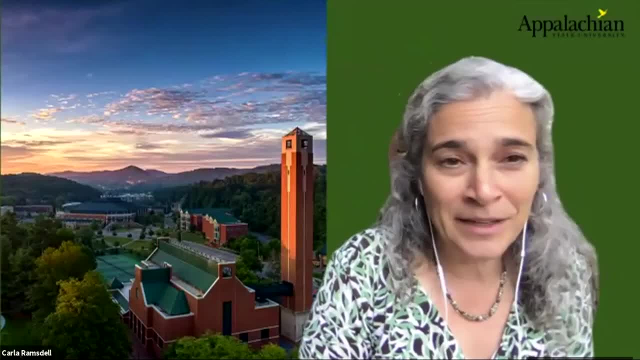 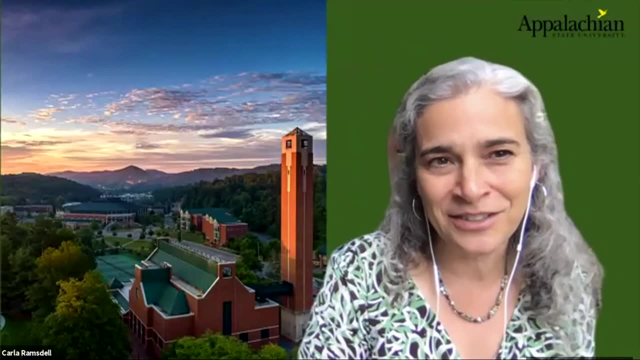 I would never talk anyone out of it. It's a. it's a great hobby. It is really fun to show up at some event and and whip it out. But I don't think it's gonna move the needle, obviously in the United States or in a you know. 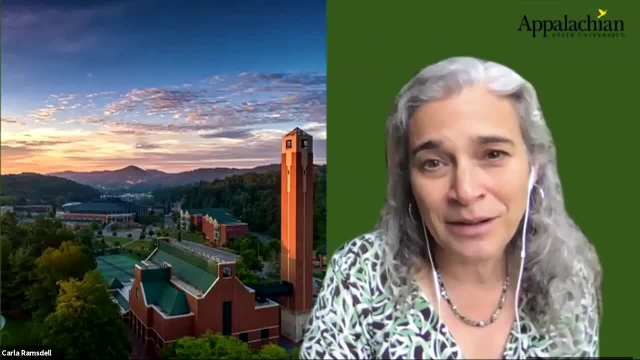 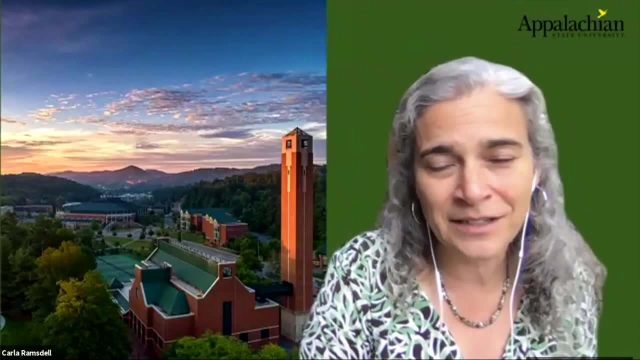 An industrialized country in our energy use. However, when we look at some other countries who are, you know, really struggling with cooking fuel, Deforesting to get the fuel they need, spending money They would otherwise spend on food, just to spend on the fuel to cook the food. 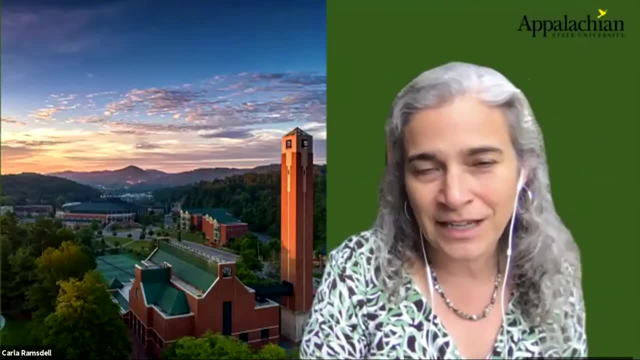 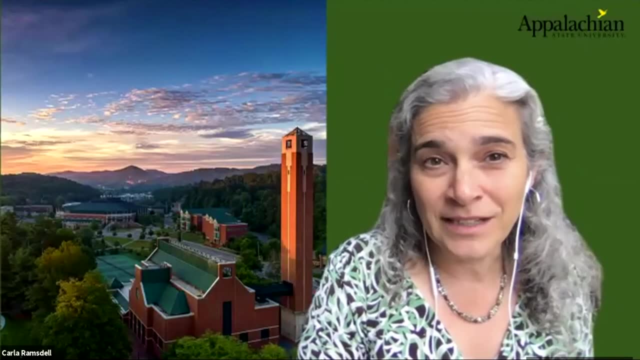 It's just enormous opportunity because typically have really good solar radiance in these locations And so you know, although they're limited a lot of resources, they're not limited in Sun. so I know both son of a In the box oven and go son the evacuated tube. 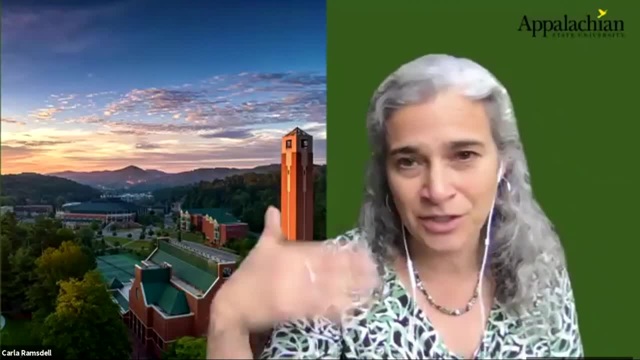 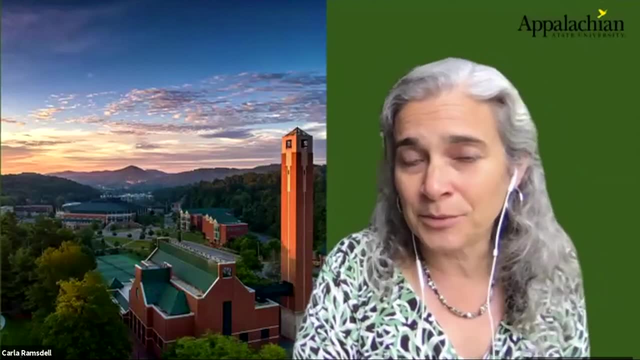 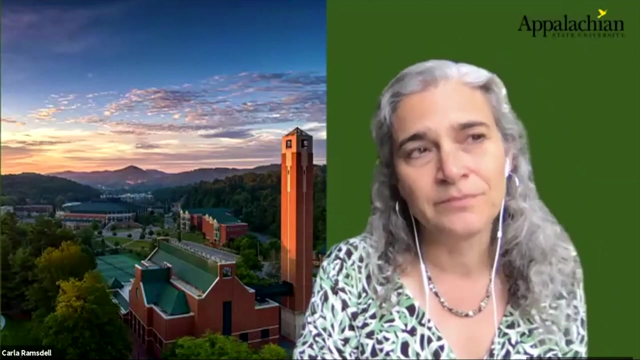 You know, for every purchase you make part of the proceeds go to purchase ovens and in other countries. So I've worked with a student on, You know, and that kind of deployment, especially for water pasteurization, You know to try to think how we can use these to make sure you have safe drinking water And so 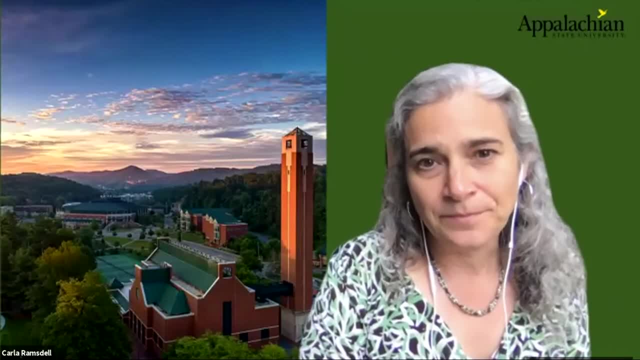 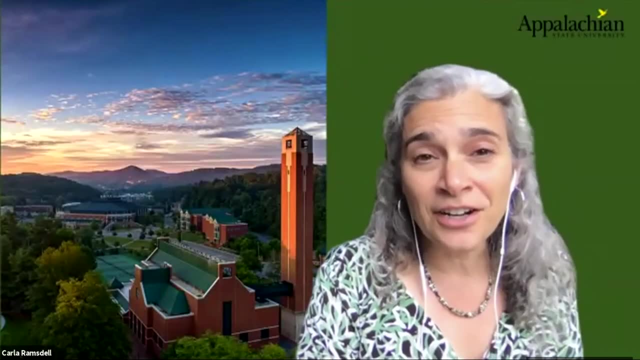 Yeah, pretty exciting opportunities there. Carla, can you scale them up? Are there bigger? Yeah, we're sure solar ovens There are. you know, the evacuated tube has struggled. So there is one example. I don't think I have a picture readily available. 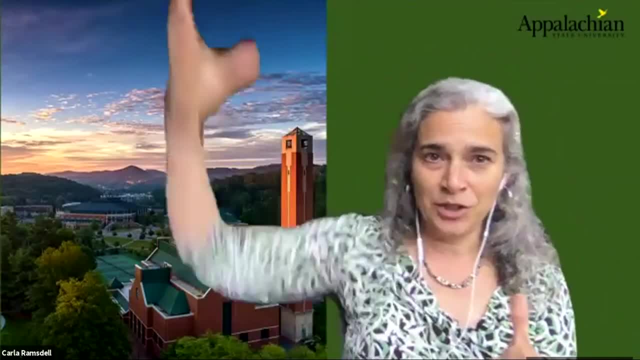 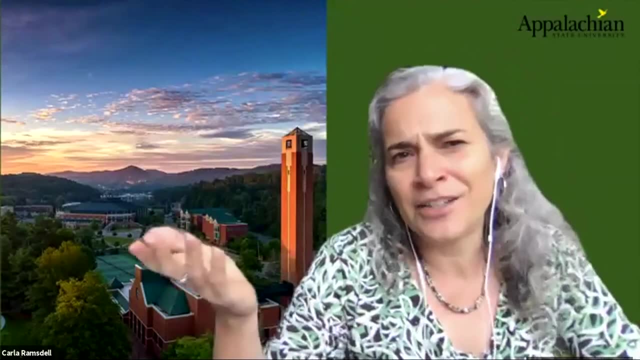 But basically it's a. it's a big sort of curved arched Reflector and there's maybe five evacuated tube stacked in there. So, like Jose Andres has done this thing on the White House, the greens of the White House once, where he was cooking on those. 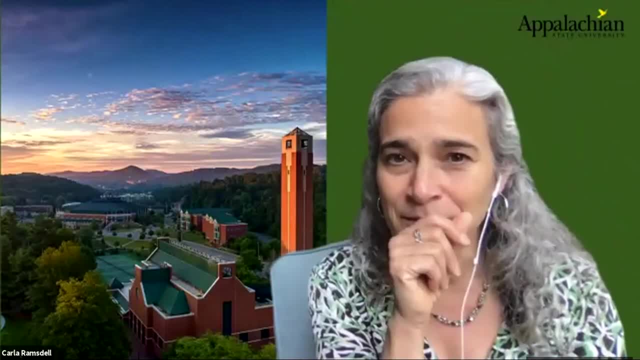 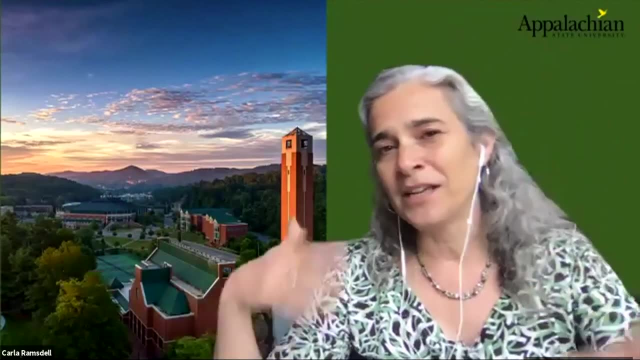 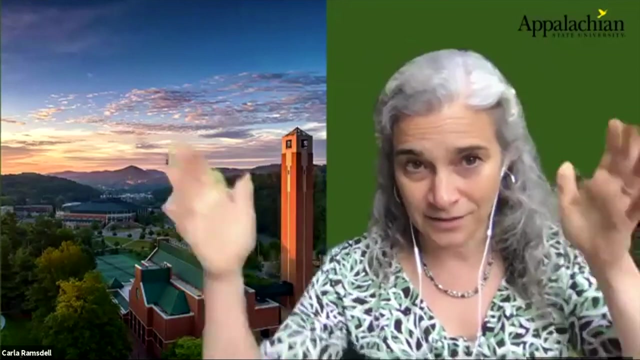 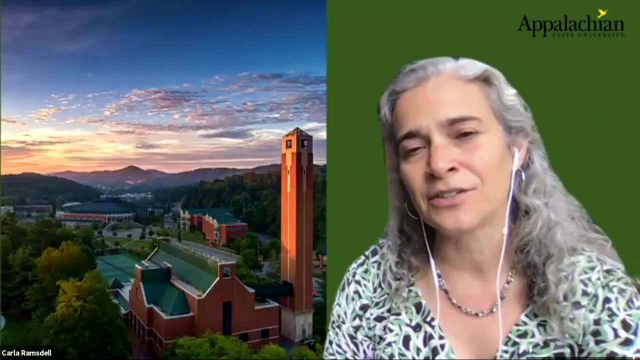 out there, But the box oven there is that that company actually has made a Trailer size big where you could actually have it in a community where they could be baking bread. you know something that's really useful And I'm not sure how you get into that thing, But I've seen it, like you know. maybe I want to say like 10 times bigger than that one. Right, It's really large with those same reflectors And so you can do something at a at a bigger scale. 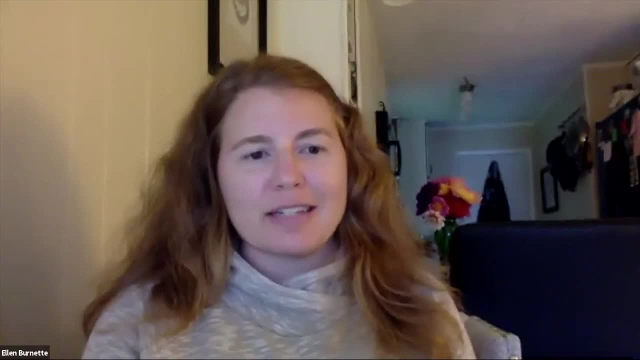 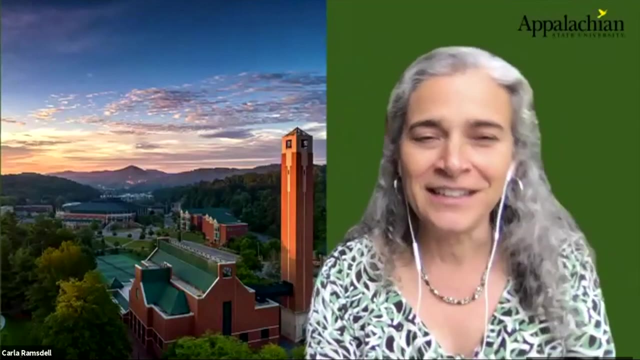 How did you get into solar cooking? Where did the interest for this gets bird? Good question. So I mean, I just think it was. It was a natural step when my backgrounds and energy and then little by little I started kind of get into this cooking thing. It was apologetically at first, because I'm 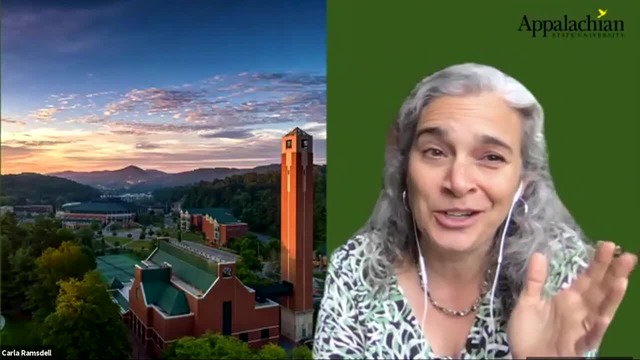 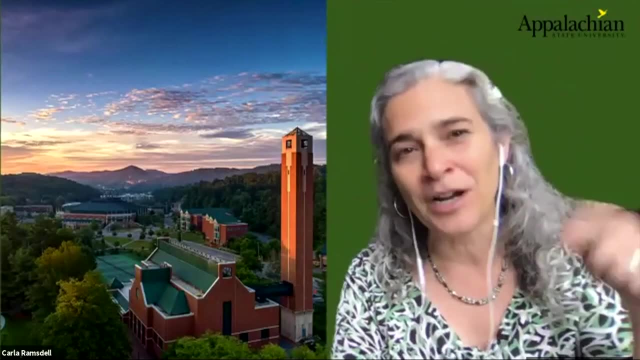 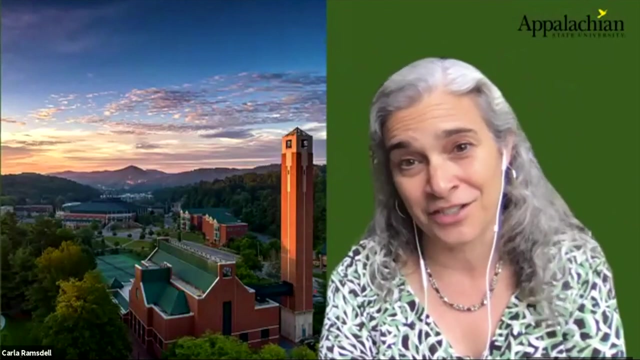 Really environmental steward and I thought, well, no, I really shouldn't be doing cooking, I should be doing renewable energy. but But just students love this cooking stuff, and but then, the more I researched cooking, It's an incredibly underrepresented energy source, especially in our energy efficient discussions. 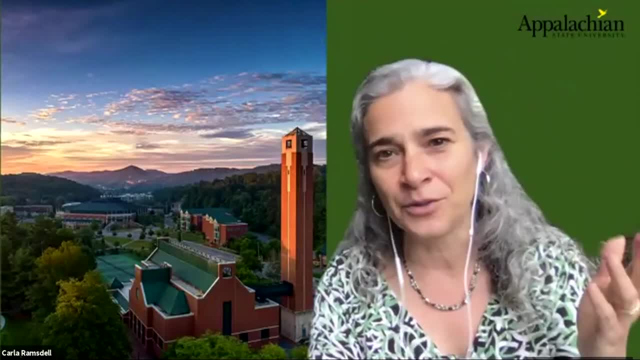 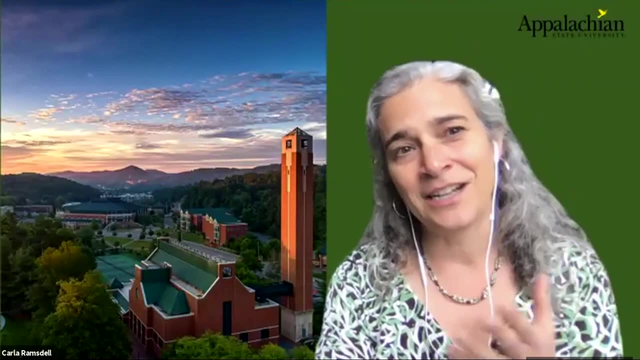 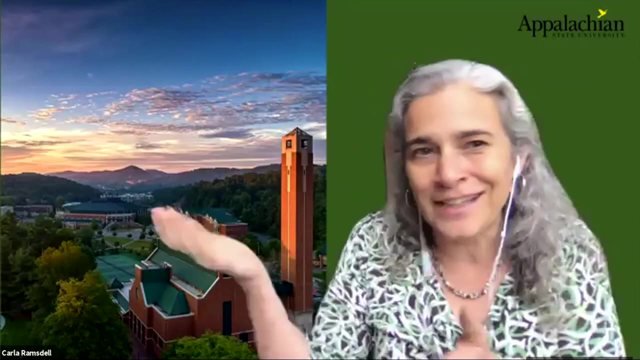 You know we talked about electricity and transportation, energy and heating, And you know a third of our greenhouse gases at least come from our food system, So you know. so then I just got really excited about this opportunity to, to Improve literacy around this energy source. And then, if you're like doing energy efficient cooking, solar ovens are just such a natural. 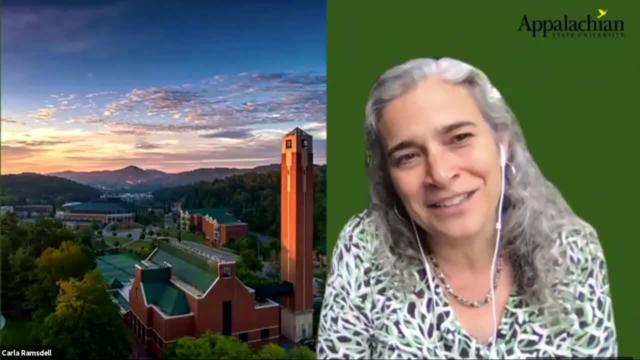 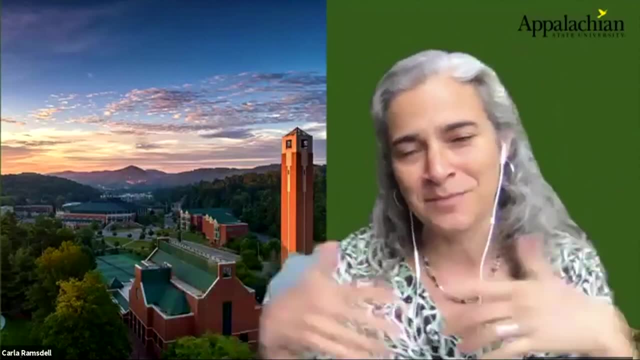 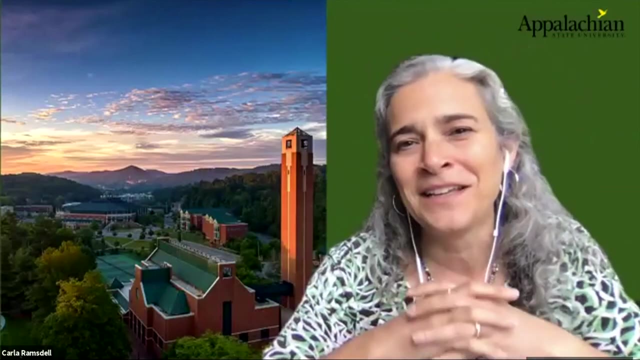 Step And there were, you know, so many options out there so that that whole collection of ovens has really taken probably eight years to gather. and every time something new comes out I try to find a great oven So we can experiment with it. And I've looked at heating curve comparisons between them. I'm a huge fan of the evacuated to, but it is fragile, you know that would be the. It's space limited and it's fragile. So I've definitely busted those tubes and I mean they're, they're great They. they provide replacement tubes pretty reasonably. so $20- $30 to get a new tube is not not so bad once you have the oven. 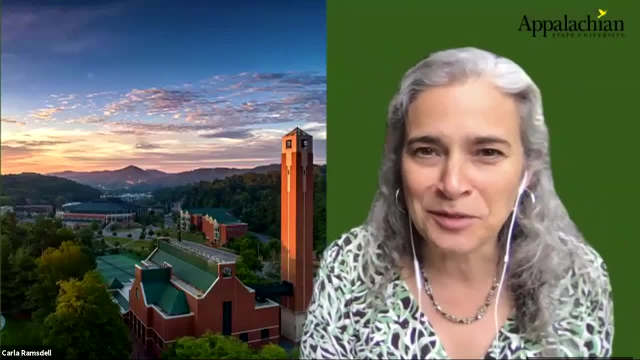 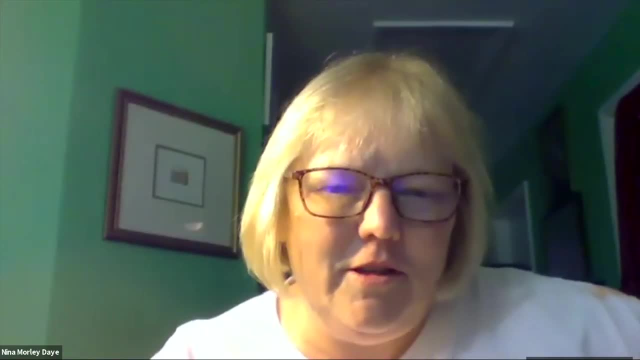 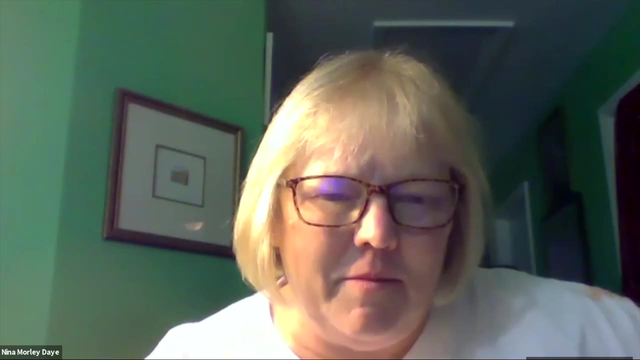 Yeah, an oven without a plug. this, It's a beautiful thing. Other, you mentioned That you've done some other work with this with energy and food. What are some other things you've done to reduce the amount, besides being differently on the food chain? 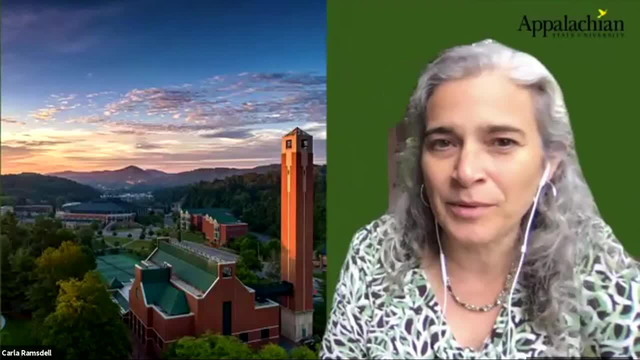 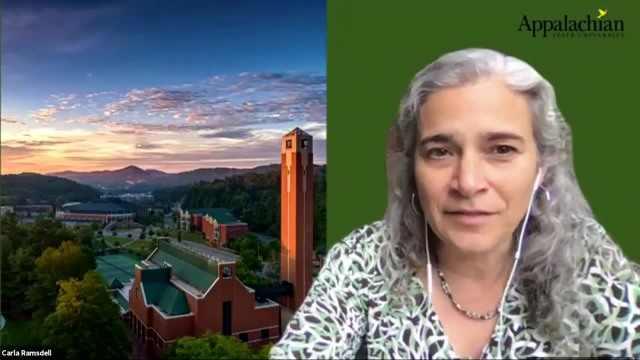 Right. So the food chain is definitely our biggest impact. if we get to eat more plant proteins, That's really where our biggest impact comes. my latest research is on skillet material. So we took- if I can, I share my screen. So we took- if I can, I share my screen. 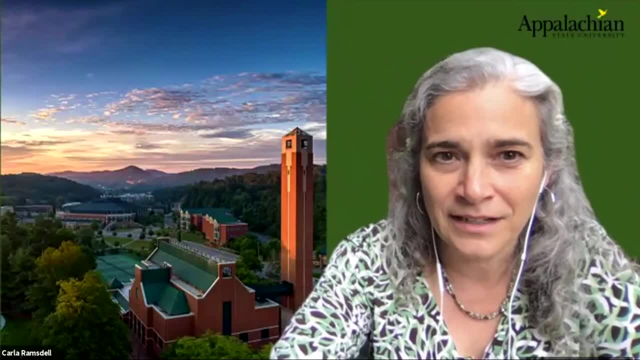 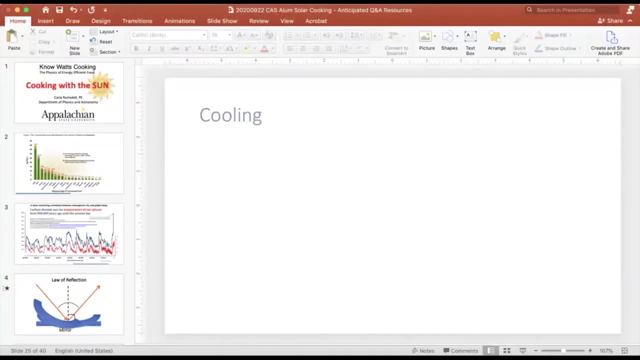 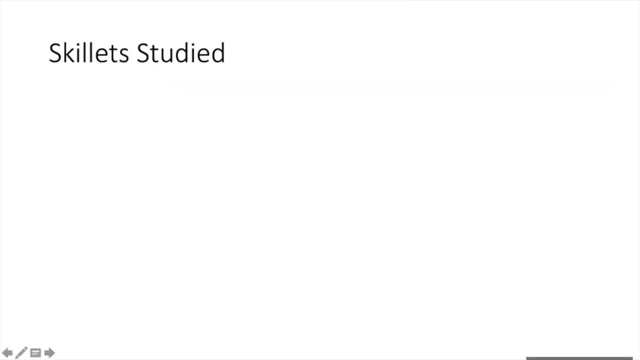 So we took. if I can, I share my screen here. I'm going to hop over to this other PowerPoint I have up here. So we tested eight different skillets. Let me see if I can get to that right here, Just for fun. So you go to a, you go to a skillet section of a of a. you know a store, a kitchen store, and the skillet options are completely daunting. There's so many different things. There's always something new. 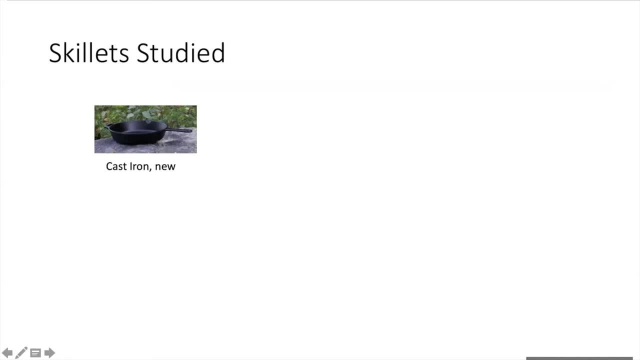 This new ceramic skillet thing now is all the rage, and so You know. so I think this, really this research, came about because, as I started getting into this, I talked to people who are really engaged in cooking and I'd say, what's your favorite skillet? and over and over again I'd hear a cast iron skillet. 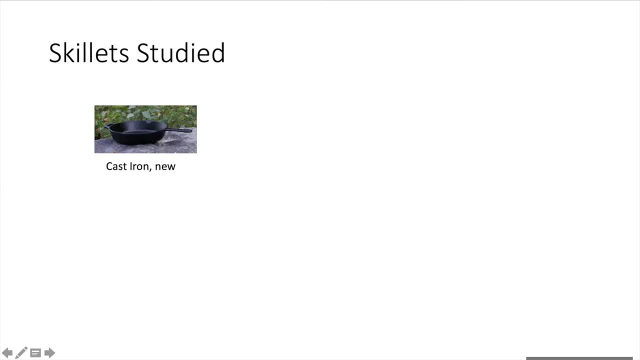 I was not raised in like the Deep South, like cast irons were not part of my my cooking repertoire, but it was. it was just incredible how often people who were chefs and really into food would choose a cast iron skillet- cast iron skillet. So I go to the thermodynamic property tables and start looking up. There's. 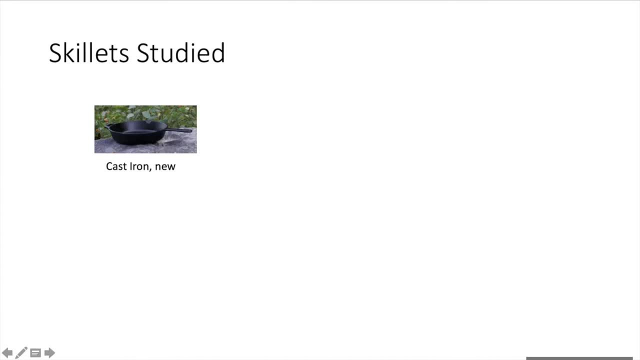 nothing about cast iron that would lead me to believe it would be a rock star. So I've just felt like you know. the other thing I thought was interesting is people would say, well, I've tried cast iron before, but everything I cook on it always burns right. So that piqued my interest. 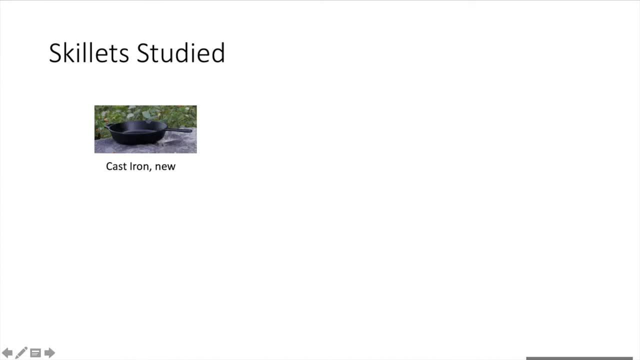 too, because if everything's burning, it means that whatever you're used to setting the burner at with your other cookware is too much for a cast iron. But why is it? the cast iron is moving that energy more efficiently Because actually its conductivity is lower than almost any other. 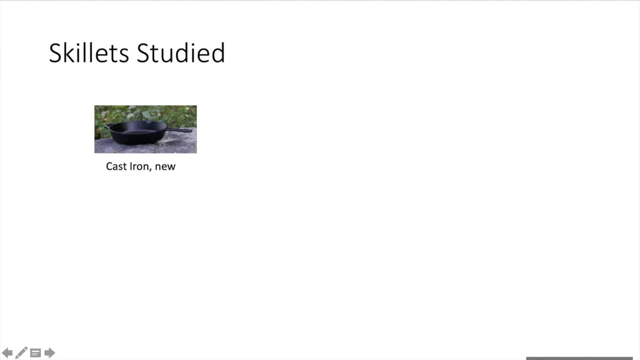 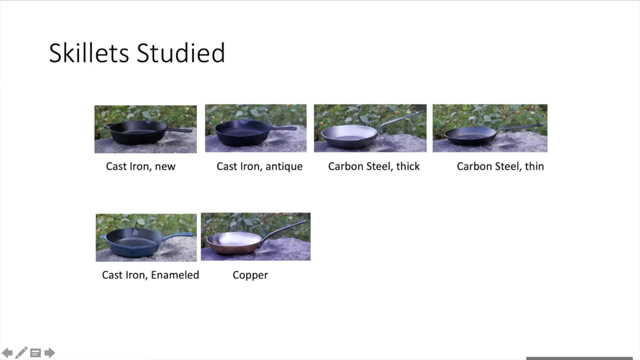 material we deal with. So I had to be able to see heat. So that's really where this infrared camera came in, Super handy. We tested. so we tested a new and an antique cast iron, two different carbon steels, thick and thin, an enameled cast iron, a solid copper pan. So this was our most expensive. 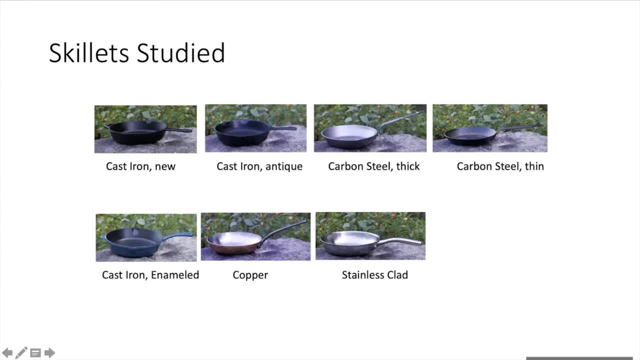 pan- $200.. And then the stainless steel, all clad and anodized aluminum pan. So this was, and these look. this is the arrangement of where these pictures will show up, So let's just watch for a second. These are the infrared images of these as they heat up, And I'll go back and forth. 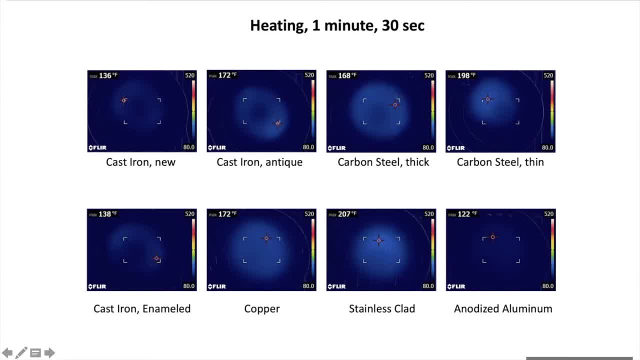 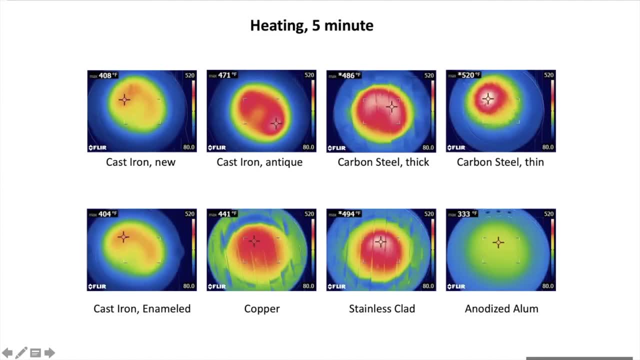 but this is like at the one minute mark and then one and a half minutes and two minutes and two and a half and three and three and a half and four and four and a half and five. So you know, and you can look at this over and over, because I've looked at it for about I don't even know. 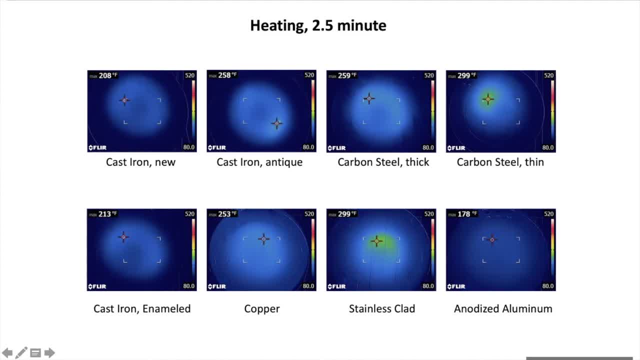 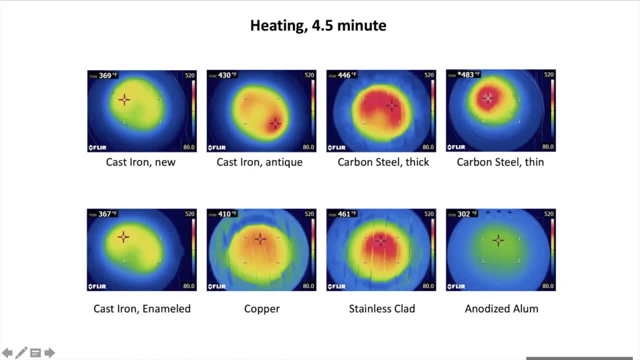 how many hours these images, but we see some really interesting things happen. for one, the cast iron, you know, even though it's a really poor conductor, you know that's not a bad thing in a skillet, because in a skillet what we're doing is we're cooking in the bottom of the pan. so I don't care, it can make it. 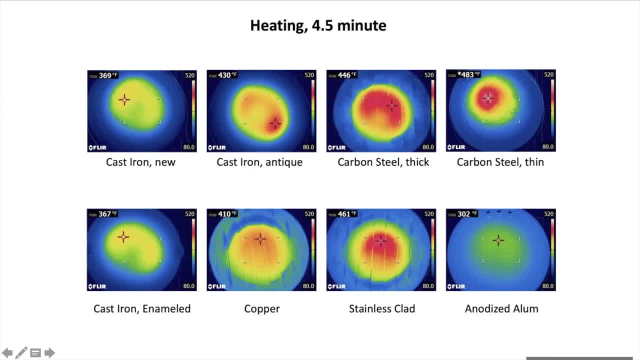 through the thickness of the pan. what happens when it's not a good conductor is that it tends to keep the thermal energy down at the bottom where I delivered it. so if you compare, for example, to this anodized aluminum, that's a really good conductor. you see that my temperature at the 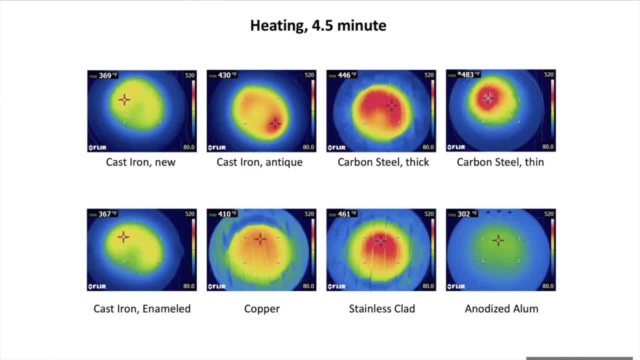 bottom with the same amount of heat input is much cooler, even though it's a better conductor, and that's because you notice the edge temperature here right. so this edge here is is hotter than my cast iron, but I don't care what the edge temperature of my skillet is. I'm never cooking. 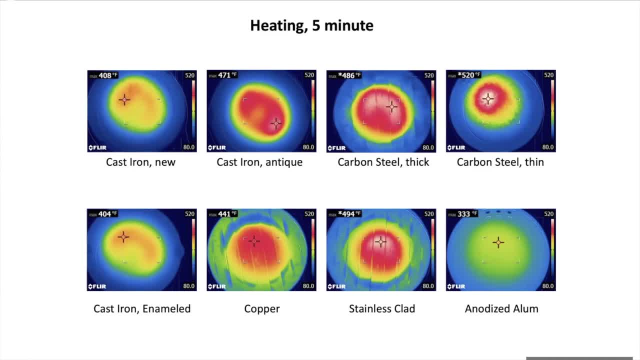 on the edge of a skillet, a pan, a pot- a totally different scenario, right. but for a skillet we really want to keep the thermal energy at the bottom where the heat is being supplied. so I think these images helped us to see you know how effective those, the carbon steel also. you see these really hot temperatures down there at the bottom because 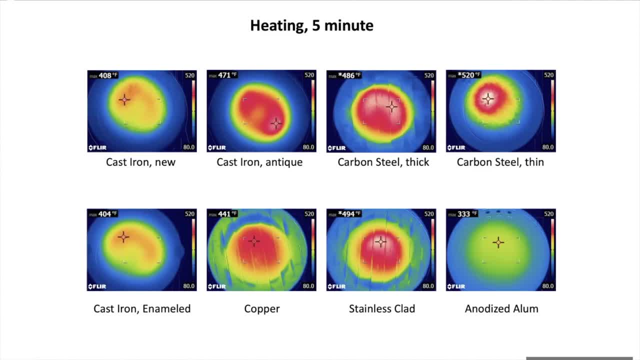 it's also a poor conductor, so so that was kind of fun. the other thing we realized that we're working on now as sort of phase b to the study is the, the radiant effect. so cast iron also is a really good radiator and, like the copper pan, is terrible. 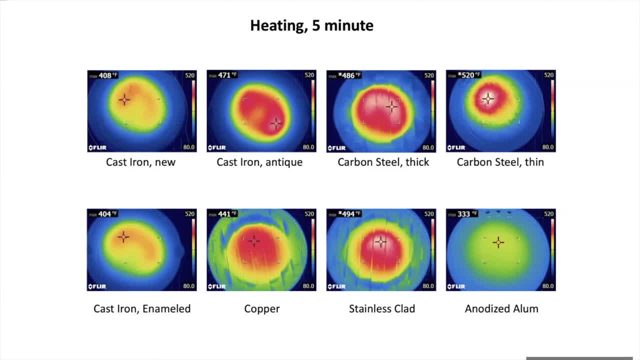 it's shiny surface, it's a great reflector, it's a terrible emitter. so so food that's in direct contact with those shiny surfaces can cook by conduction. but if you put, like, a pile of potatoes, and some of them are not in direct contact with the, with the pan, if it's a shiny pan, 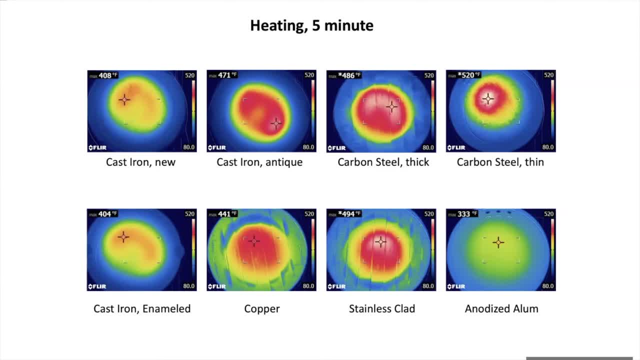 the it can't reach it. it's not an emitter, but a cast iron can cook those potatoes even through an air gap, because it's a effective radiator. so what we're trying to do now is quantify that and use this infrared to look at the radiation and see if it's a good radiator and if it's not. 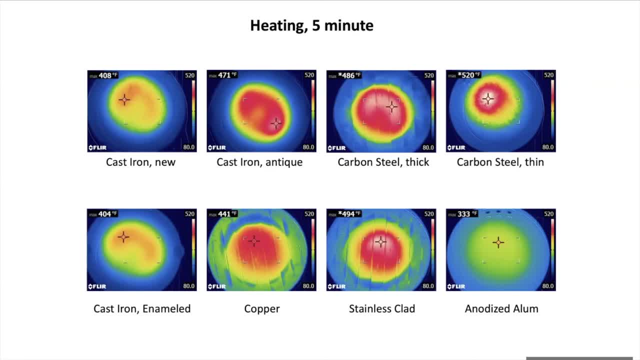 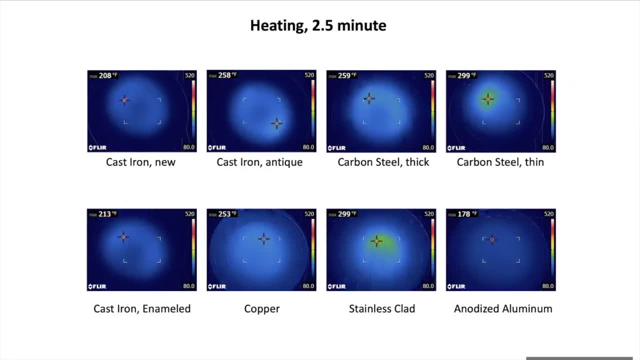 the radiant differences in these different surfaces. we can watch them cool down too. you want to watch them cool down, it's just so much fun. so anyway, it's a good question. and so we found out. i mean, whether we looked at embodied energy or longevity or toxicity, or, you know, cooking energy, the cast. 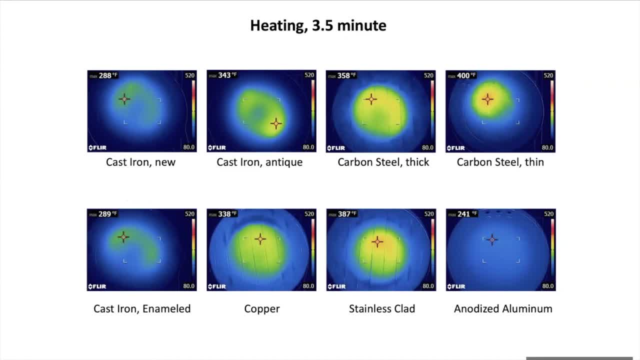 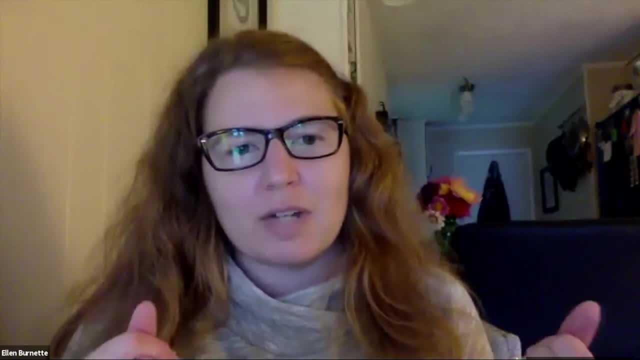 iron really just rocked it. it was, yeah, by far the best. that was really cool. i was going to ask you. i noticed you were using a cast iron and you were using a cast iron and you were using a silicone hot mitts. are there certain things you're doing, solar, that tend to be safer to? 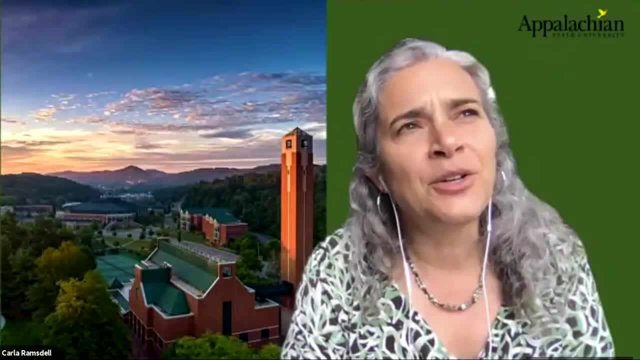 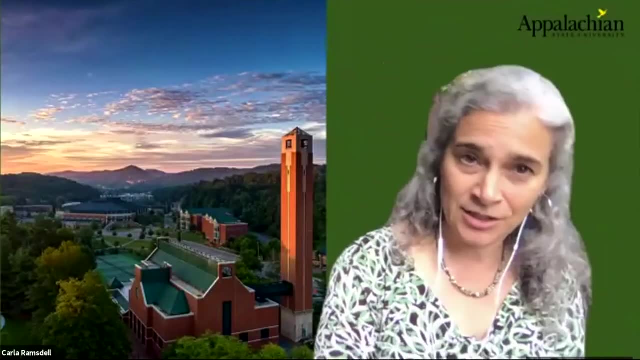 handle things or utensils that are best? that's a good question. um, for the most part, what's coming out of a solar oven is no different than your house. i love the silicon stuff, uh, because it's all dishwashable too, you know. so, again, if we're looking at a sustainable kitchen, we want to make. 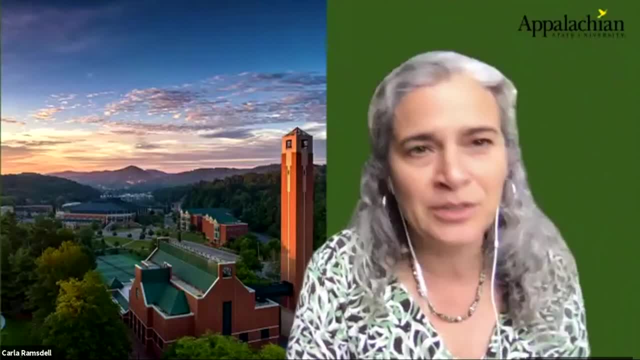 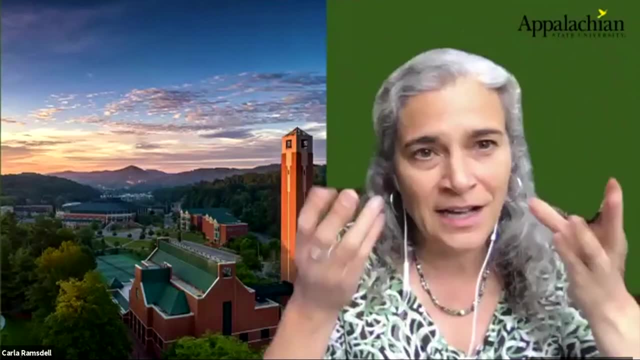 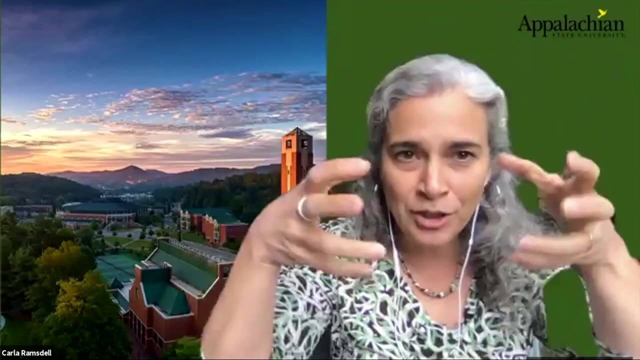 sure we're minimizing having to purchase and repurchase, and repurchase, you know, and so, um, you buy one set of good silicone- that's the, the flexible stuff, uh, hot pads, or or even the you know hot pads that you put pots on, or the mitts, and, uh, you know like you can grab a turkey with those and then just walk over to the sink and 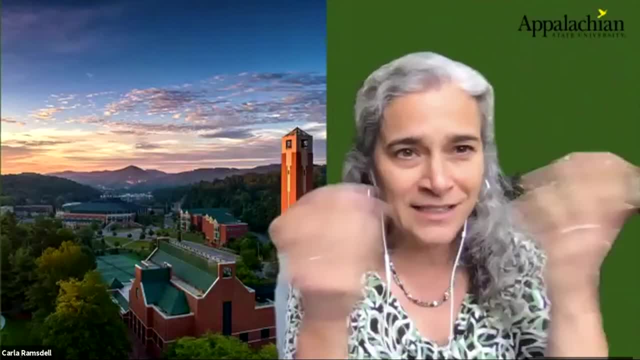 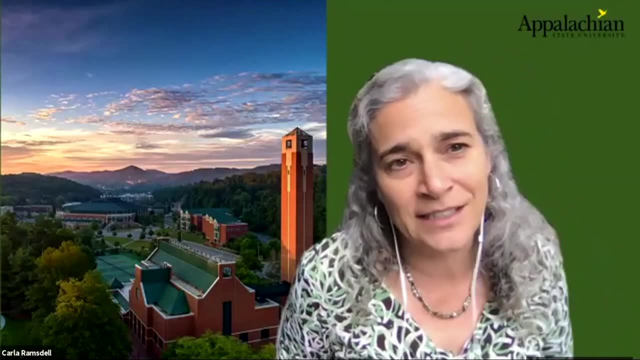 put hand soap on them and just kind of wash them while they're on their hands and they're good to go, and i do just i pop them in the um, in the dishwasher, to the hot pads, and they come really clean. so you know, it's one of those things you just don't have to have to purchase often once. 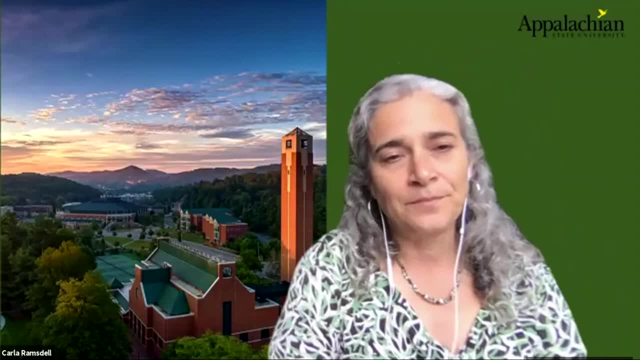 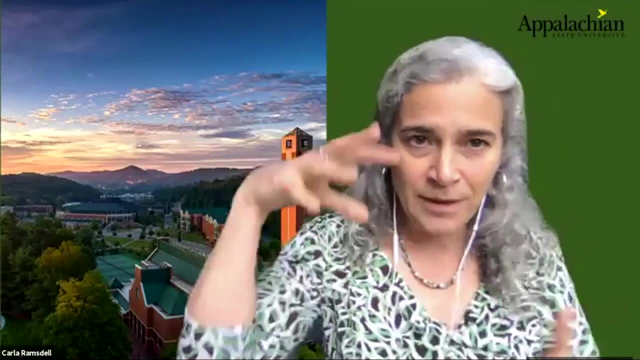 you got them. they last a long time and you're doing you know uh cast iron stuff, like in the oven sourdough break baking and you know you can make these uh sort of contained. you can cook sourdough in a cast iron vessel because it helps to contain. 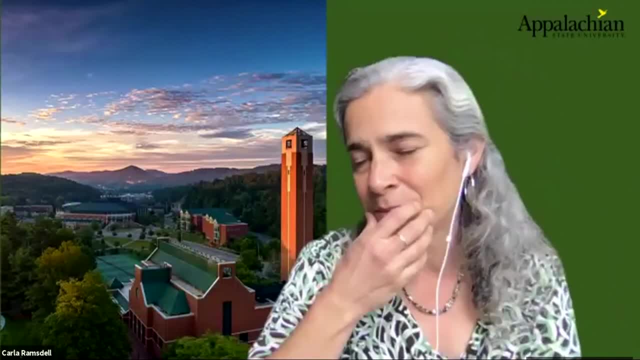 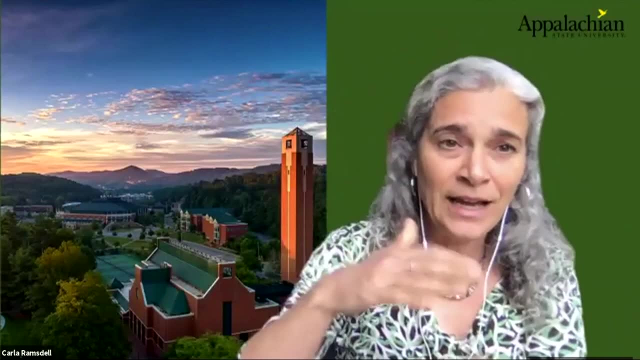 the steam, because our ovens aren't steam injected like a commercial oven would be. those are really it's like 500 degrees. so you want to be careful that when you're putting it on the counter after that, that you have something that's a really good insulator, and silicone is really good for that. 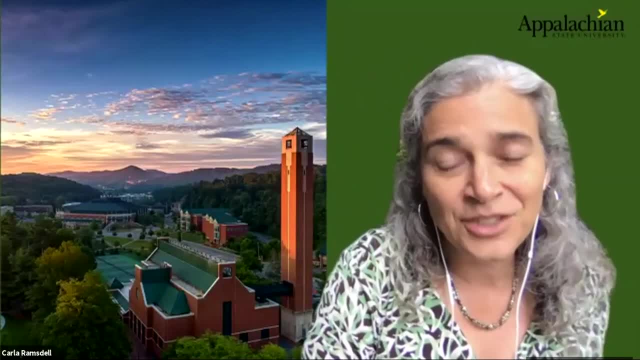 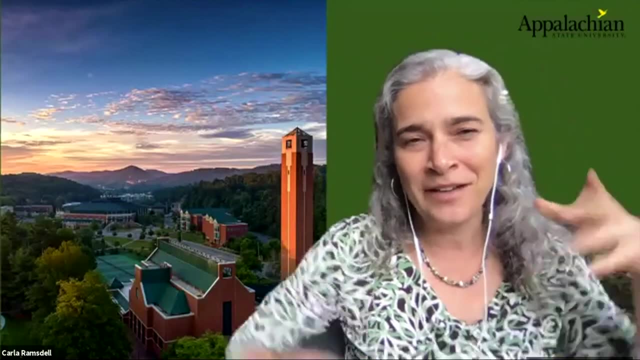 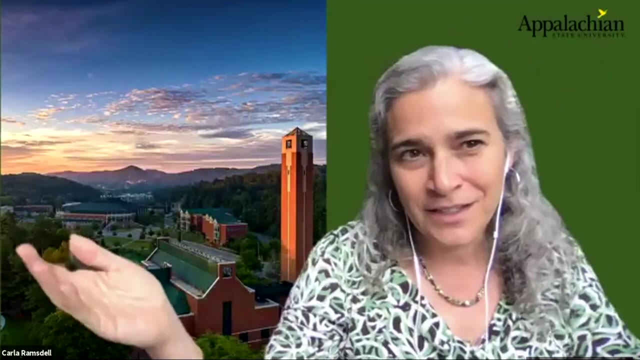 so a cast iron pot's not a great idea, right? because going on this whole radiator concept, if you have this big black external tall surface and you heat it up, well, it's just throwing energy out to the room. so when you're talking about pots like, um, you know, for pasta or whatever you 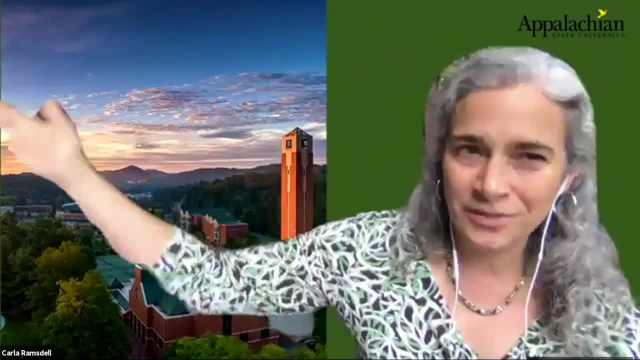 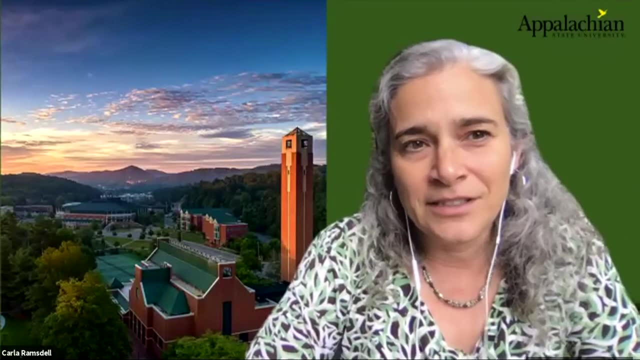 actually want a reflective surface because you want something that's not going to throw that energy out, but for a skillet when your food's above it, you want it to be a good energy source. reason to think that a process could be really difficult when you're cooking. but a기도 it's. 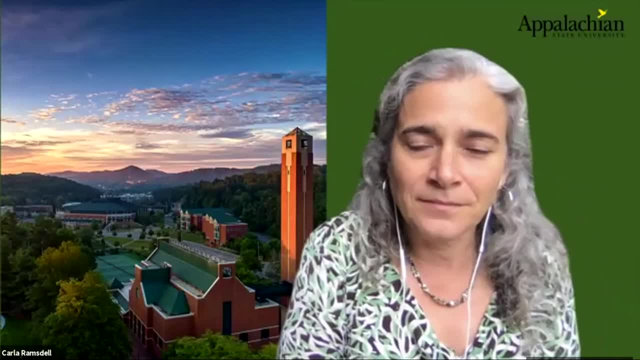 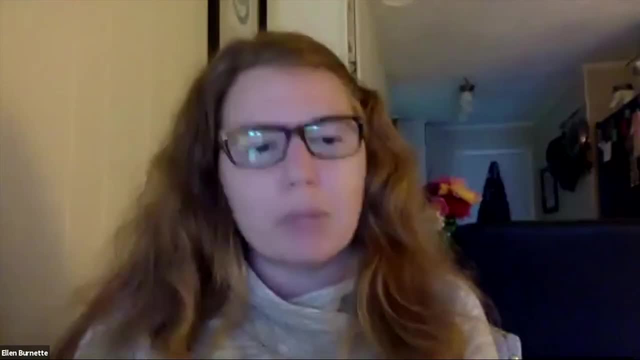 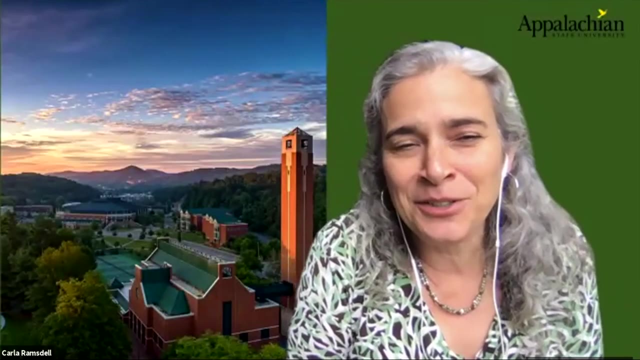 going to be a good radiant surface. so different considerations for different purposes. any other questions? so for a pot, is a ceramic lined cast iron better then? oh, good question. i have not done that. that's really actually study. i want to do is: does the color of your late crusade dictate how good of aOK? 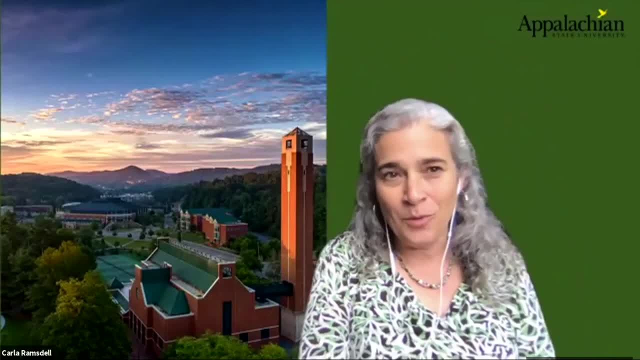 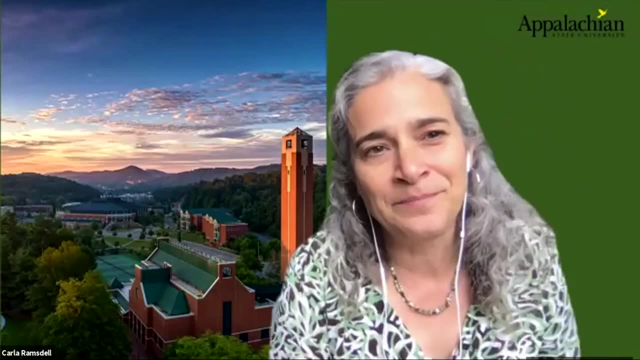 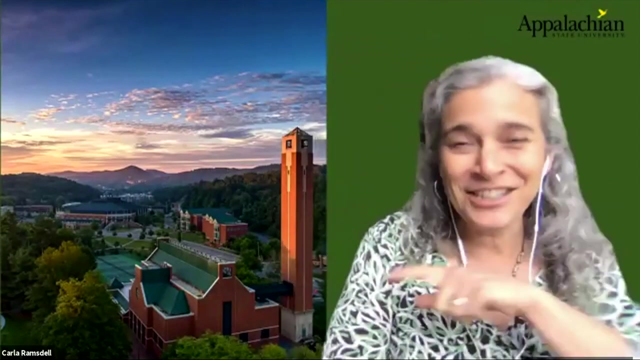 emitter. it is- and my gut says probably yes- that a white Le Creuset is probably more efficient than a black external Le Creuset because of this, you know, emission thing. so I don't know the answer to that. but I have actually reached out to the art department so I 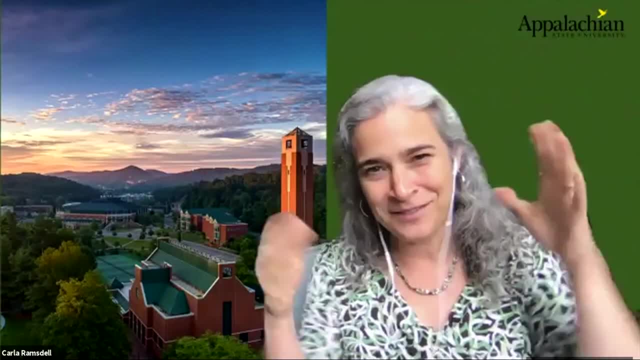 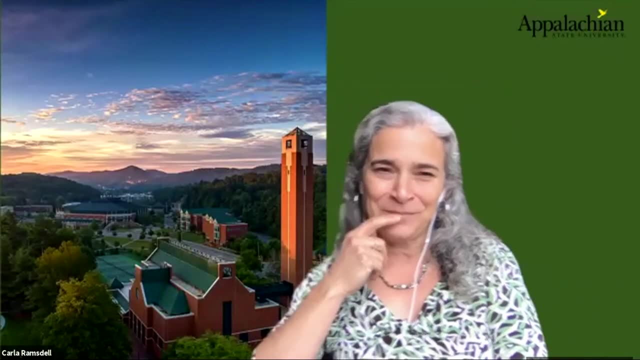 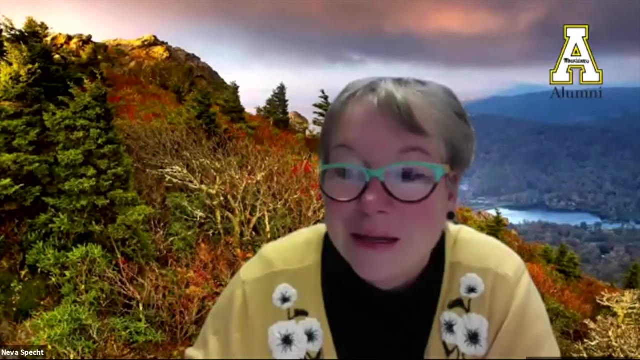 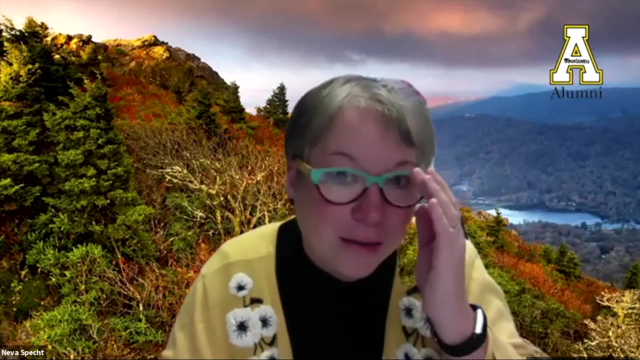 thought that'd be really cool collaboration if they could make me a bunch of glazes of different, so anyway, so stay tuned. we might be doing that research here in the future. anybody else? well, Carla, I really appreciate you doing this. it was. I mean, I think being able to see all those different varieties of ovens is just 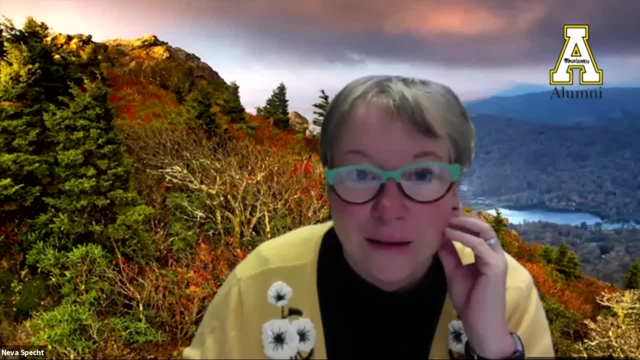 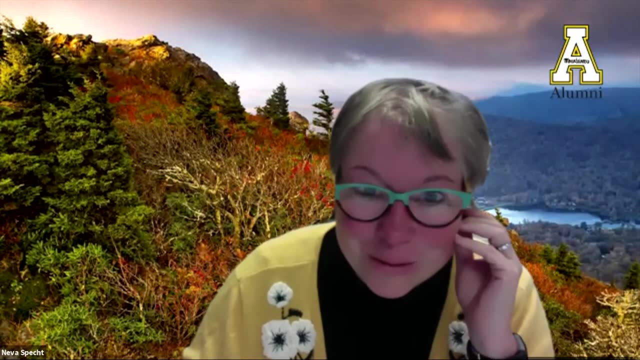 amazing. I I guess I like these things the best because I get to learn so much about what everybody's doing in their work. so thank you for those of you who may have joined us late. we'll be posting this out on our website, correct, Ellen? Ellen? 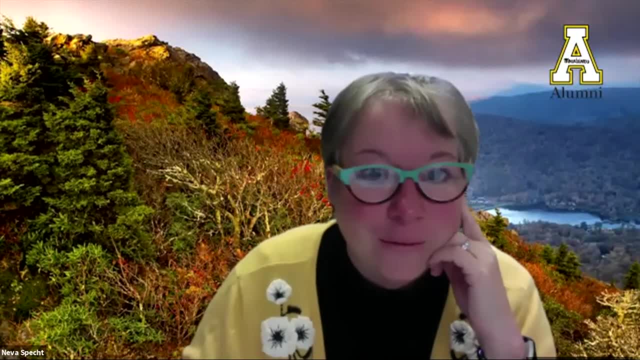 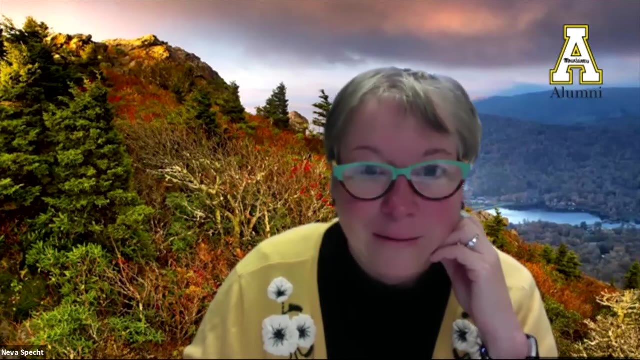 Ellen, Ellen, good, and we have three more coming up this fall and if somebody can help me with those dates, next one is October 6th, and that'll be with the biology department talking about the fall leaves and other plants, and then that's where I 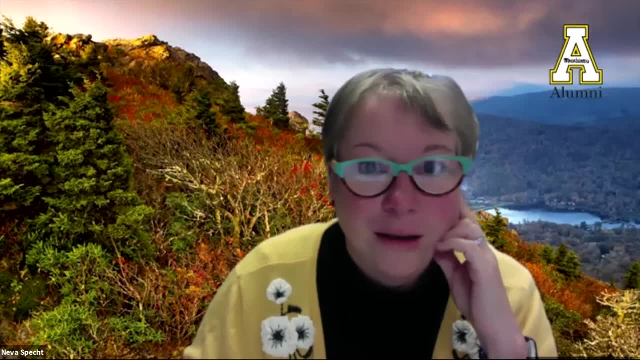 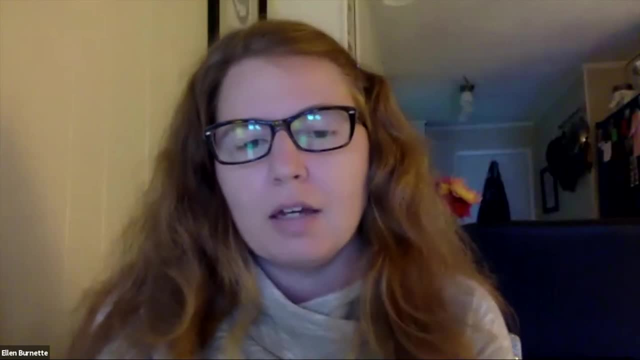 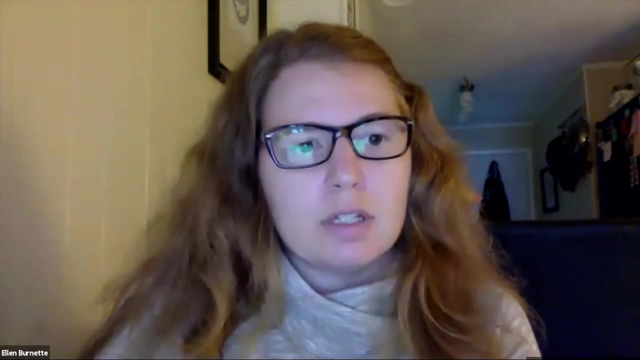 need some help. after that one October 20th, we'll have a we're partnering with career development to look at resume writing or interview techniques and then on November 17th- I do believe I'm gonna double check that- we'll be interacting with some other STEM related disciplines. 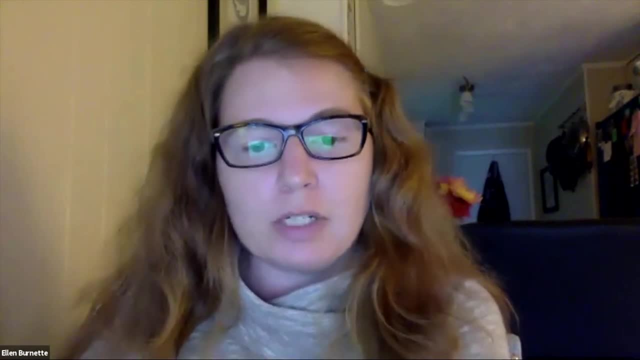 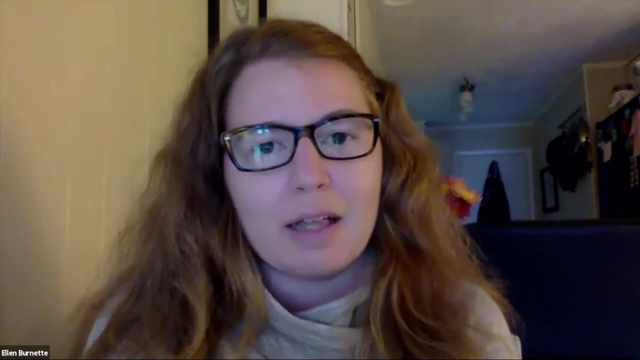 in the college for some information about outreach and some activities. and then I do know Carla wanted to plug another awesome event that's gonna be coming up in the college that is open to everybody. yeah, absolutely, thank you for the reminder. so I'm excited to get to know you and I'm excited to be able to. 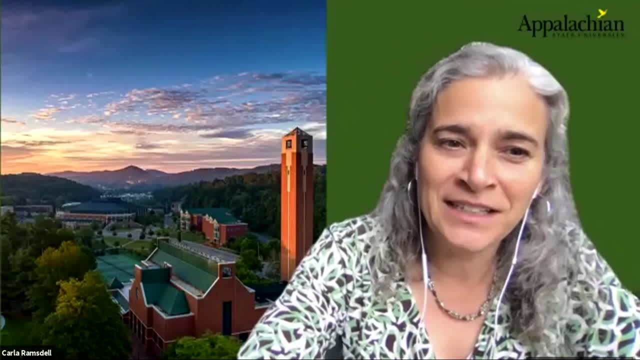 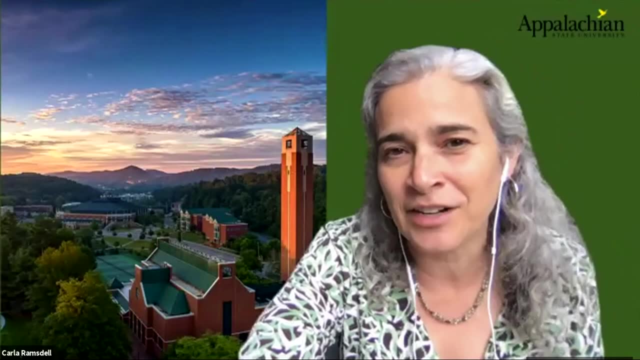 talk with you about some of the events that we have planned for this fall. on November the 12th, we will be hosting community feast, and so I'm just gonna give you a little snippet. I can change my workload of background. so the past three years we've held this event on campus called community feast, where we 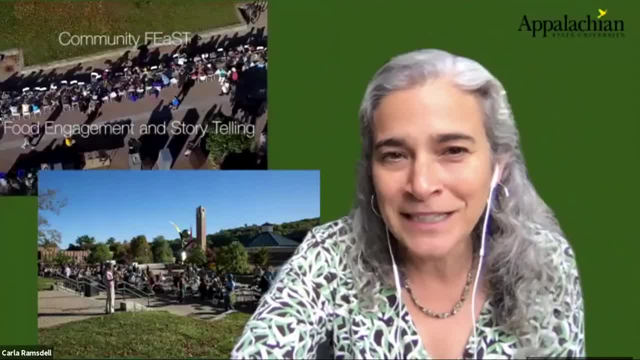 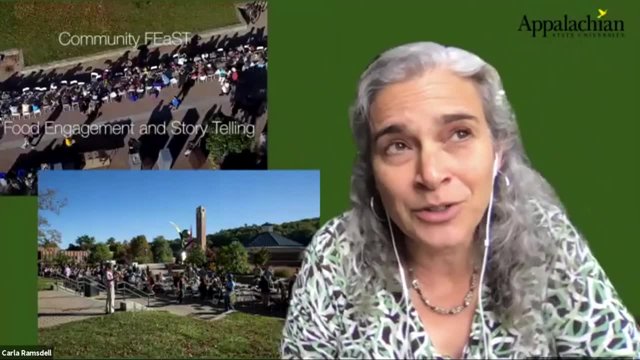 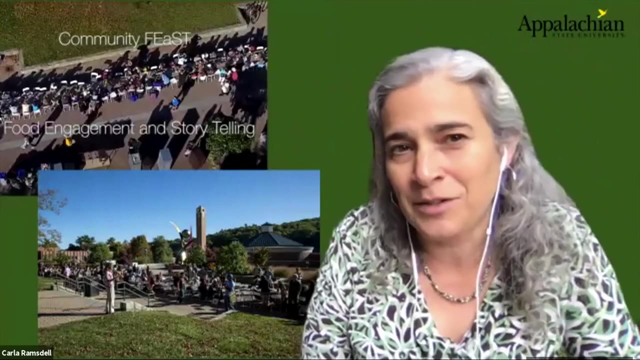 we set a 100 yard long table down the middle of campus and invited people to come join us for a meal, and so these are some pictures of the past events. it's really phenomenal. we invite anybody to come with two others. three goals: we try system by storytelling. We also try to reduce waste so people have to bring their own plates. 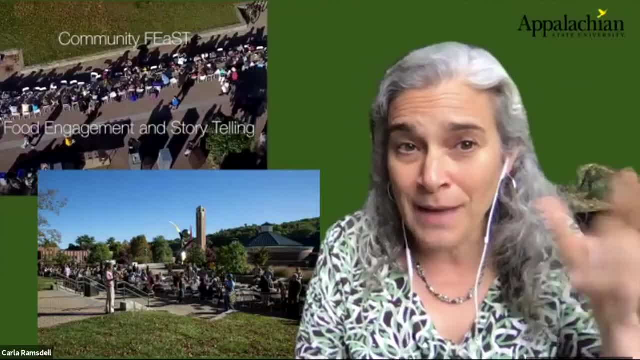 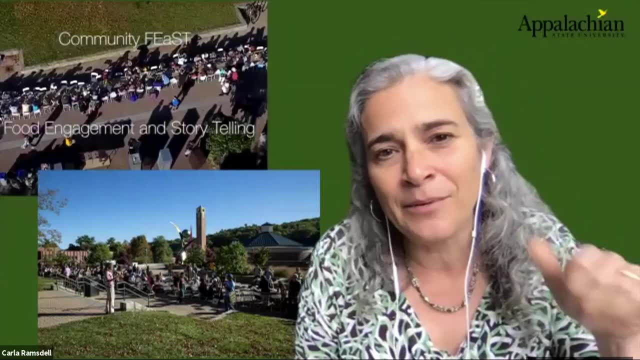 and water bottles and then also maximize local sourcing. so we've bought our food from the High Country Food Hub and it's a really simple meal: baked potato and apple pie. We have student groups come and provide the toppers. Obviously, we are not going to be gathering around a hundred. 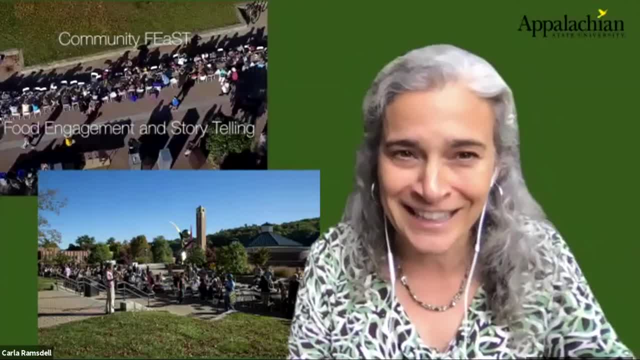 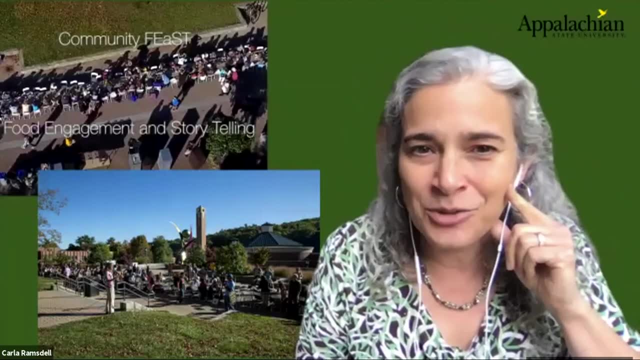 yard table in the middle of campus, although we would love to do that this year. so we're going to hold a virtual event instead. so it's on November 12th at 5: 30, and anybody can join us. We are actually dreaming big for this one figuring to try to take advantage of the